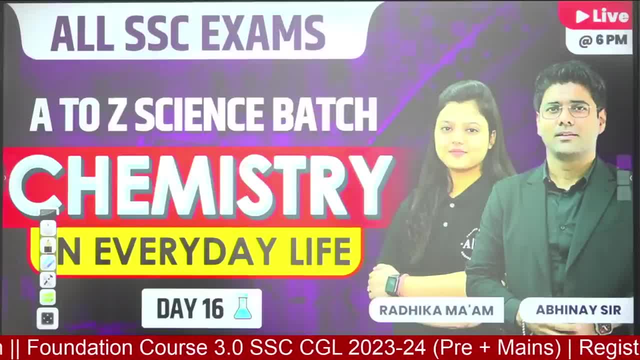 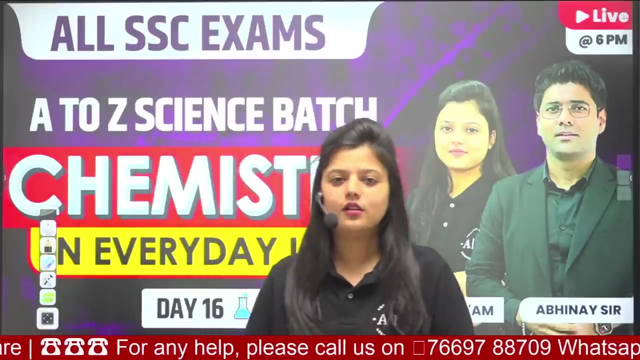 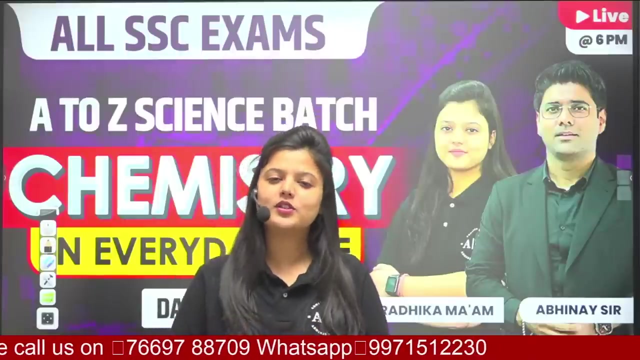 Thank you, Hello, and a very good evening to all. Welcome to SSC Abhinav Maths, and this is Radhika Gupta. Hope you all are good and healthy. Let's start today's session. How are you all Tell me quickly? 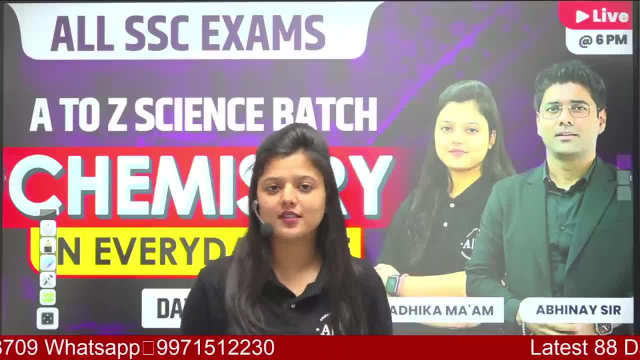 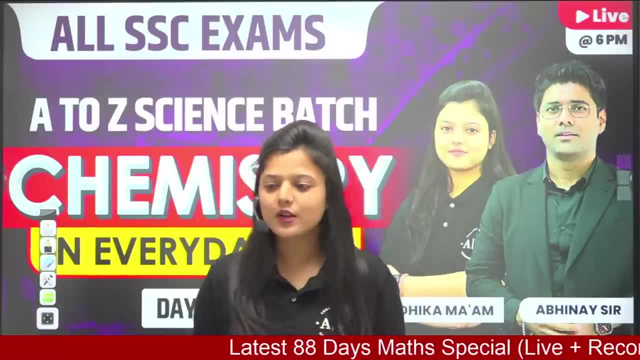 In today's session we are going to practice some of our questions so that we know where to start. How much water do you have and how is your preparation going on here? So I hope all of you are good. A very good evening to all. and with this we have studied a lot of organic compounds so far. 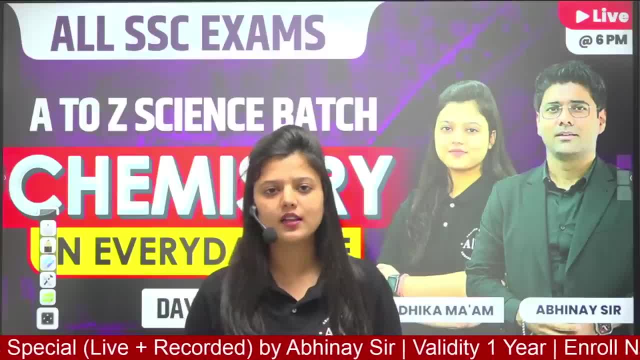 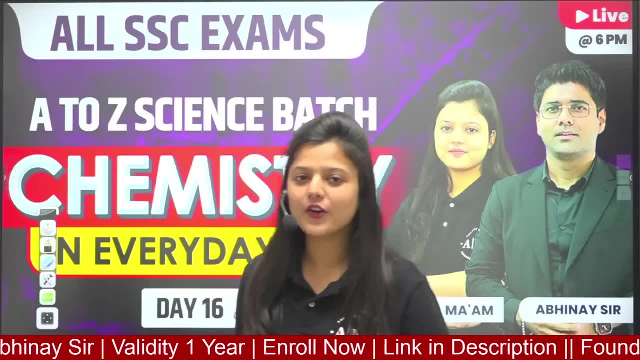 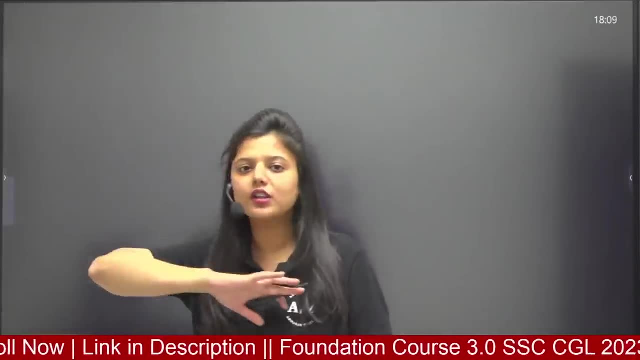 What is hydrocarbon? How are your different ring compounds or open chain compounds made here? So let's do the session and share it quickly and let's start some of our questions. and a little important topic: So far we have divided the complete organic compounds, divided their structures. 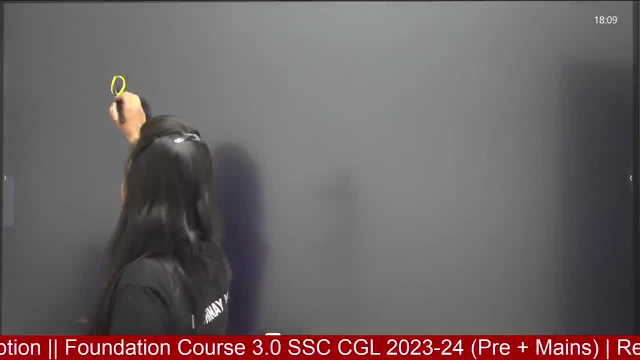 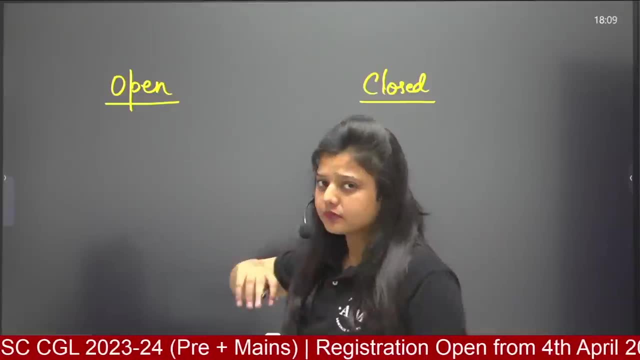 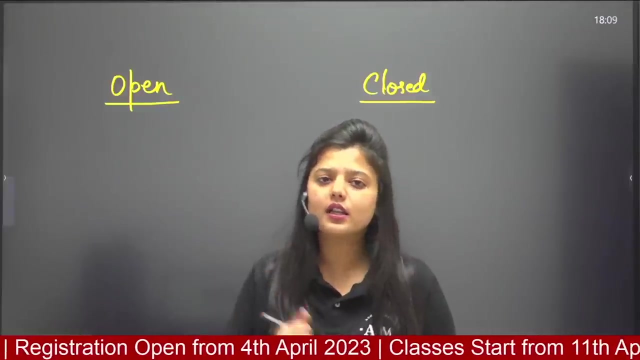 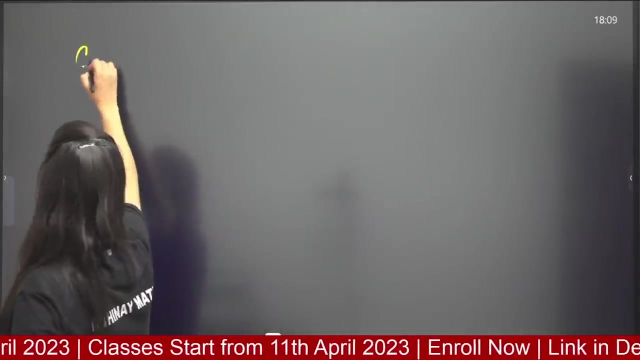 We have studied that on one hand, there were our open chain compounds. On the other hand, there were some of your closed chain compounds, which you also knew as your cyclic compounds After that. if we have understood these two compounds well then, one important thing is that all your different carbonic compounds have some chemical properties. 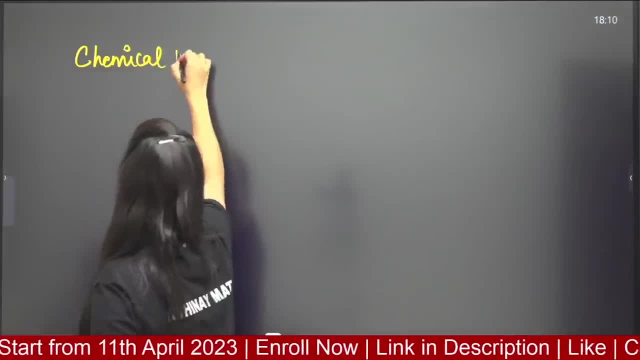 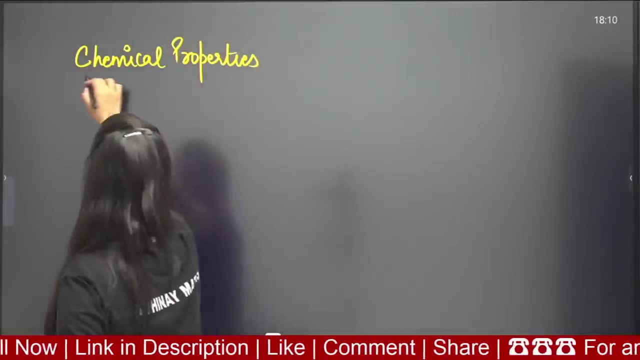 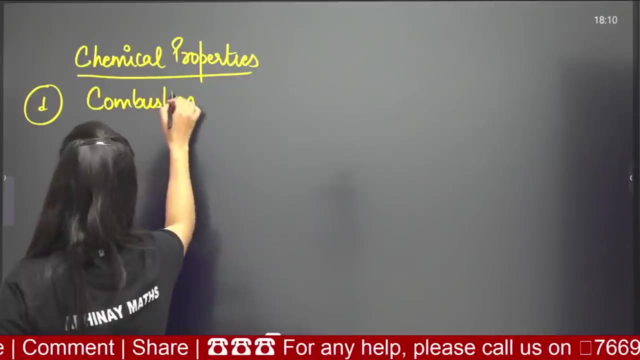 So first of all, let's talk about them today, And after that let's start our topic. The chemical properties of all your organic compounds will be here, In which the most important and the first property comes is combustion- Combustion. 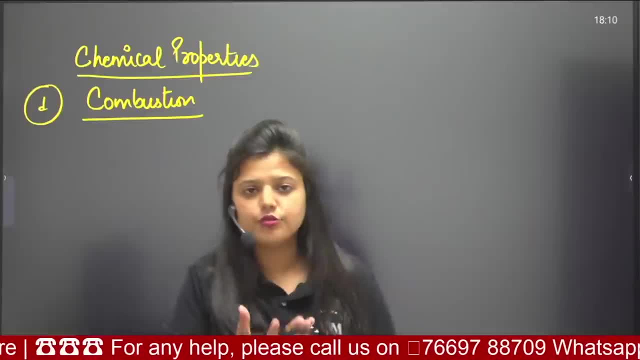 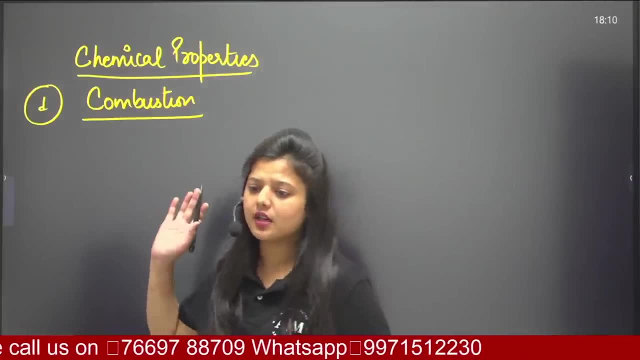 You saw that the process of the body. usually, if I am talking about any oxide, I usually talk about carbon dioxide only How is your carbon dioxide made? Everyone is getting audio and video clear here. The session is live. Everyone has audio and video properties. 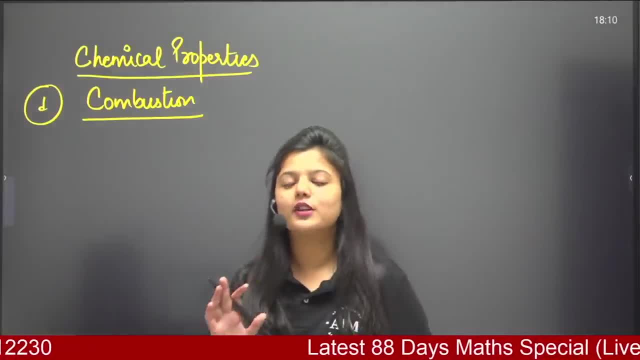 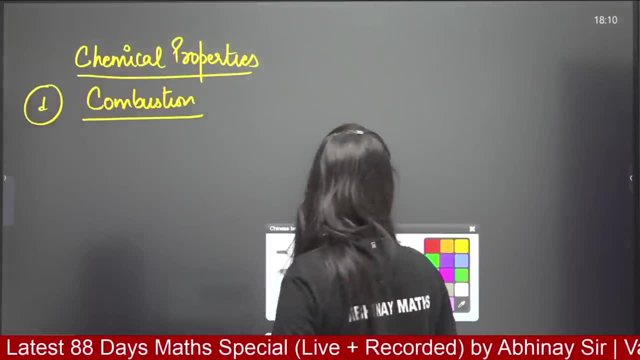 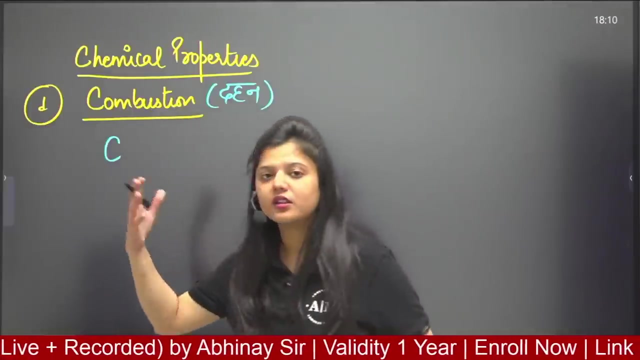 Once. you share the class with all your friends, so that this free session should reach every student And everyone's preparation should be done in a very wonderful way. So we are talking about the properties of the body. You said that the compounds that were made from carbon. we called them organic compounds. 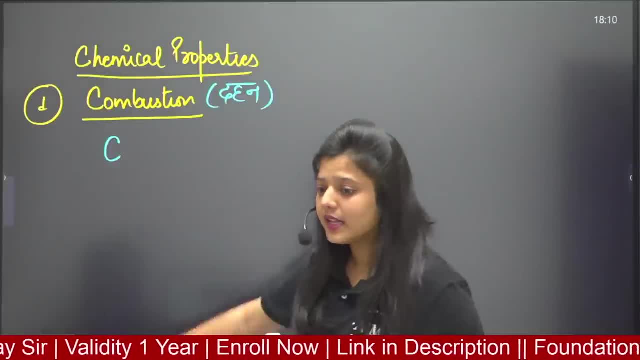 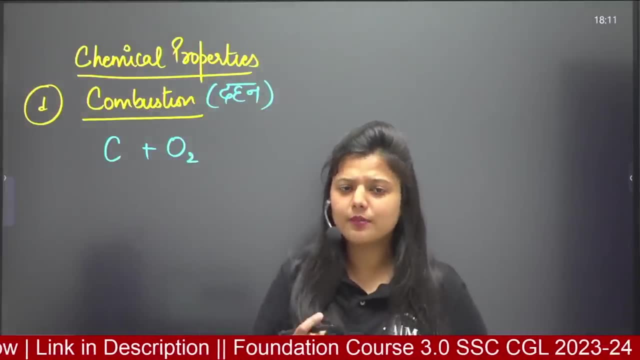 Carbon and hydrogen are coming, so we called them hydrocarbons. If I want to burn this carbon in the presence of oxygen, what should I do? I want to burn it with oxygen, So tell me what will be made. You said that it is simple. 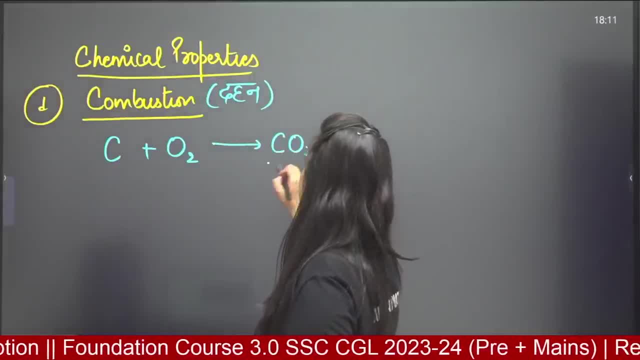 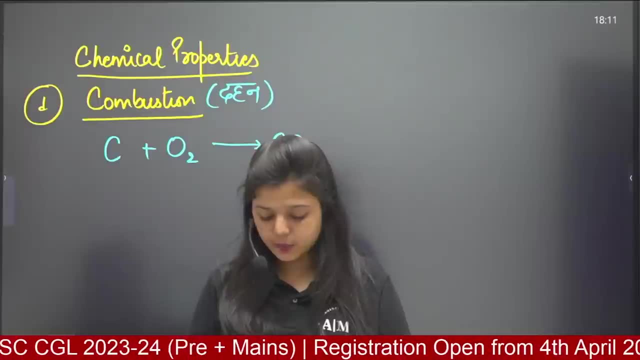 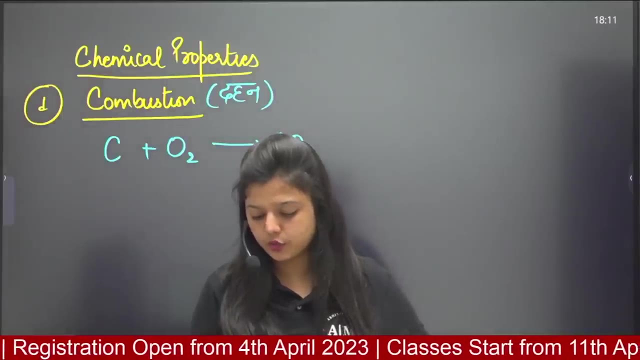 Carbon dioxide, which we call carbon dioxide, is made here and is ready. We get to see the property of combustion here. Tell me, was this clear to everyone? Daily classes are going on Every evening at 6 o'clock. your class is there. 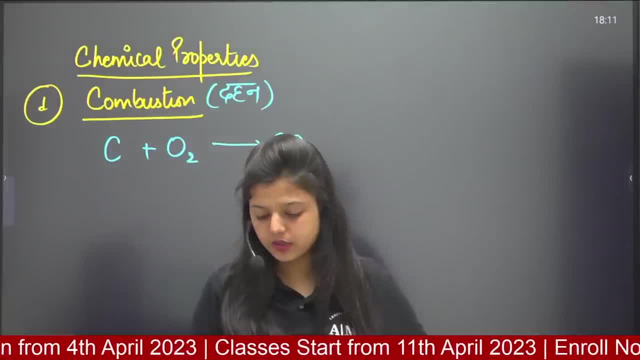 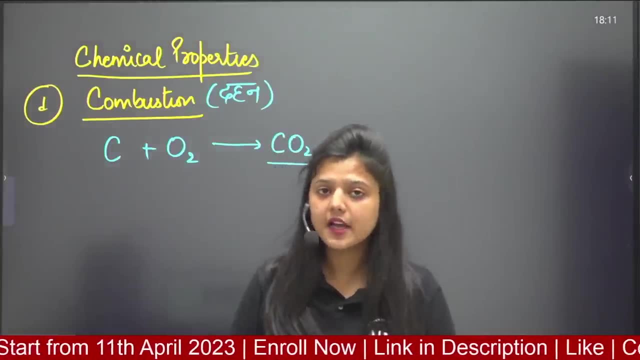 Okay, your class is at 6 o'clock every evening. There is no change in it. Clear, Clear, Clear, Clear, Clear. It is clear, Ma'am, this carbon dioxide has been made. Will something else be made with it? 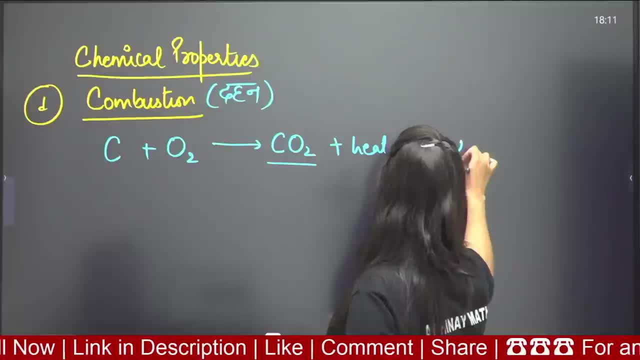 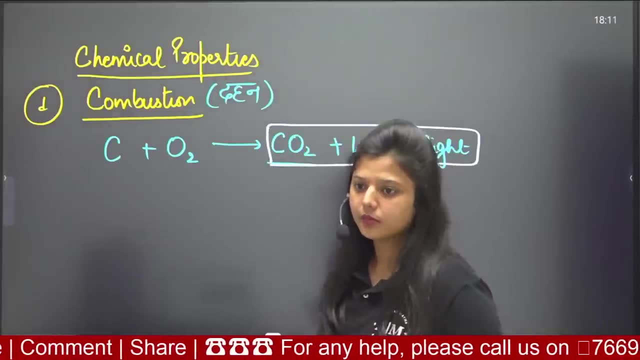 So you said yes, the heat will also come out and some light will also be visible to you. Is it true that we can see these products being made here? We took these reactants and burned the carbon in the presence of oxygen. What has become? 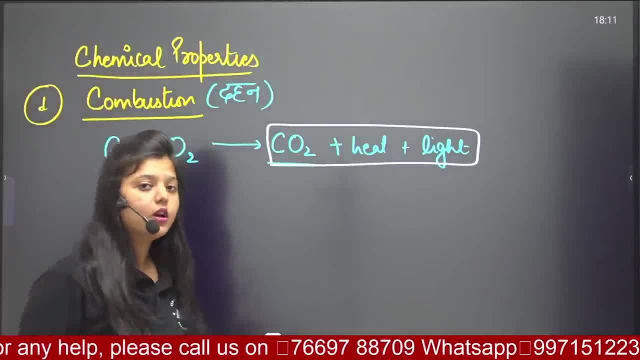 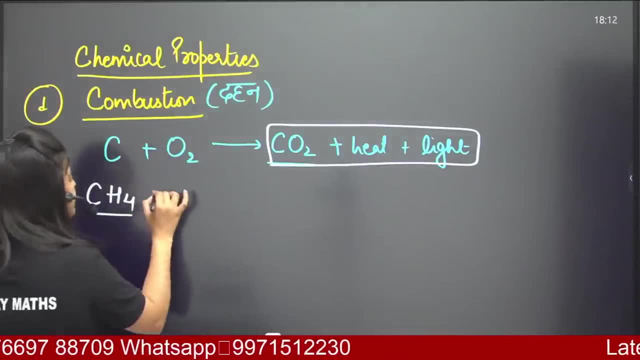 Some of our things have become like this. Now tell me one thing: If I take methane here, other than this carbon- I said it is CH4. Now, if I am reacting CH4 with oxygen, If I am doing the combustion process here, then what will happen? 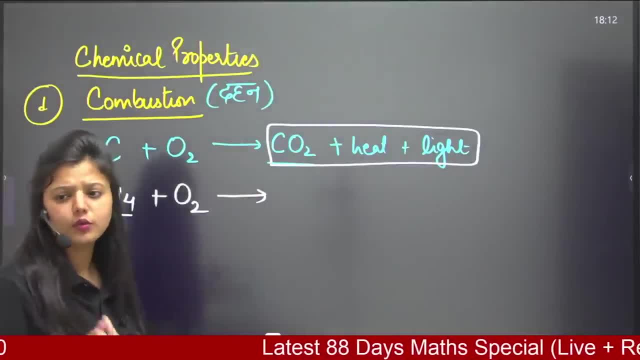 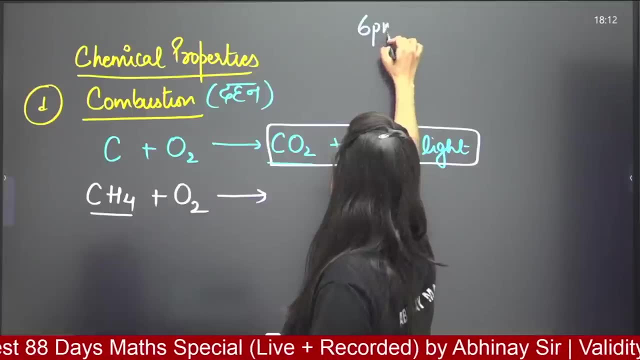 Will the same thing be made even then? Will there be a reaction or not? Tell me quickly once what can happen. You all know the timing of the class: Daily 6 pm, Isn't it Class daily at 6 o'clock? 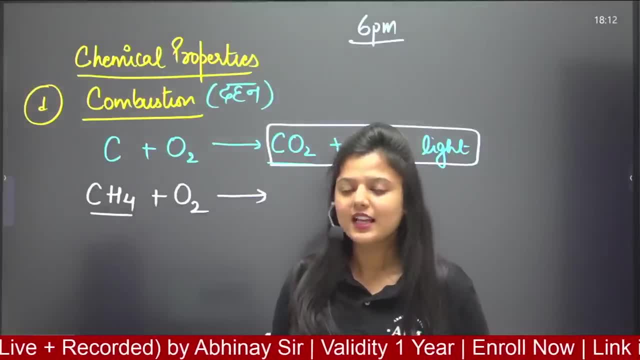 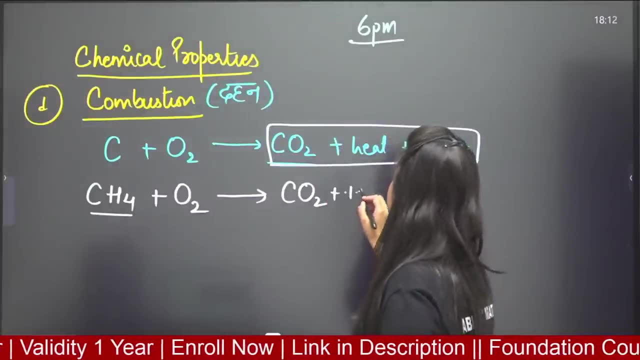 Ma'am, you get it here daily. It is simple, Ma'am. look, our CO2 will also be made here, But because hydrogen is also coming from the brother in methane here, So a molecule of water will also be made along with it. 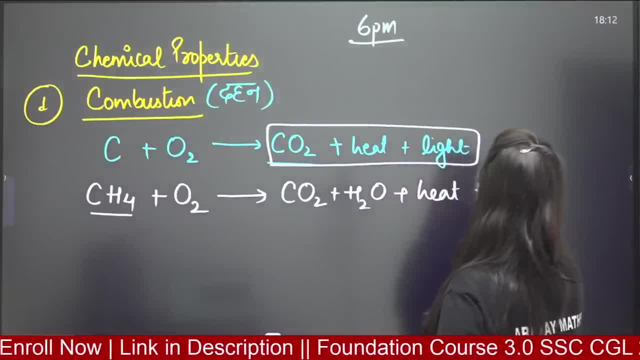 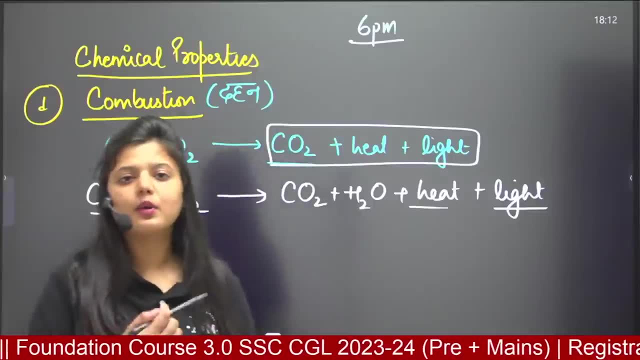 Heat will also be made. Heat will also be made and light will also be made. Heat and light come out together and you can see it. That means somewhere the process of the body is of different carbon. Whether I talk about carbon, I talk about the different compounds made from carbon. 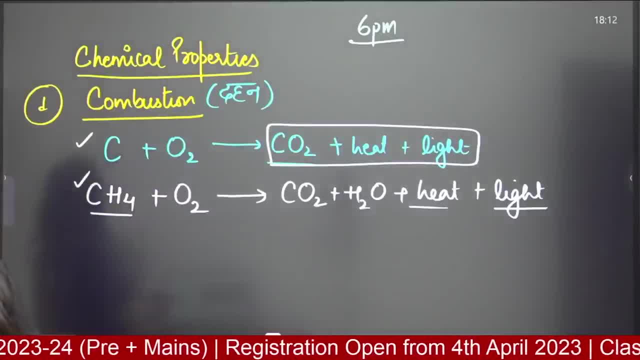 I have taken methane here. In the same way I will take the other compounds here. I talk to you about alcohol. Even then, we see the same process Absolutely. You say we talk about alcohol, Let's talk about CH3CH2OH. 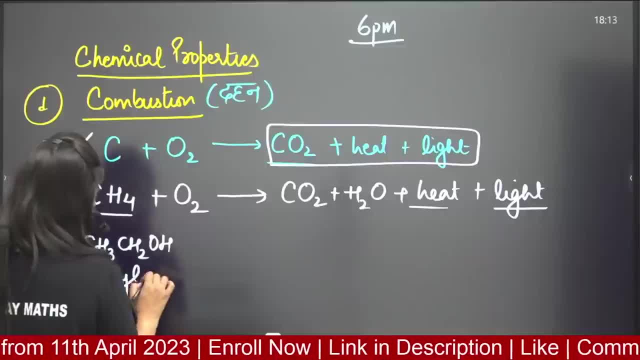 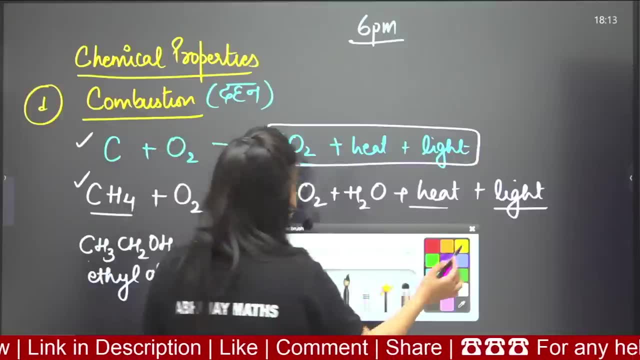 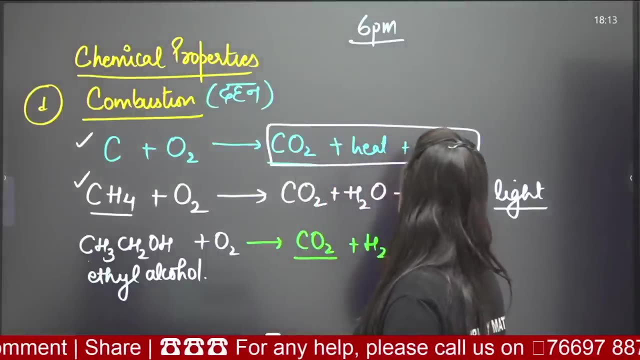 What did I take here? Ethyl alcohol. Okay, Ethyl alcohol. Even if I add oxygen to this ma'am, I will see the same reaction. One carbon dioxide will definitely come out, One water molecule will be visible And heat and light. 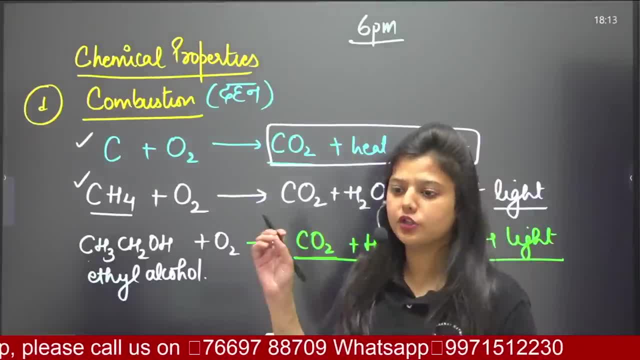 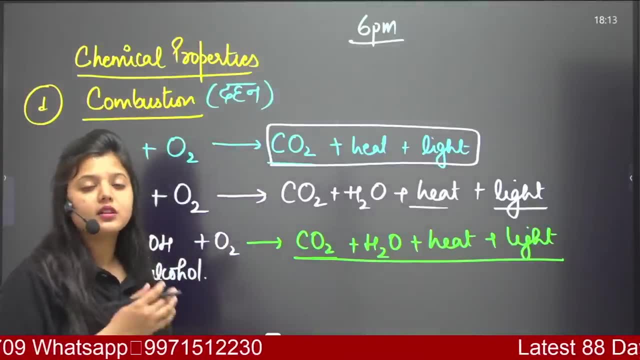 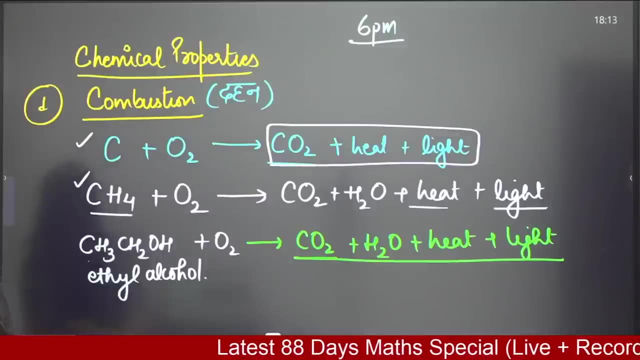 Whenever the body is there, these products will definitely be made for you. I mean, these products will definitely be seen being made. That's why we are calling it the property of the body. What did we do? by mixing it with oxygen, We started making heat, light, carbon dioxide and water molecules here. 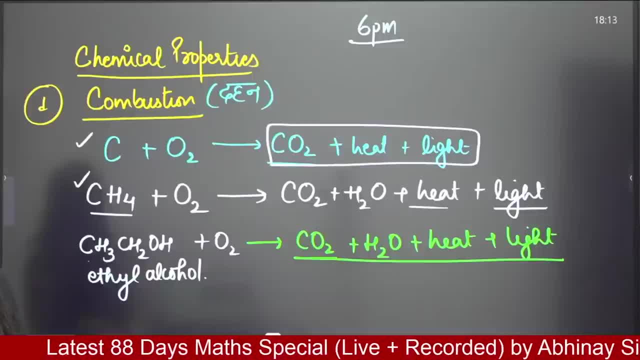 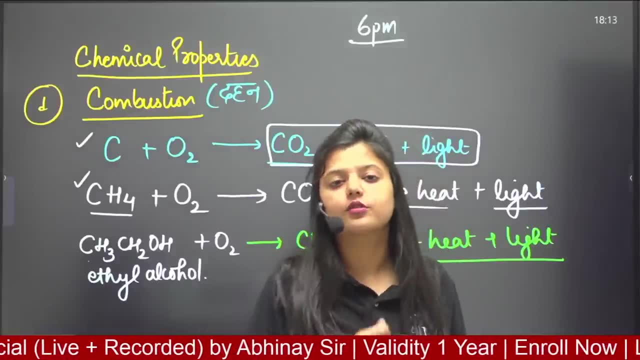 And these are all the processes of the body. If you have studied saturated hydrocarbons and unsaturated, you can see them in different ways. We told you that on the one hand, we have to make carbon dioxide. On the other hand, we have to make carbon dioxide. 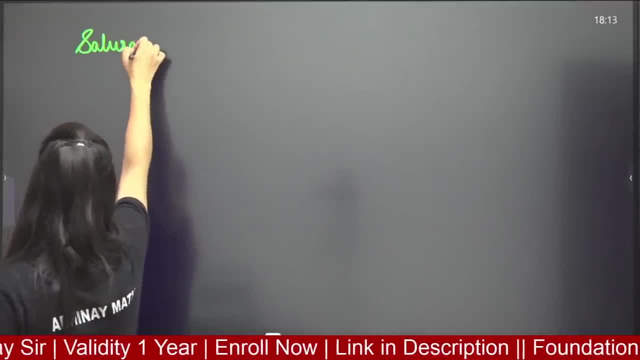 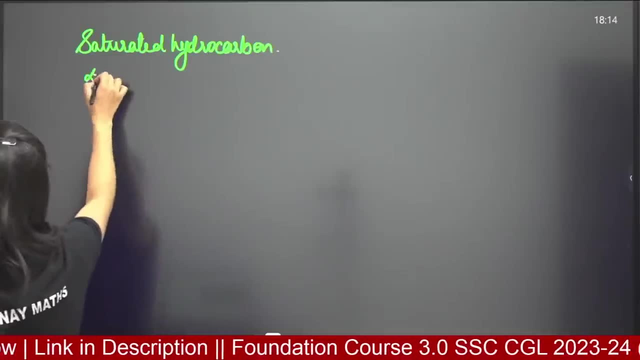 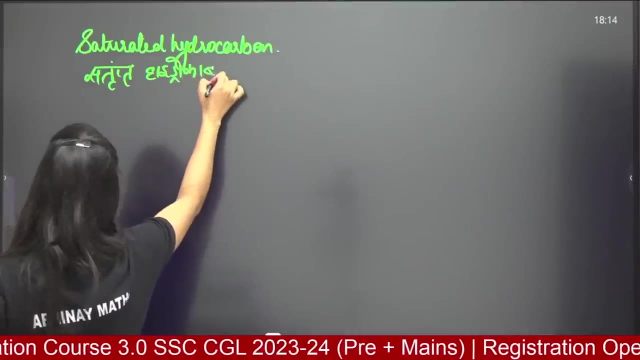 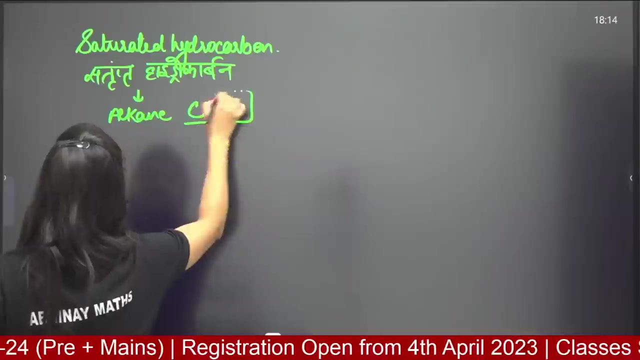 On the other hand, our alkanes come Saturated hydrocarbons. Saturated hydrocarbons- Saturated hydrocarbons: We had studied alkanes. in them, Alkane is a single bond between carbon and carbon. When we burn them, 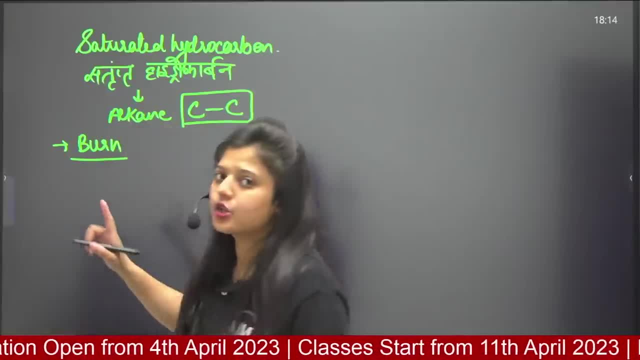 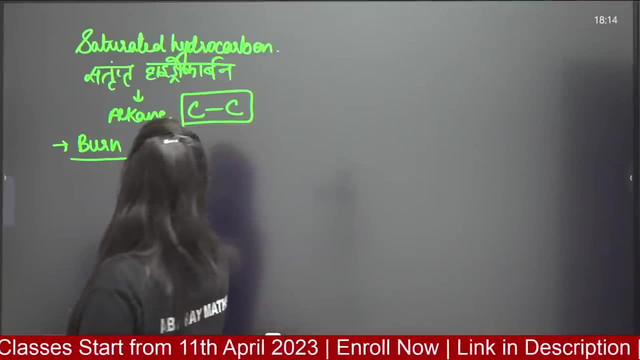 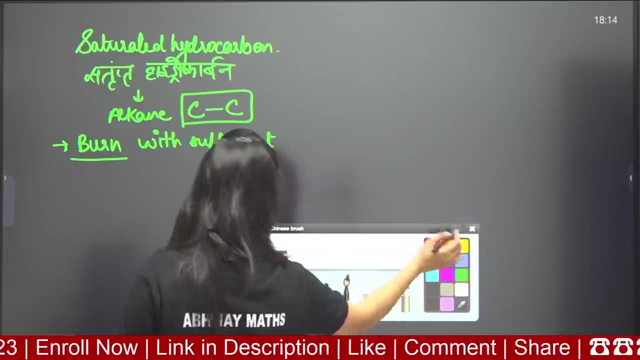 Okay, They burn, Okay, The flame that comes out with them. I told you that it is not yellow. You can see the blue flame coming out. They burn with sufficient amount of oxygen, Sufficient oxygen. And here you can see the blue flame. 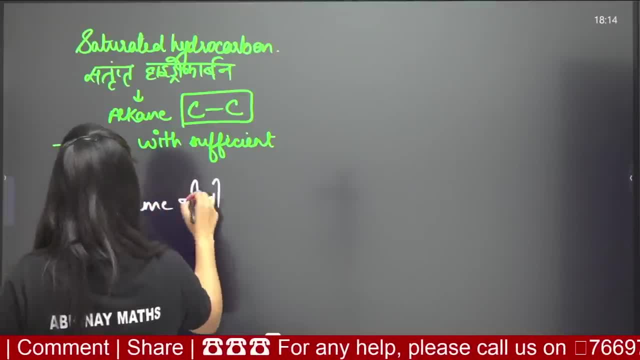 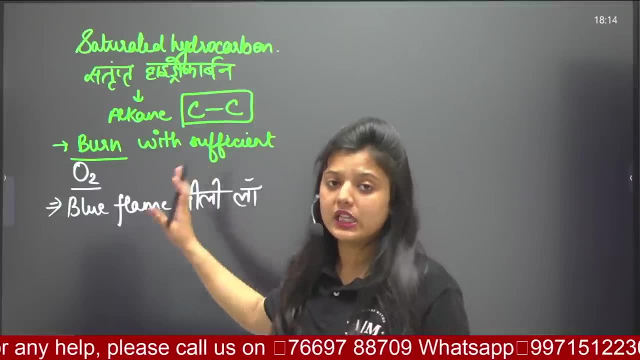 Blue flame, Blue flame. What does this mean? Combustion is happening here. You can see it properly. You can see the whole body here. Here you have the process of burning alkanes. There is complete combustion. So this question can also come from you. 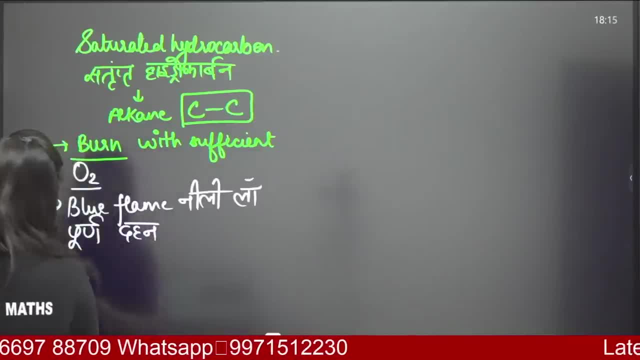 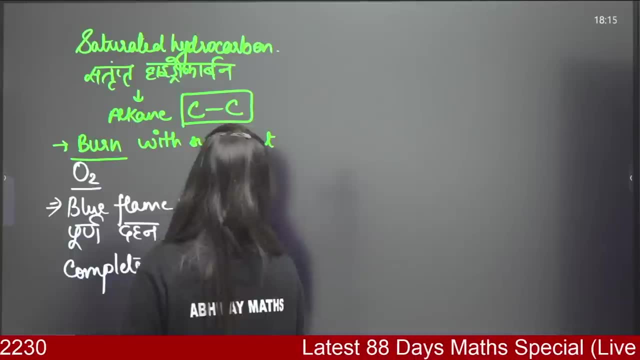 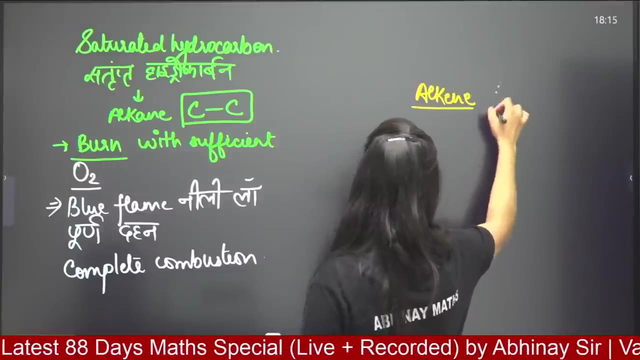 Brother, in whom is the complete combustion happening And in whom is it not happening? Here is the complete combustion. Tell everyone that you are understanding If we talk about this comparatively, If we talk about alkenes and alkynes. Alkene and alkyne. 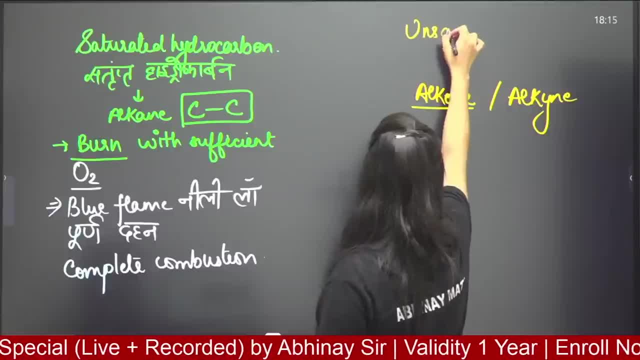 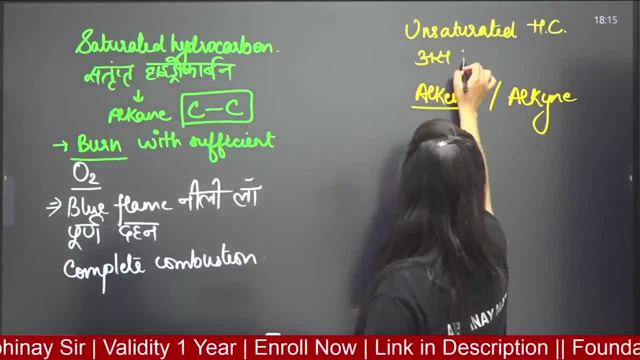 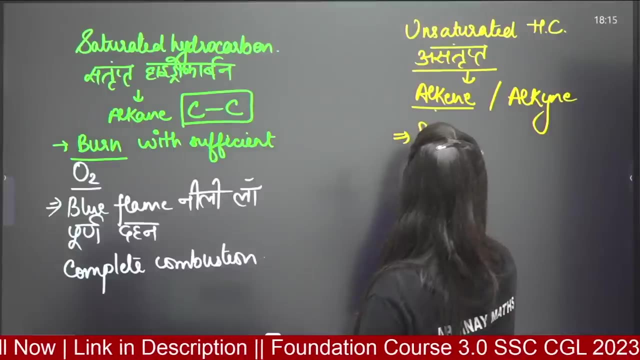 Which come inside, Come in unsaturated, That is, come in unsaturated, Unsaturated hydrocarbons Unsaturated. So if you look at these two inside them, So they burn with insufficient, What will be the oxygen? There will be less. 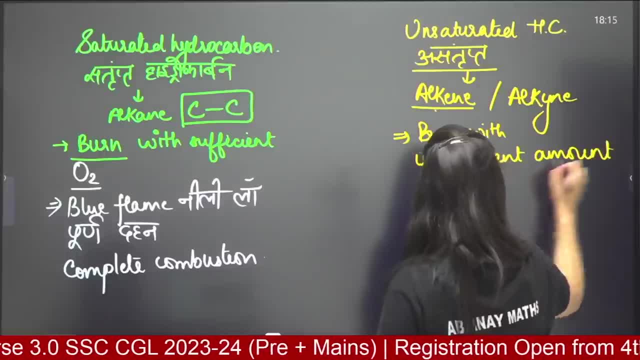 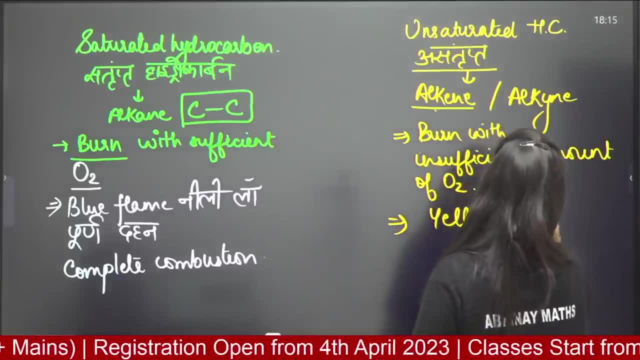 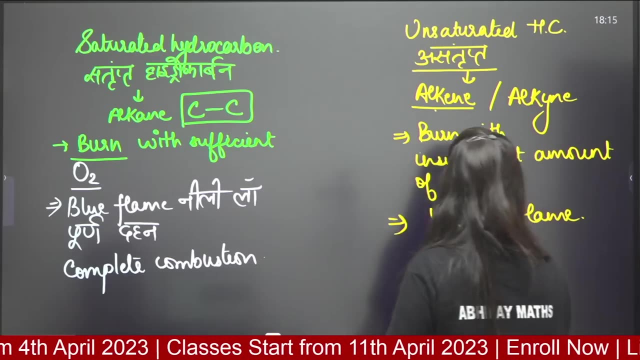 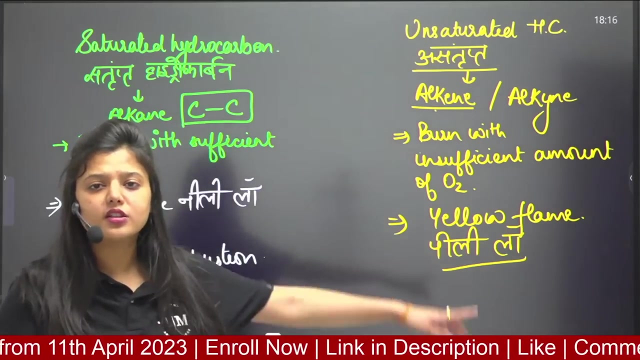 Insufficient amount of oxygen. Along with that you have yellow. here You can see the flame. You get to see such a yellowish red color. You must have seen many times that our gas stove The oxygen is not going completely. So when the oxygen does not go, the color of the flame changes. 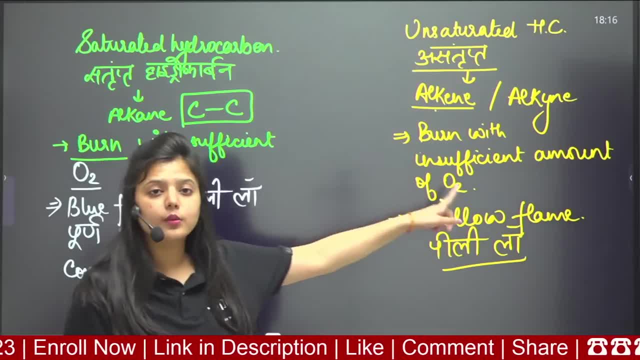 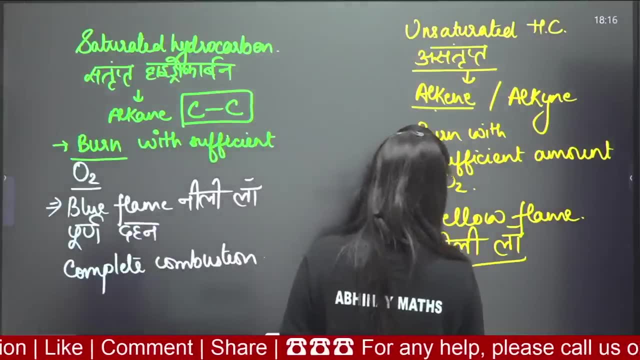 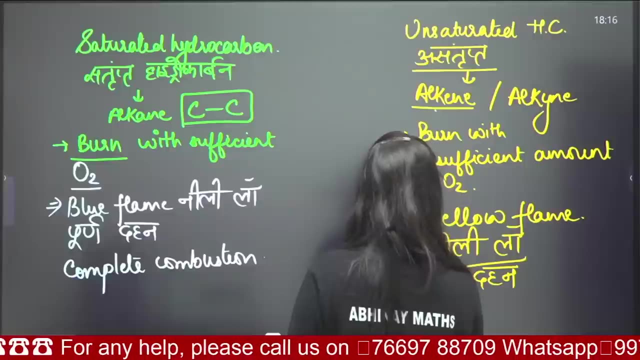 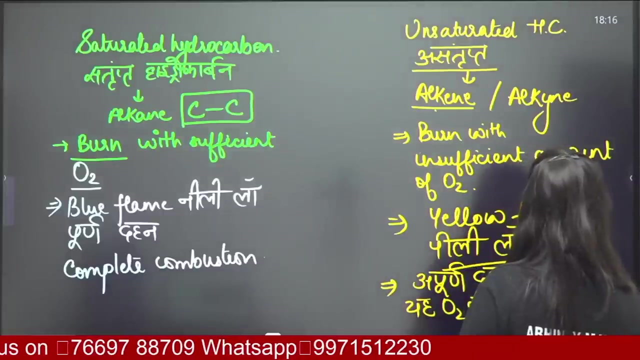 Something else happens here, When there is incomplete combustion, When things are happening in the absence of oxygen. So here is not complete combustion, Here you can see incomplete combustion. Here you can see incomplete combustion, Incomplete combustion. Why? Because it burns in the absence of oxygen. 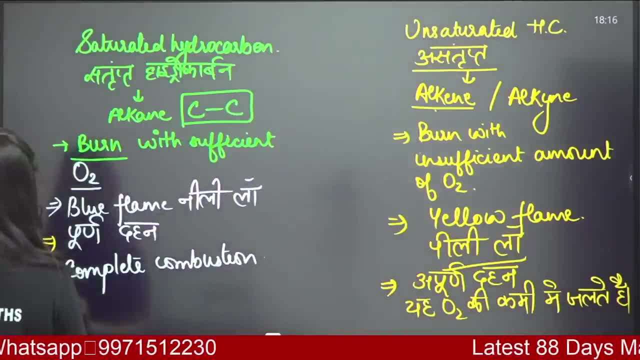 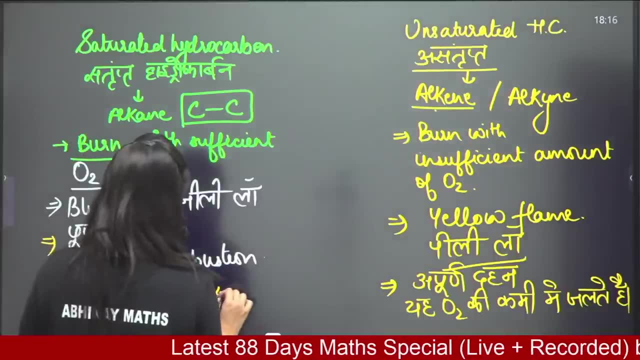 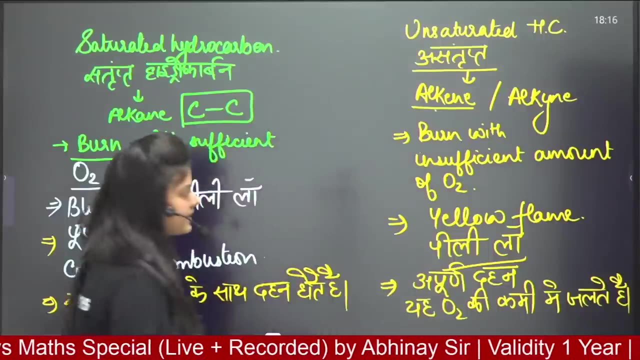 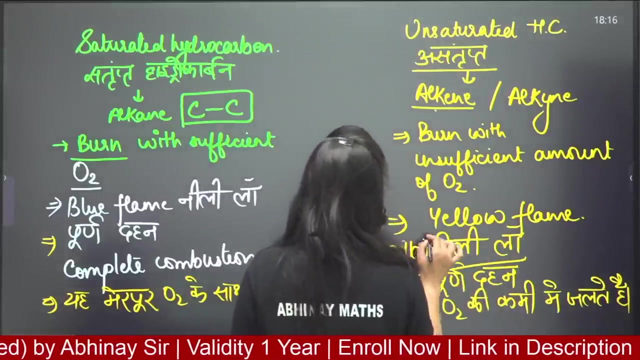 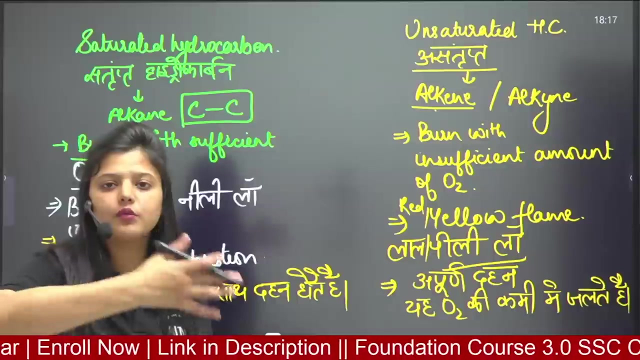 Okay, And if you talk about them, It is full With oxygen. There is a body. Call it, a body Burn. See, Any problem? Let's tell someone quickly. Once Yellow, yes, Red- also comes, Yellow red color, you will be able to see. 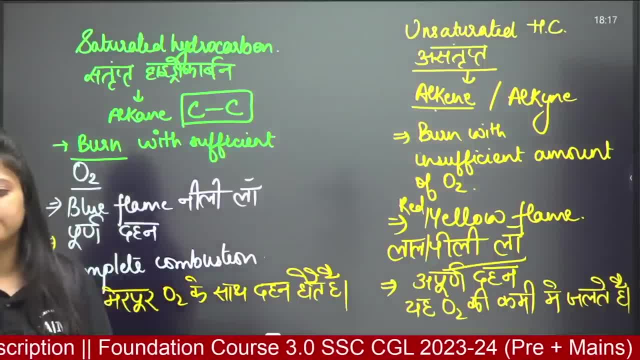 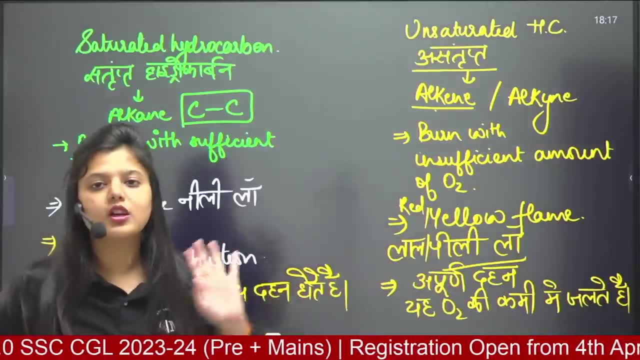 Yellow, red, Reddish. yellow means what is happening over there: The lack of oxygen. Your gas is properly not in the full amount of oxygen. It is visible burning in the full amount. but it is possible that in both cases I will see different. On one side there are alkanes and on the other side there are alkenes. 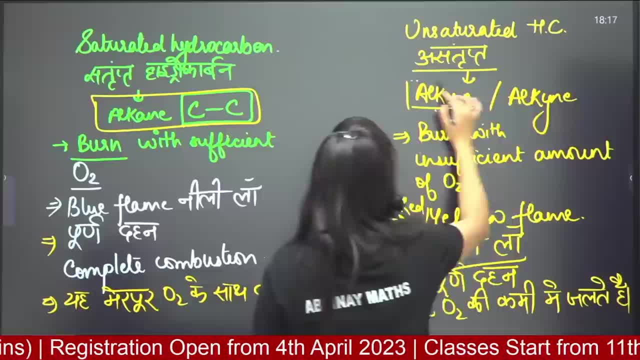 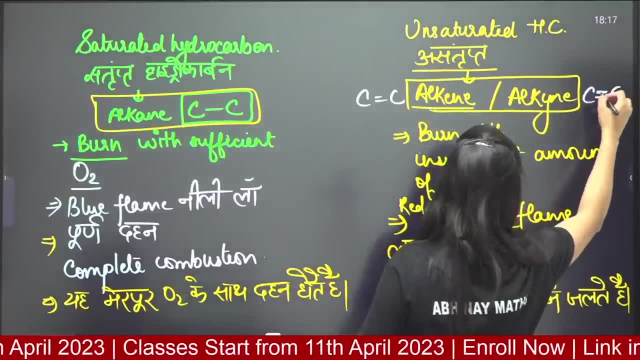 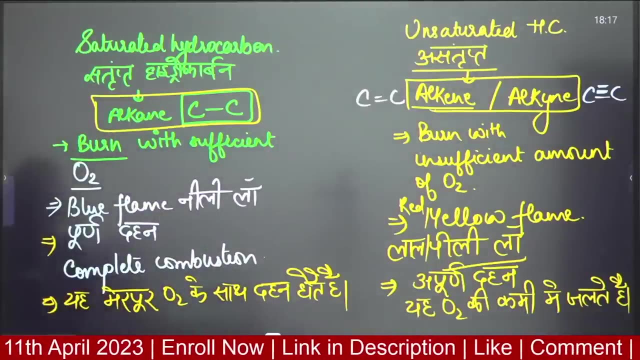 Write it as important mark: Alkene- alkene and alkyne- Alkyne. this is carbon double bond and this is triple bond. Take a screenshot. whoever is writing here: Yes, with oxygen it will work more. If it is oxygen, then you will see clean flame. 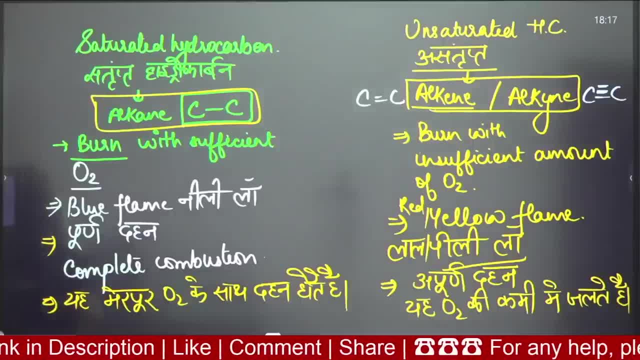 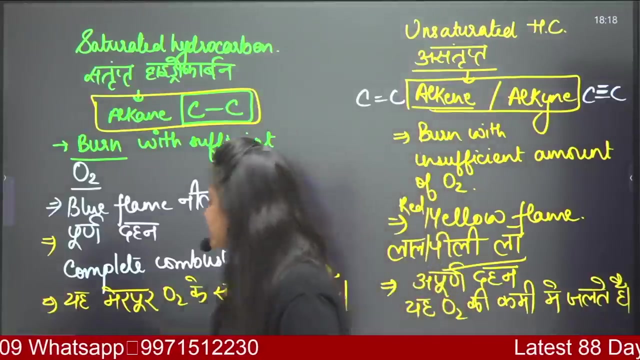 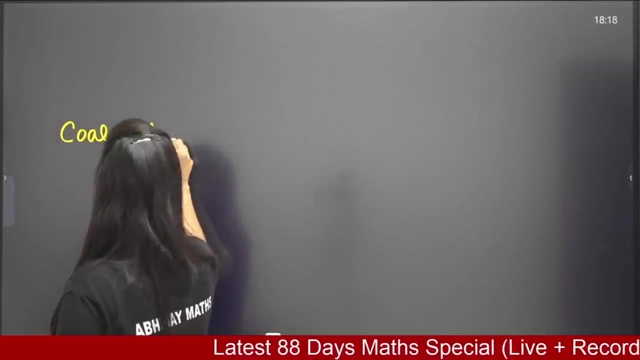 You have sufficient oxygen, You will not see yellowish black scene. Let's go Clear. This is how the story happened With this. we see that we are talking about coal. We are talking about petrol. We have burnt them. We have burnt them. 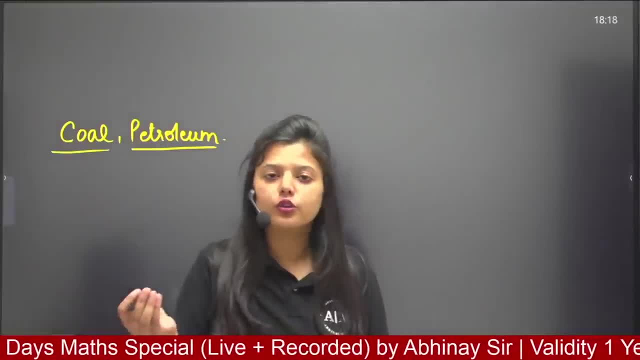 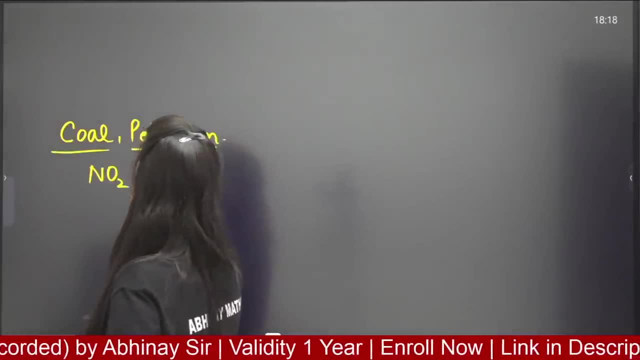 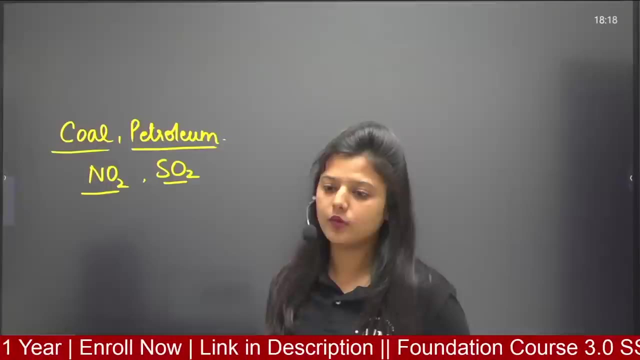 Now with burning, when they will go in the environment, then somewhere. in the same way, it will affect When you will burn them, then two mainly: one, NO2 and one SO2.. You can see these two things being made. Understand this concept carefully. This concept is important to you. that, ma'am, we have burnt them. 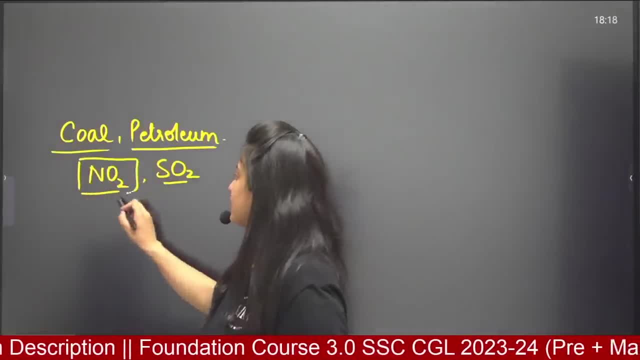 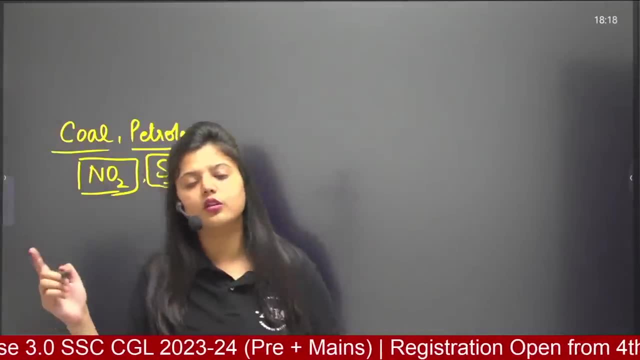 We use coal, we burn petroleum, After that, these two gases, These two gases are the most dangerous gases. Ma'am, it looks very calm, But when they are in the environment, and what happens then It rains. That means they are reacting with water. 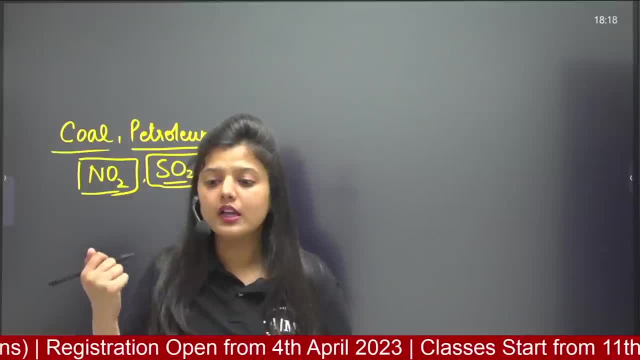 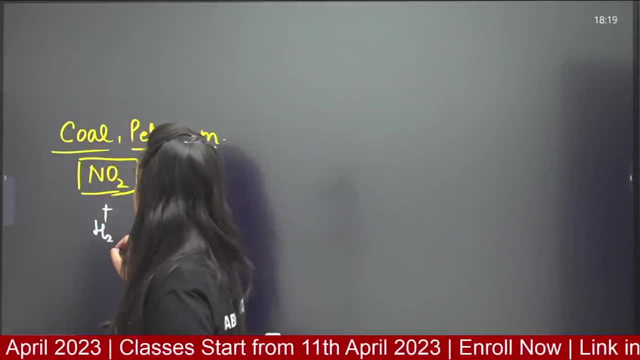 There are gases in the atmosphere. It is not just that there is only oxygen Or there is only carbon dioxide. There are all kinds of gases. Air is a mixture of gases. So what will they get with them? They will get water. 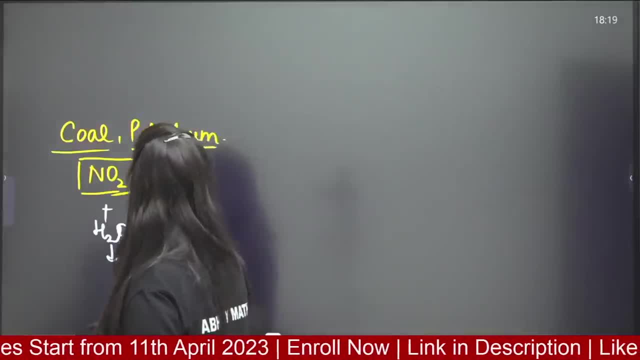 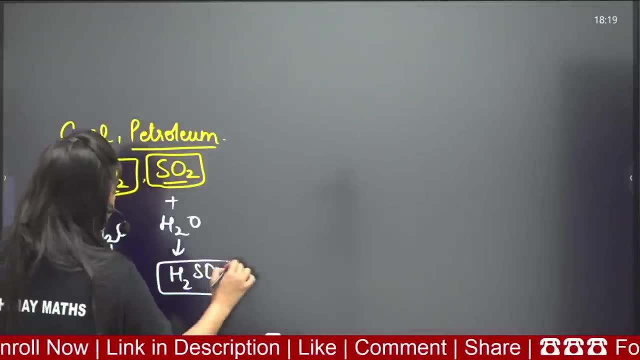 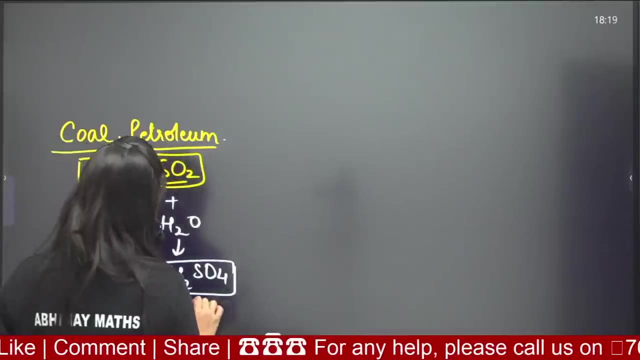 They got water with this. They got water with this. So, ma'am, these two, One makes HNO3 and one makes H2SO2.. H2SO4. H2SO4. That means nitric acid, And on the other side, your sulfuric acid. 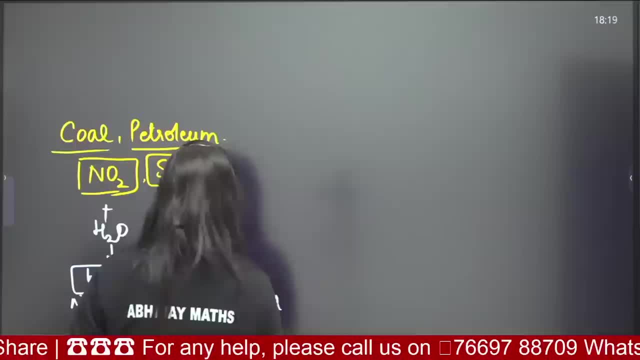 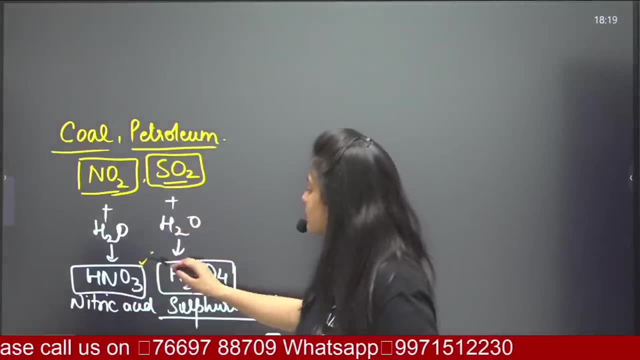 King of chemicals, which we call, Okay, The king of chemicals, which is called Now, when something like this happens. So, ma'am, because of these two gases, when this acid comes down from the sky, Carbon monoxide is also there. There are also many poisonous gases. 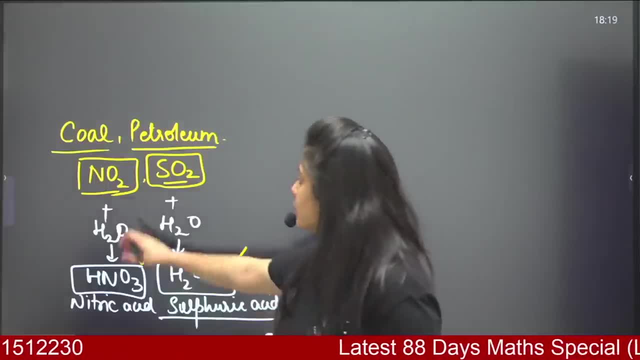 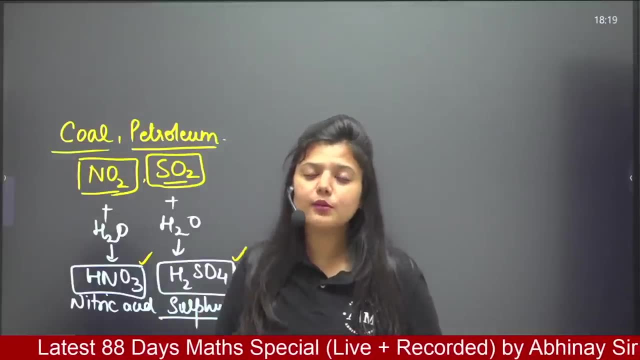 But mainly when, But mainly when I am talking. What are these two gases made of? They are made of ammonia and rain. You say acid rain is happening, So where did the acid rain come from? Just think and tell me, Ma'am. you are saying this again and again. 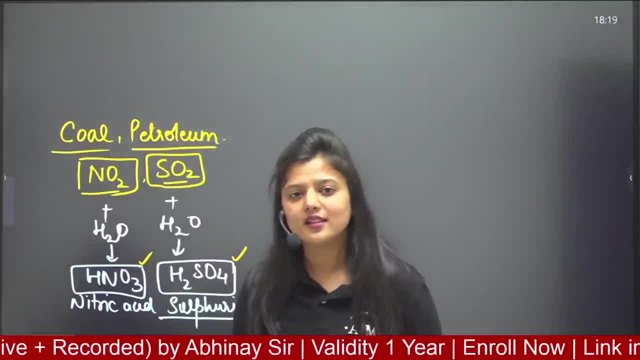 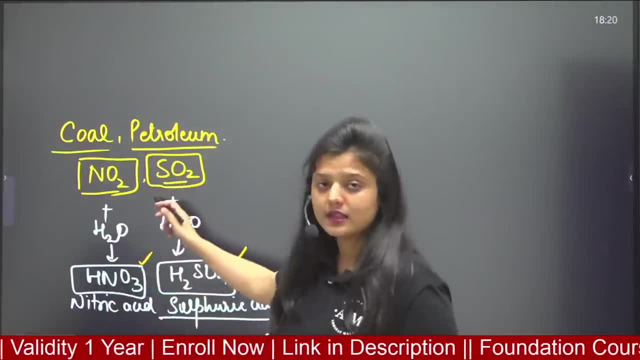 It is raining and acid is coming in the rain. Where does this acid come from? I mean from where There are gases in the whole atmosphere. So this acid becomes when water mixes with these gases And this nitric and sulfuric acid, which is highly acidic. 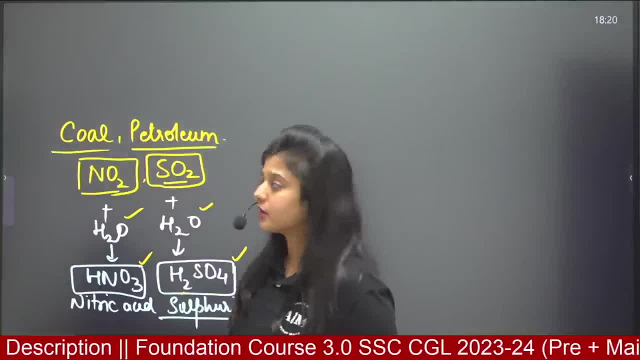 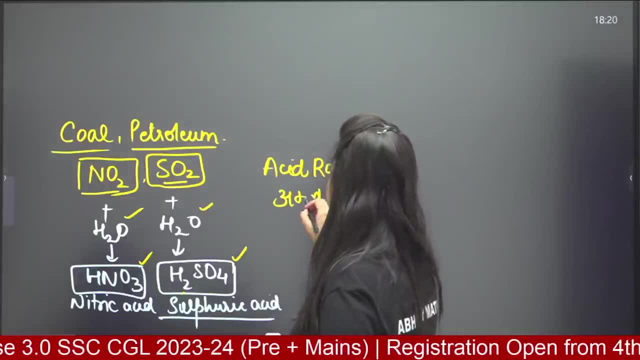 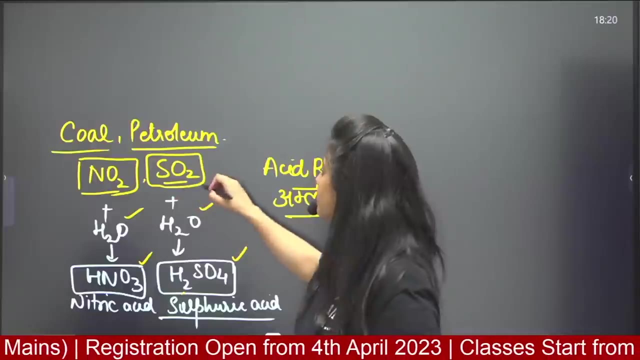 It works to make them. And ultimately, what do you see? Because of this, your acid rain. What do we call it? Amliye Varsha, Amliye Varsha. This is the main reason for this. So the question directly asks which two gases are working in Amliye Varsha. 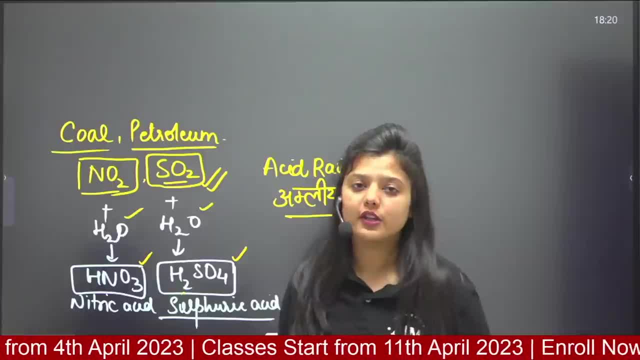 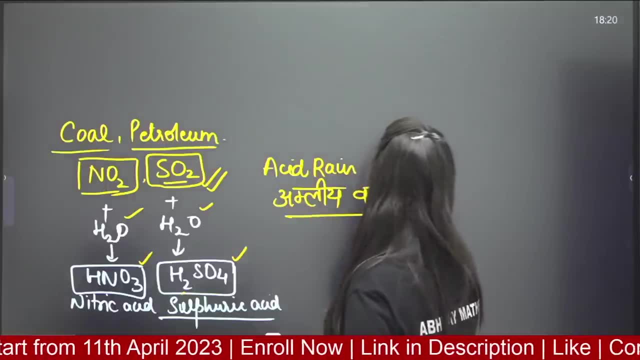 You will say nitrogen dioxide and sulfur dioxide. These are the main gases which are the reason or responsible for the acid rain. And because of acid rain We have seen a very common thing: What is the color of Taj Mahal? The stones of Sang Marmar have turned yellow. 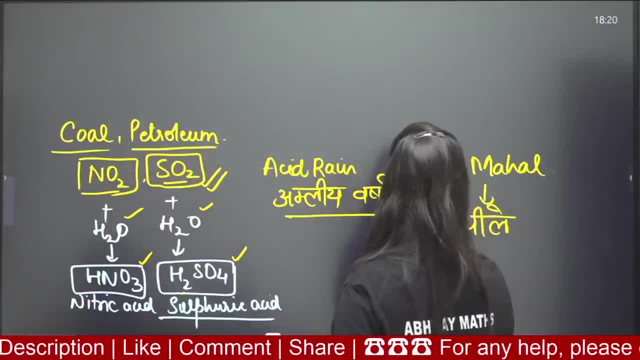 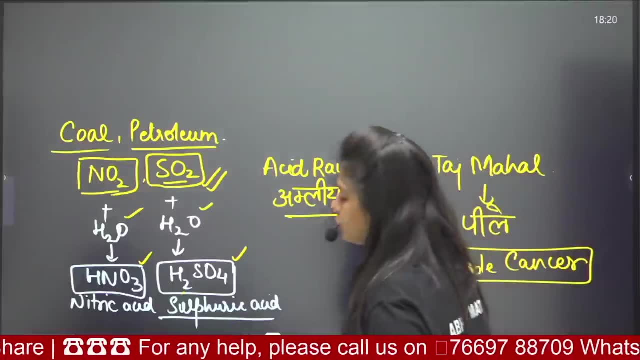 What have they turned yellow? They have turned yellow And along with its yellowness We had heard another name here, That brother marble cancer has happened. How many people remember that when this news of marble cancer came, That refinery, which is the Mathura refinery, near Taj Mahal. 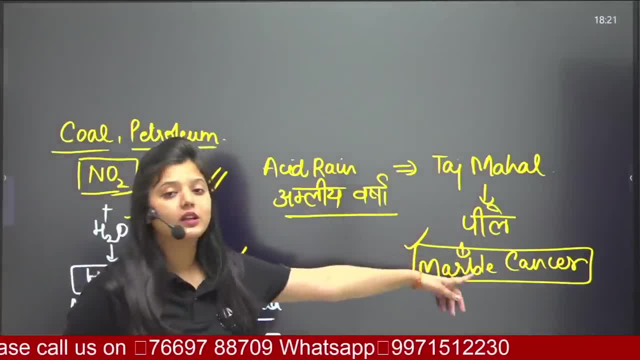 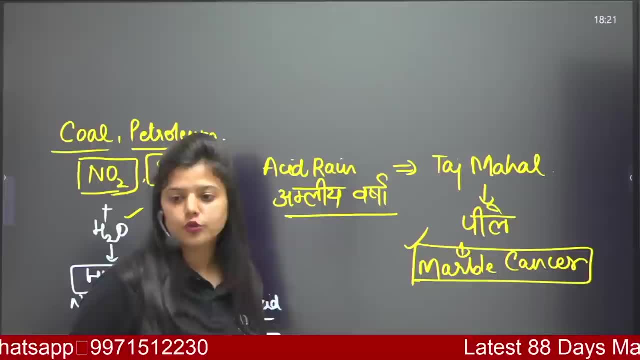 There is a lot of pollution from there And ultimately, marble cancer has happened. We can see the yellowness of Taj Mahal. in this way, The reason for the pollution is being made here. Okay, So this story is a round trip. 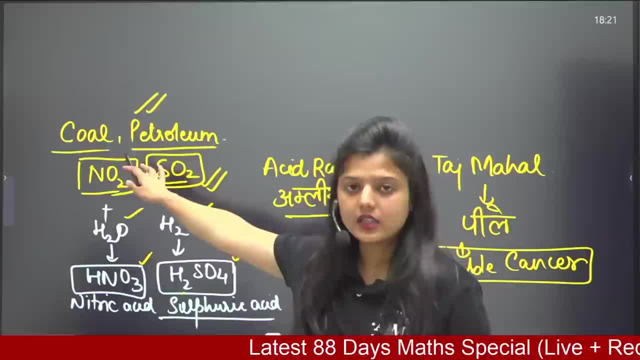 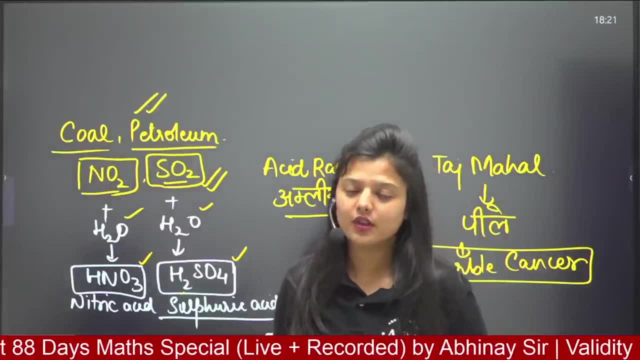 Who came from here? It started from here. Where did the beginning come from? From here, We can also see that they had a combustion. And when there was a combustion, what was made? These two types of different gases were seen to be made. 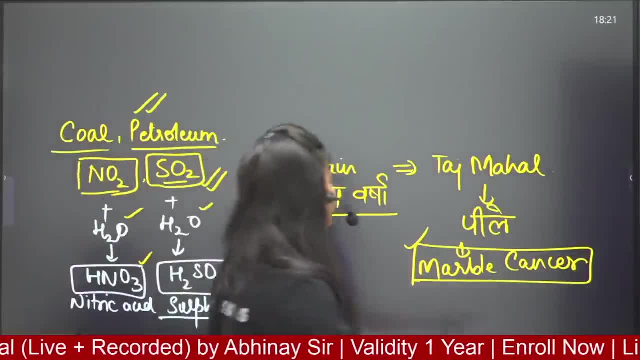 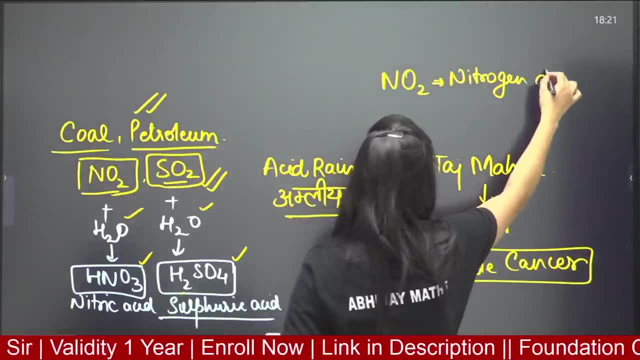 Tell me whether everyone is clear or not: N2.. Do not you mean Understand here. This is NO2.. This is nitrogen dioxide, Which we call nitrogen dioxide, And If I say N2O, So this is nitrous oxide. 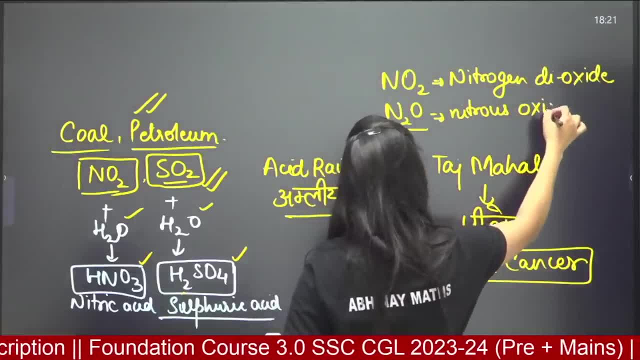 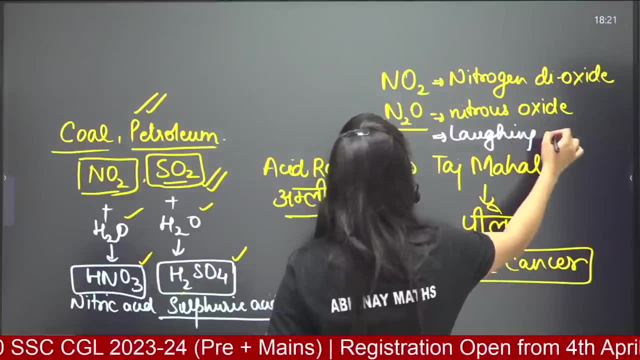 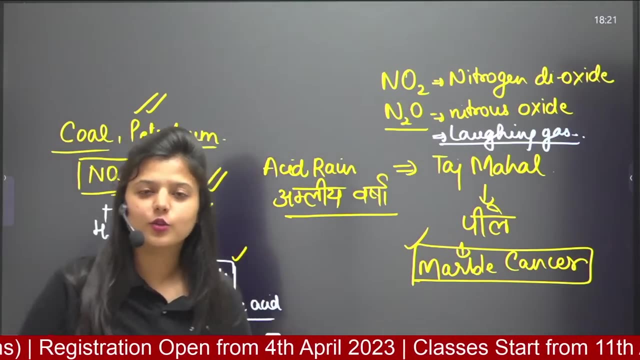 Nitrous oxide. This is called laughing gas, Laughing gas, Laughing gas. Everyone must have seen the movie laughing gas. Okay, Brother, if this gas spills out, Then you start laughing for no reason. People make you crazy. Now, whatever the matter is, 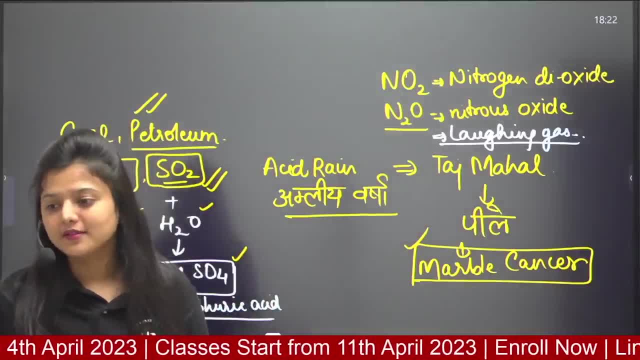 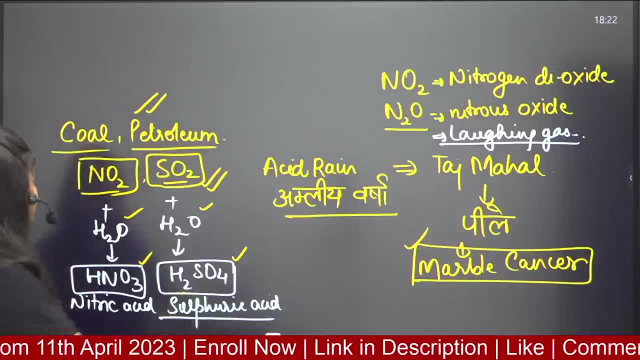 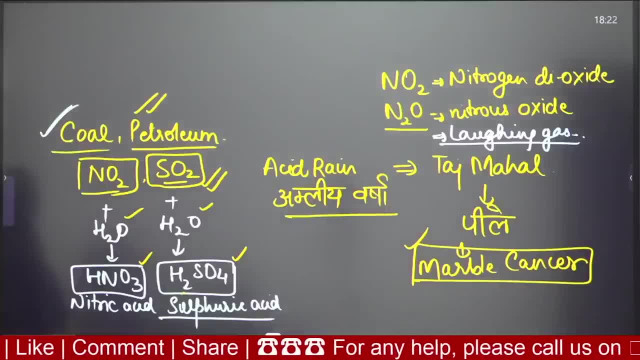 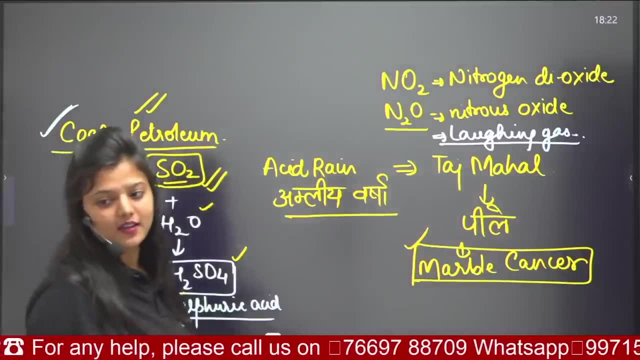 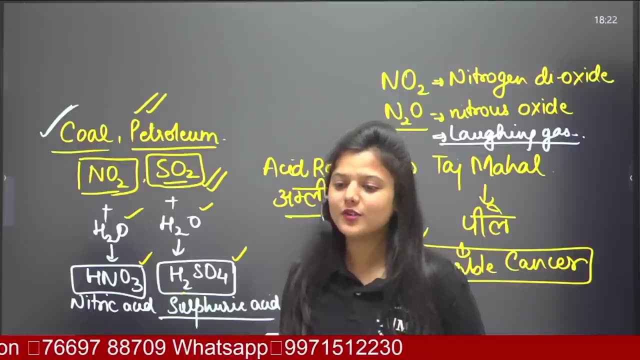 Quickly note: Yes, Do you see the movie names You remember so quickly. Now I will ask which enzyme of there was working. Then you will forget everything immediately. you will forget everything, Ma'am. there are some such issues. So this is what we have studied: the combustion reaction. 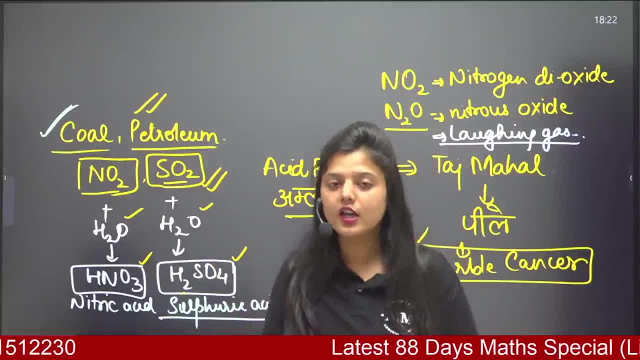 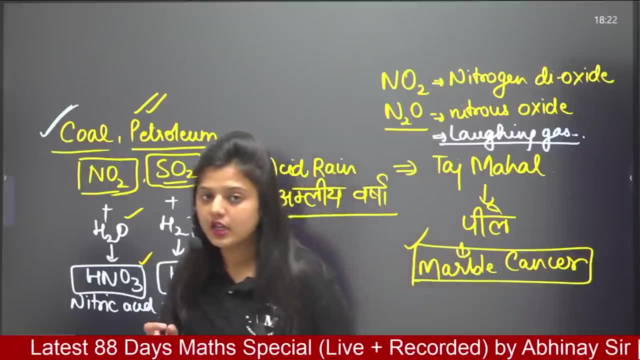 Similarly, the oxidation happens, the addition happens. so we will study every reaction one by one here. If I tell you that oxidation is happening here, that is, there are also processes of oxy-current, which makes your organic compounds what from what. 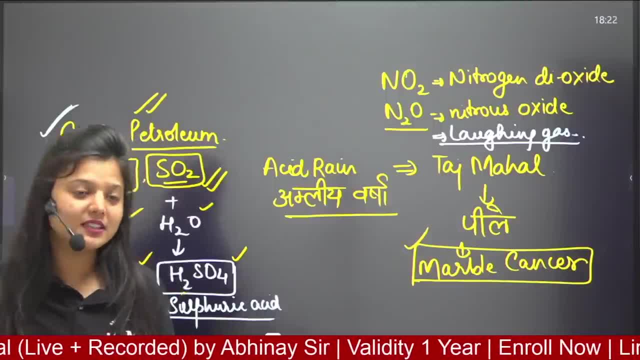 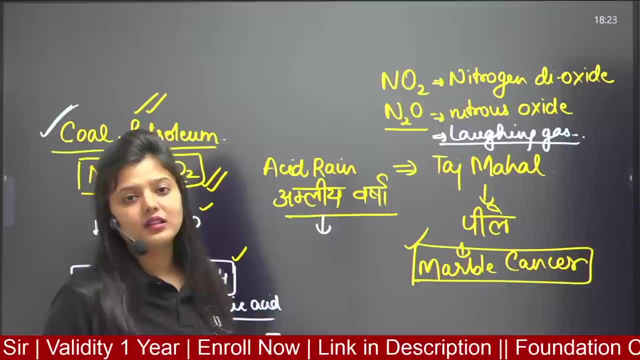 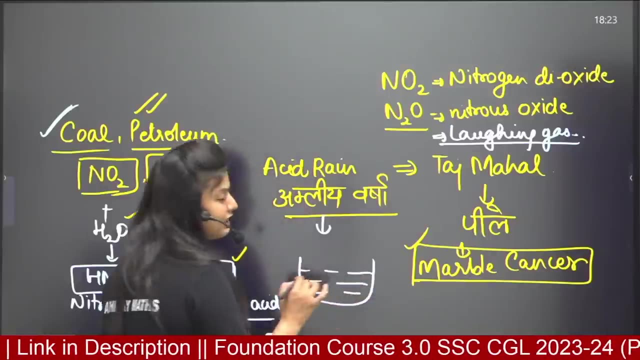 Which makes your organic compounds? what? from what Here? the acid rain? you see it, mainly it affects all kinds of living organisms, on the soil, on everything, Your river body, in the water body, all the different organisms. it works to kill them. 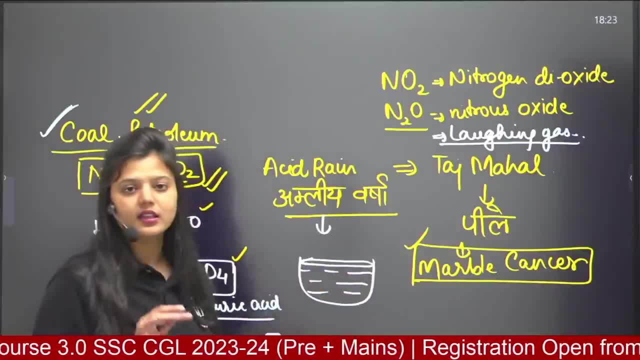 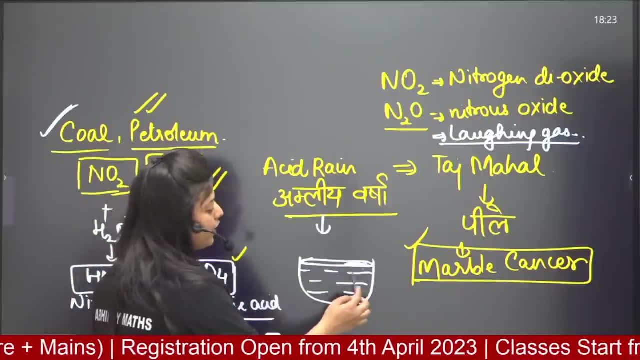 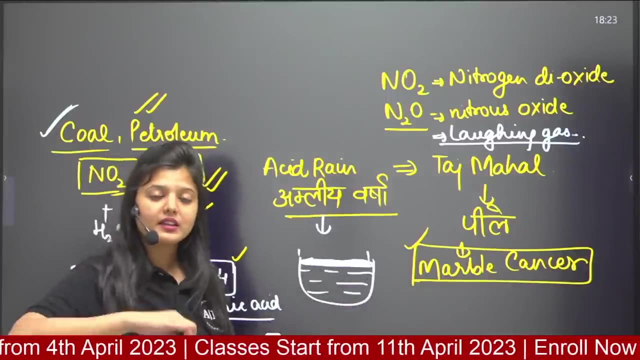 And ultimately, when the acid rain is happening here, when the water is accumulated, then all the organisms in the river, body, aquatic living organisms, they die Along with that. you see, we say algal bloom happened, eutrophication happened, 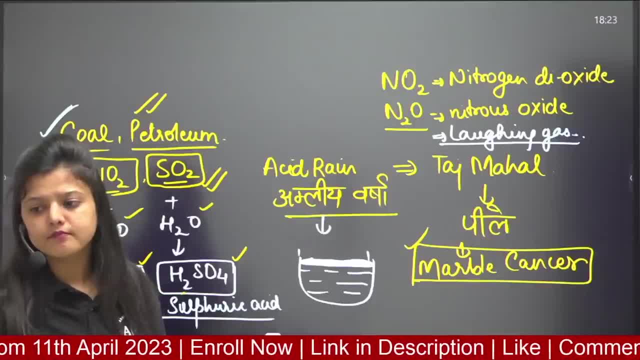 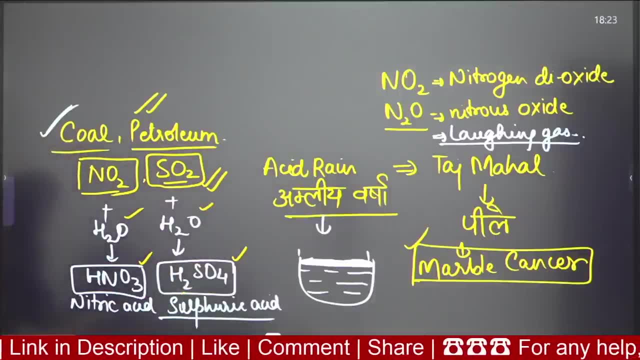 we see all these cases. It is a very old news of Marble Cancer but yes, Marble Cancer happened because of this. It happened because of this. it was seen here. Come on, write the next reaction quickly. Our next reaction is: 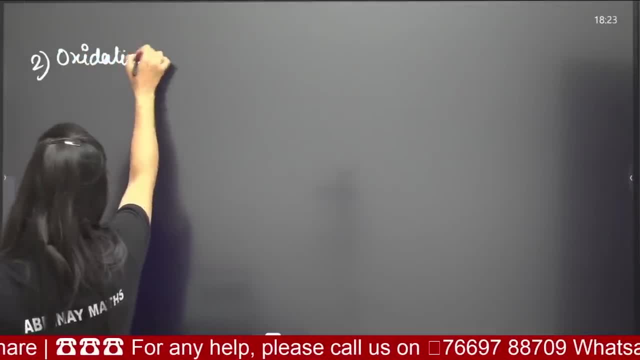 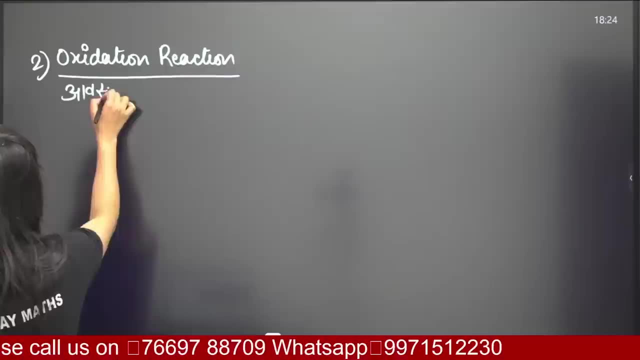 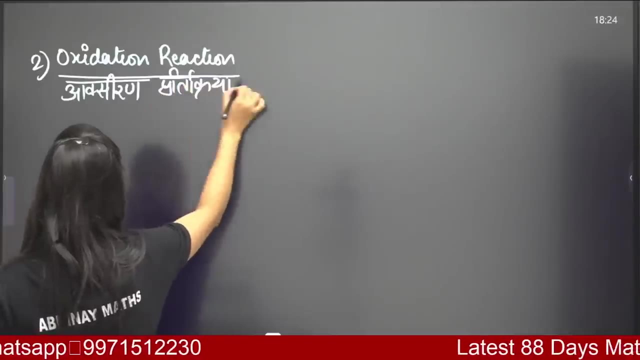 oxidation, Oxidation reaction. Oxidation means oxygenation, Oxidation reaction, Oxidation reaction, Oxidation reaction. Now, what will happen in Oxidation? Ma'am I took CH3CH2OH. I took CH3CH2OH. 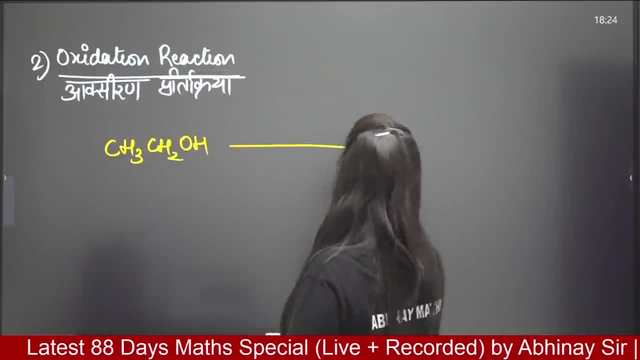 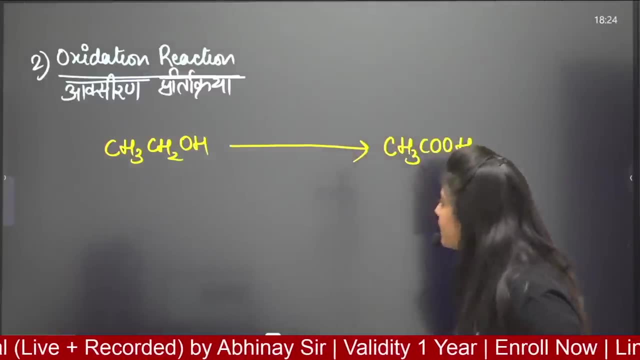 I took CH3CH2OH And what did I make from this CH3CH2OH? I made CH3COOH. I made CH3COOH In this reaction. what do you understand What happened here When I took Ethanol here? 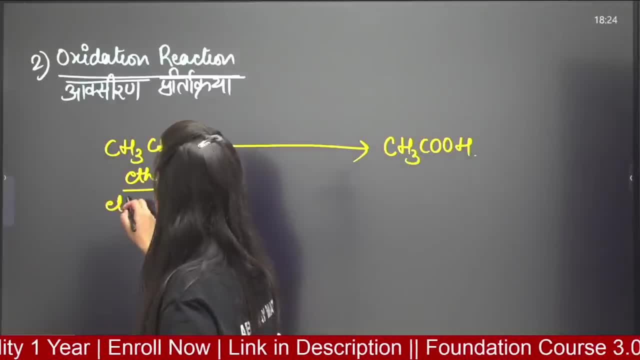 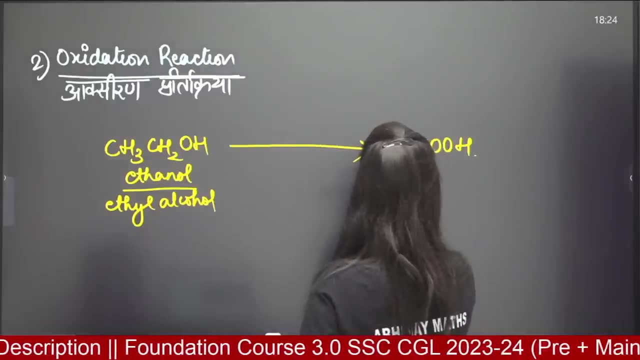 Understand the example carefully. What is Ethanol? Or we can call it Ethyl alcohol, Ethyl alcohol. What did I make from this? I made Ethanoic Acid. I made Ethanoic Acid, Ethanoic Acid, Ethanoic Acid. 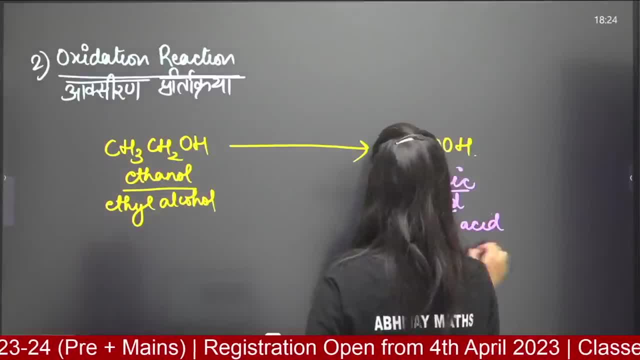 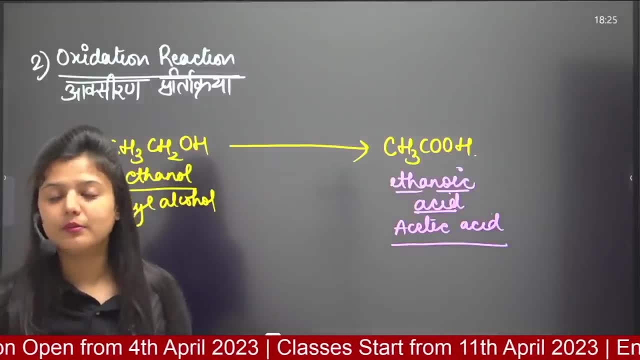 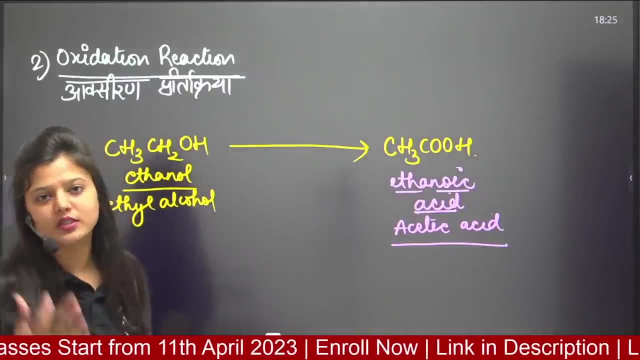 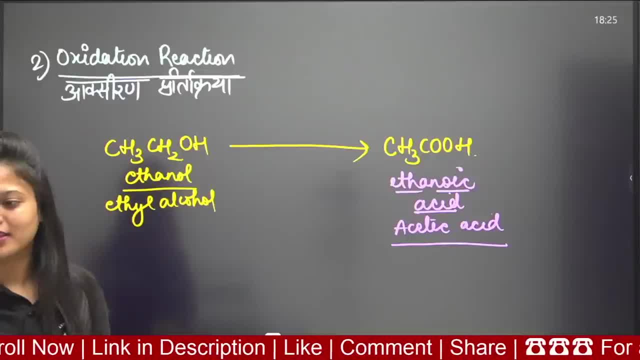 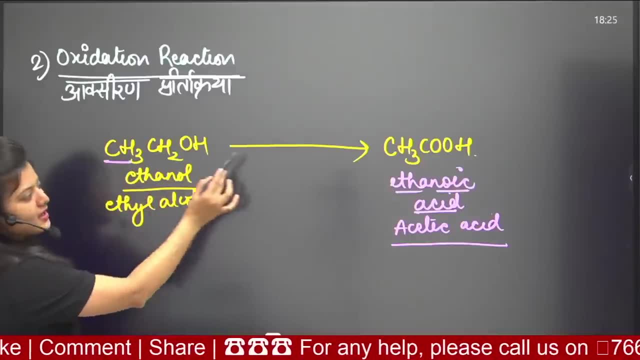 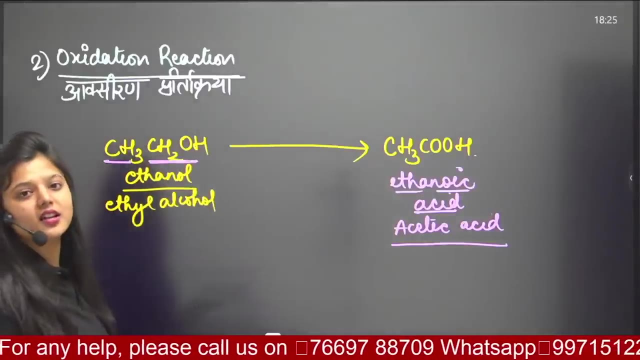 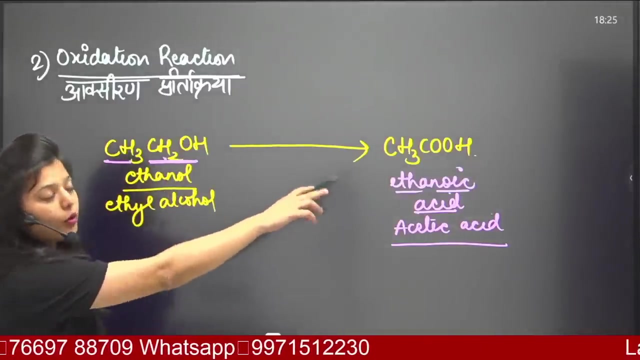 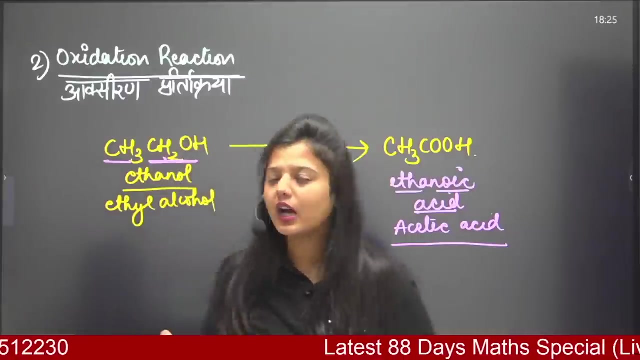 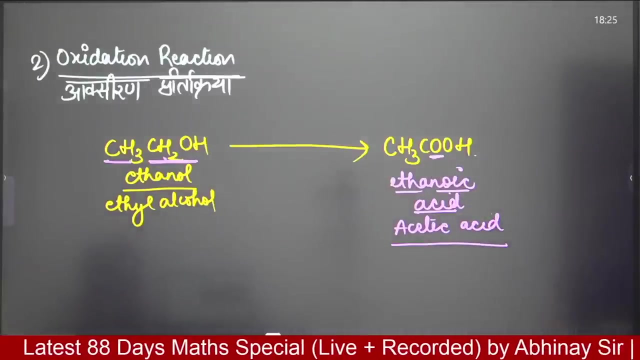 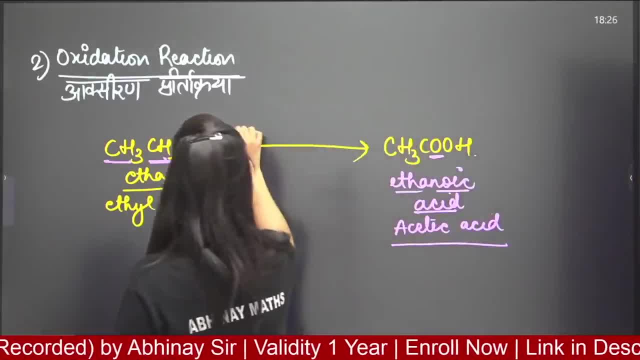 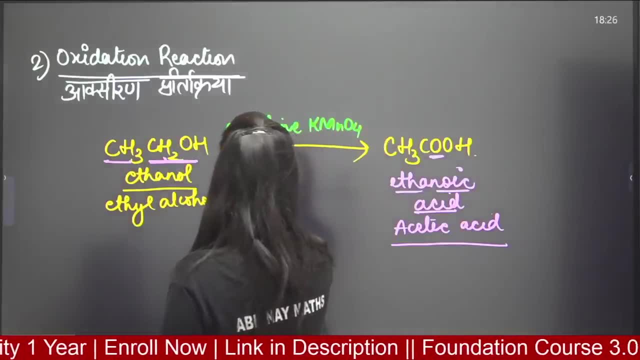 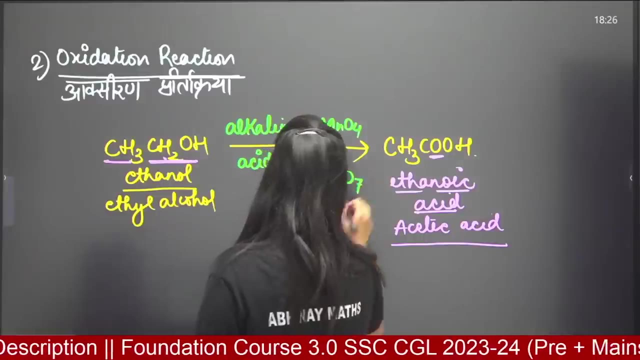 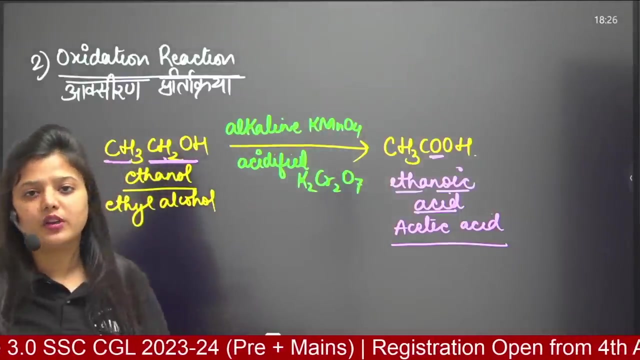 There are some agents that do all these things that work. here we will talk about alkaline KMnO4 and acidified K2Cr2O7 potassium dichromate. they are working to do this oxy current, that is, it is helping here like an oxidizing agent. oxidation reaction is happening here. you can see that an H2 has disappeared from here, then an oxygen has come out of here. 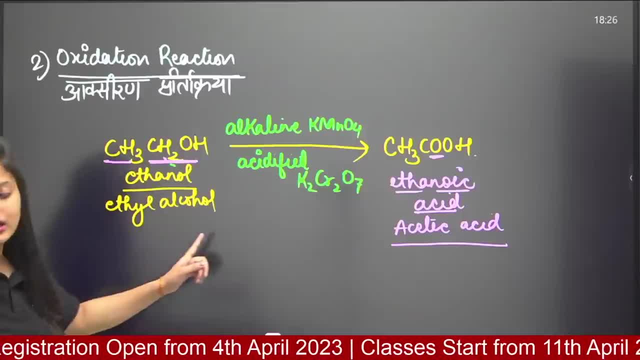 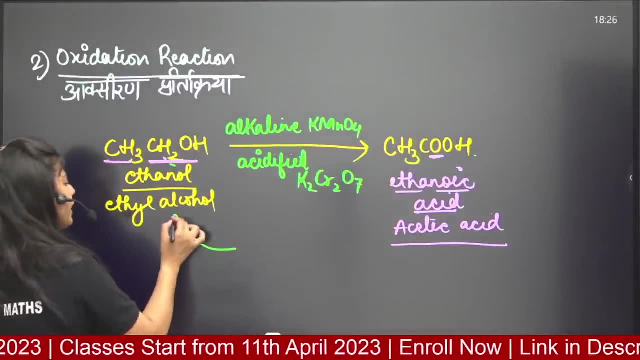 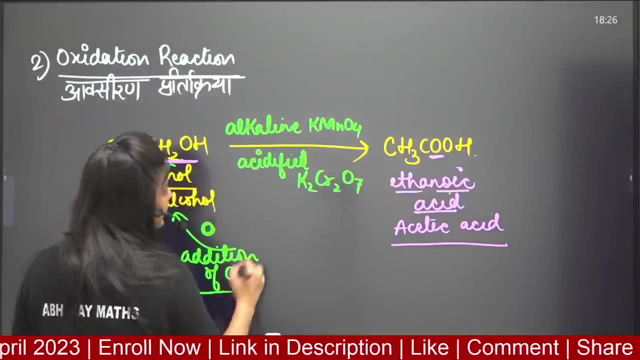 an oxygen has been added there and this conversion is happening of an alcohol in which one carboxylic acid in one carboxylic acid. so, ultimately, the addition that has happened here, whose oxygen? you can write that the addition of oxygen has happened, addition of oxygen, and this is working as a catalyst here, due to which your reaction is possible. it is important to write it once. 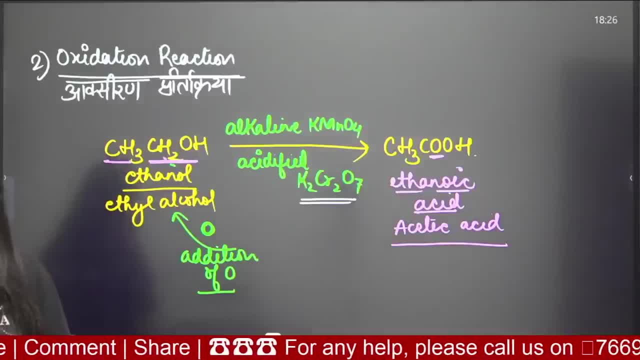 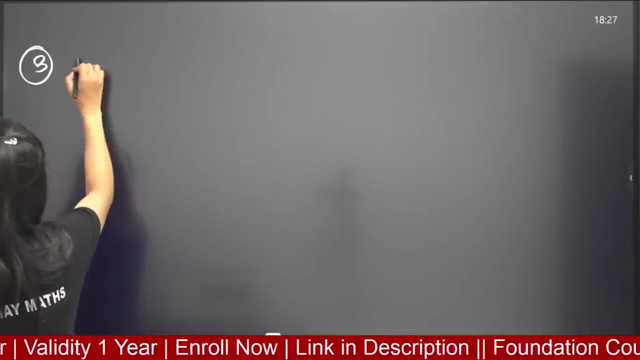 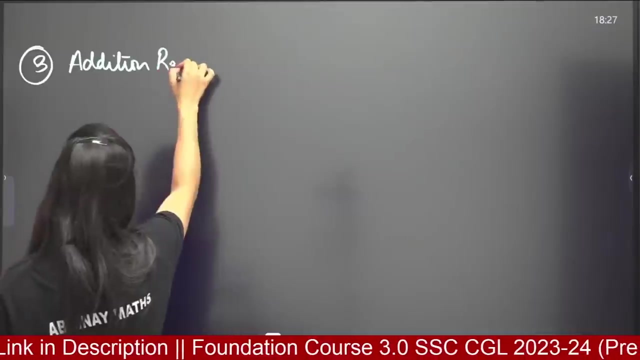 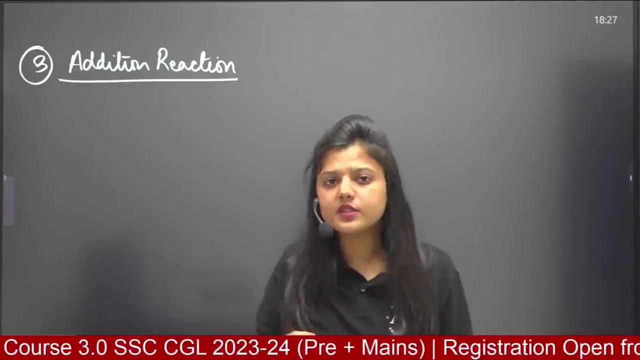 okay, note it here quickly. okay, note it here quickly. everyone clear. Next comes the third reaction, which is called hydro or addition reaction. welcome to the third reaction. I am doing something is adding. Watch from. Are there anything? What is it? 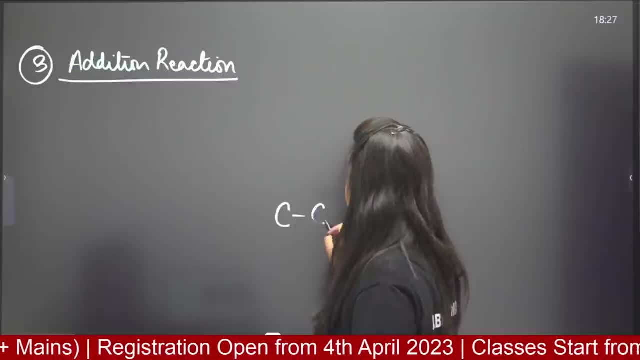 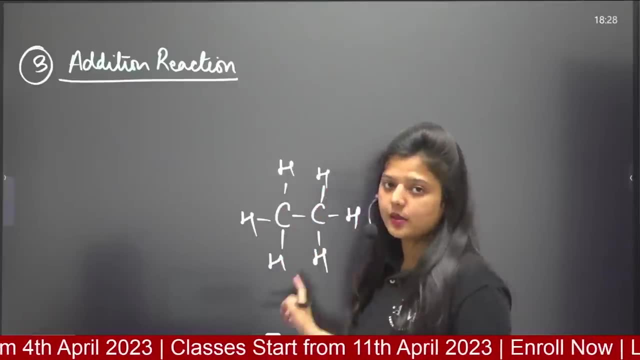 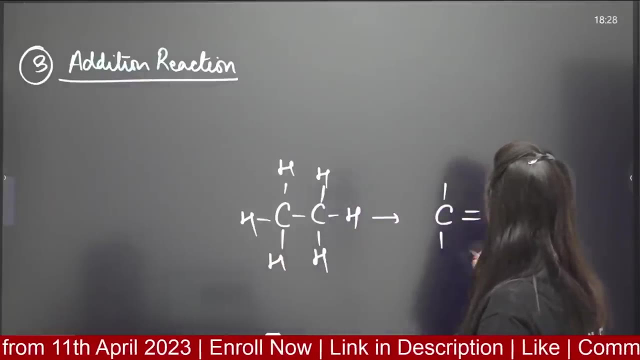 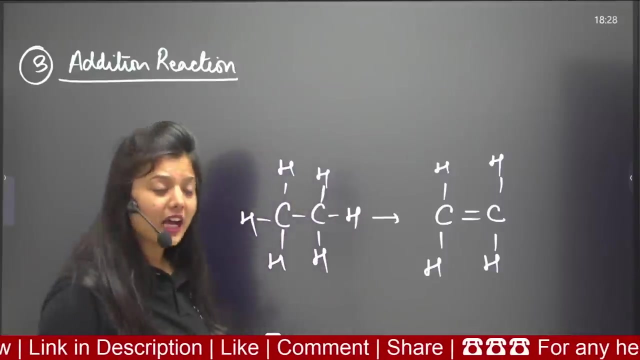 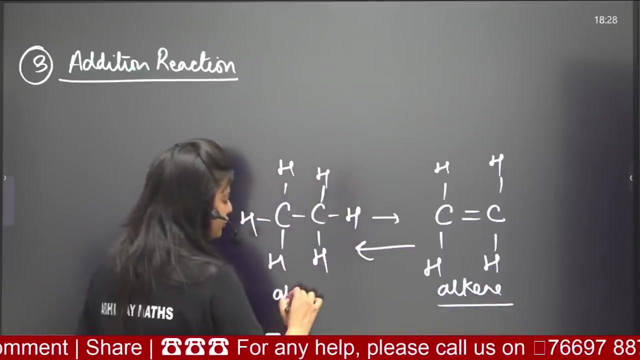 You are organic Heat's out. Michael is doing alone. This is a complete structure. all carbon bonds are fulfilled here. after this, if I tell you that I have an alkene in which a double bond has been applied and it has become this, it means that we have stolen some hydrogen from here. we have removed some hydrogen. is its reverse possible that I make an alkene from this alkene? 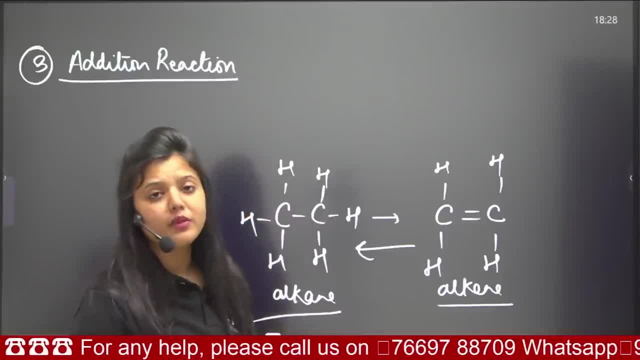 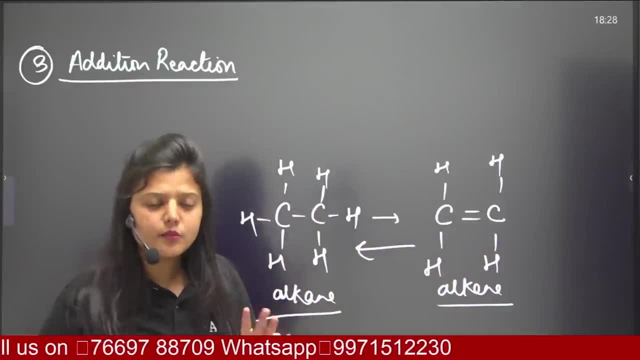 is it possible or not? you will say that, ma'am. it is absolutely possible. when I can apply a double bond by removing two hydrogen from here, then I can apply two hydrogen by removing double bond from there. is it simple or not? is it simple or not? tell me quickly once. 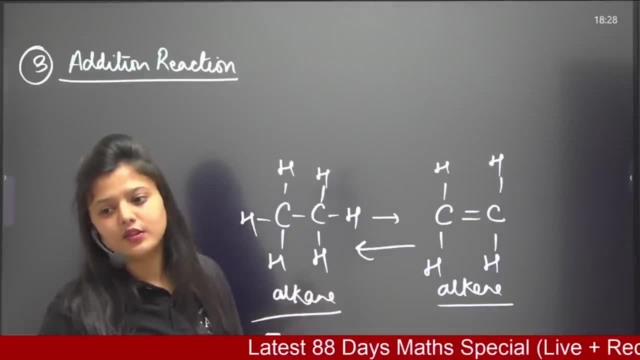 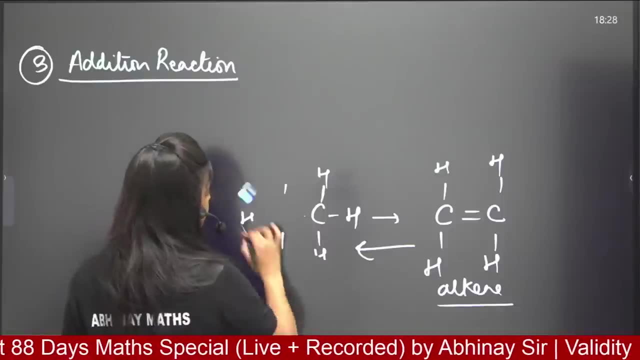 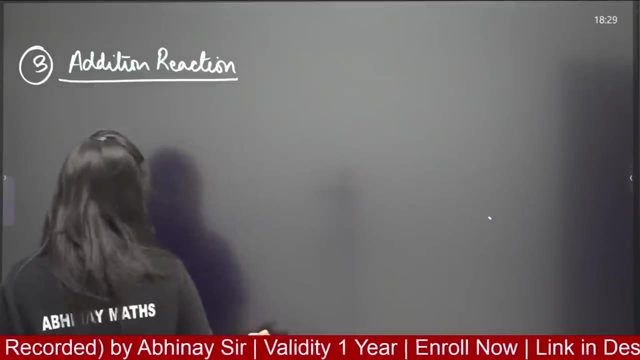 Prabhat class is live daily evening at 6 o'clock. class is live only. okay, it is still live. it means that whatever you have to do, ma'am, you have to disturb the class by doing anything, then that student will hide him and send him to a point where he will talk or keep him near it. now you can. Honda factory will not be able to do this. I need this particular teacher to come further through him. 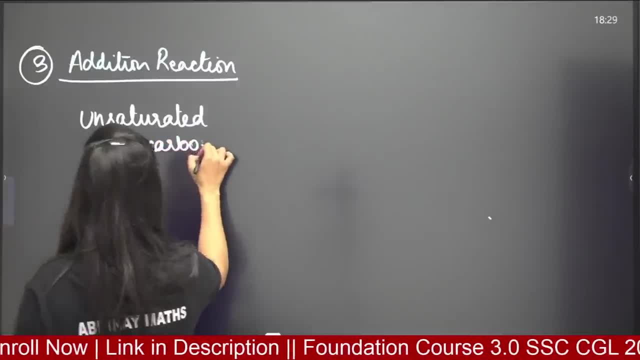 now what we will do. the same thing. location will come tolook inside the site, which means, if I talk to you, I have an alkene or unsaturated hydrocarbon. now, if I talk to you, I will make this unsaturated hydrocarbon. 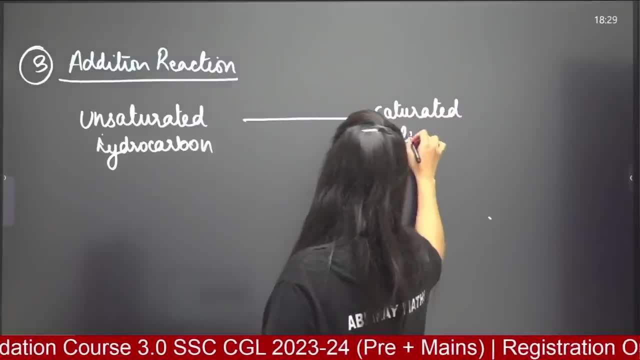 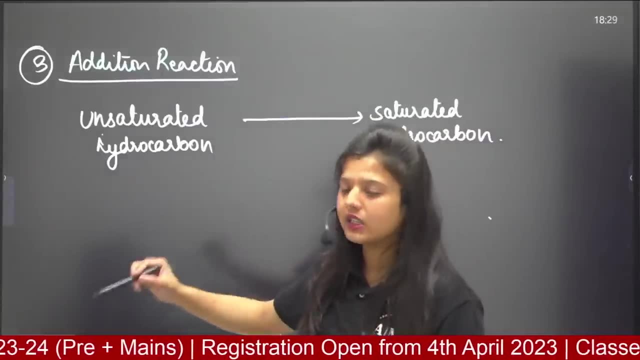 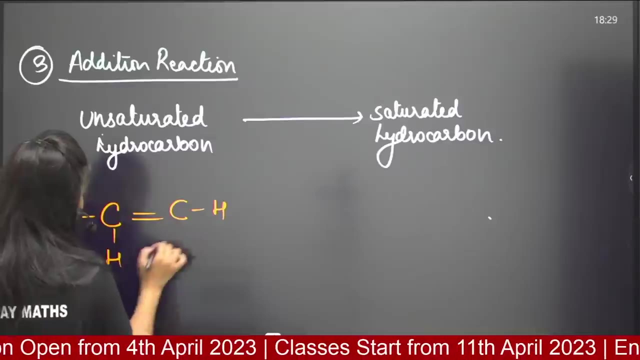 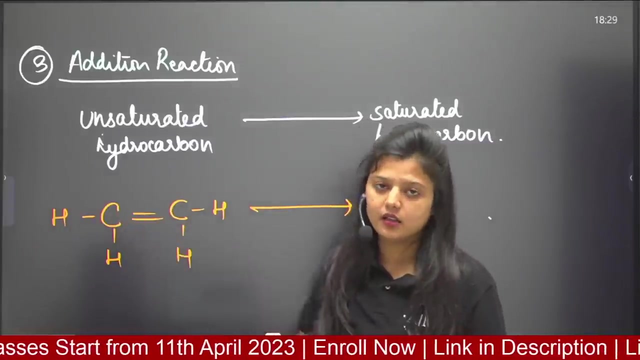 Now in unsaturated both can come. alkene can also come, alkyne can also come. I will need either one of the two to make an atom. suppose I took alkene here. you said that ma'am C, double bond, C here hydrogen, here hydrogen, here hydrogen and here hydrogen. what I did with it? I removed a double bond of it. this is a double bond. one bond basically tells the transfer of an electron here, correct? 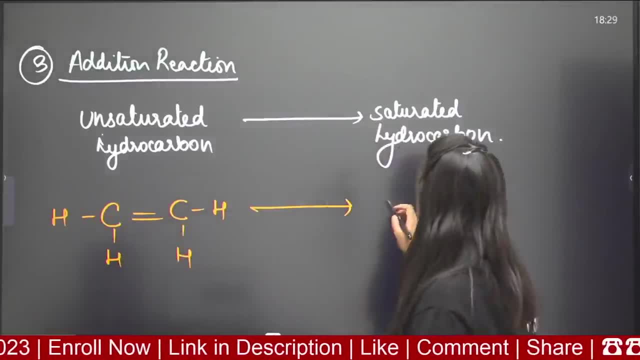 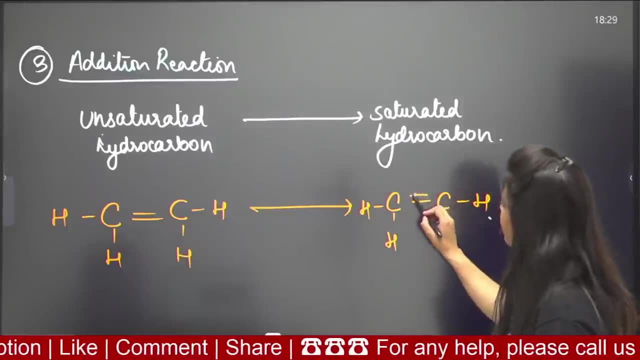 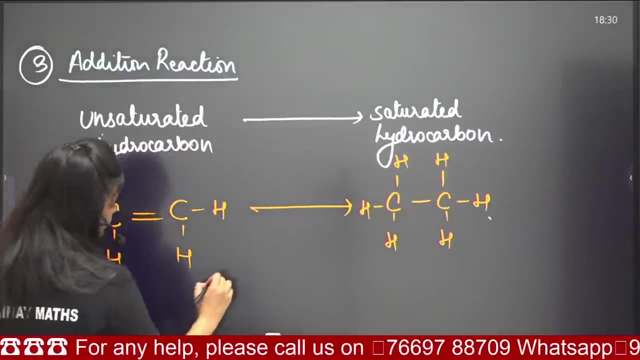 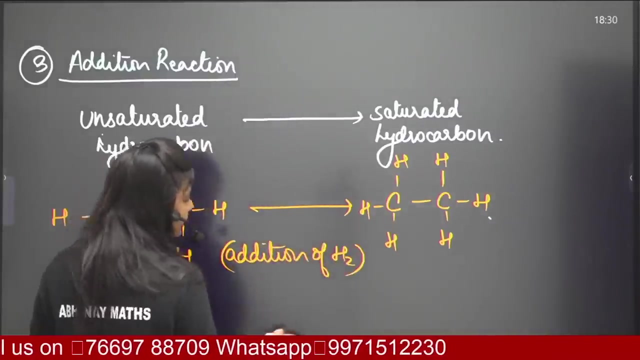 Now I removed a double bond. what did I make with this alkene? Here I made an alkene. what was the whole story? It was the same, just the double bond. here we removed it and returned both hydrogen. when, When we did addition of hydrogen, here we took two hydrogen and joined them. and with whom do they happen? 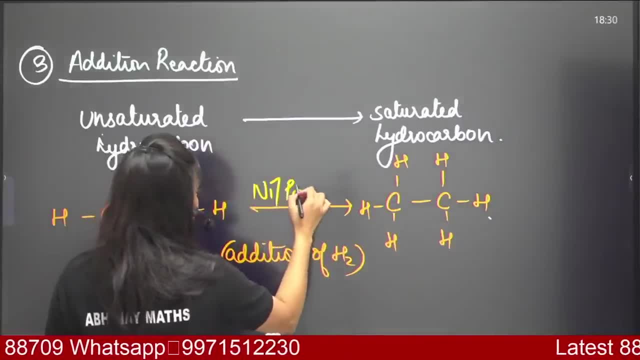 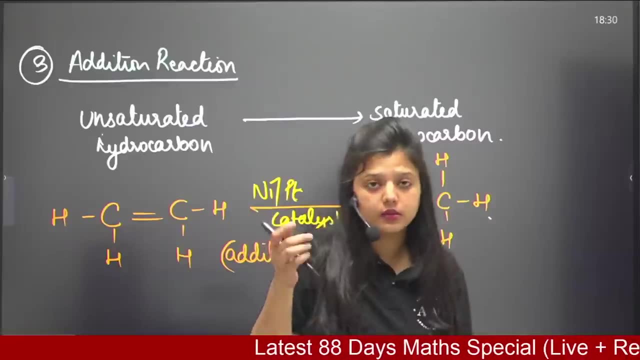 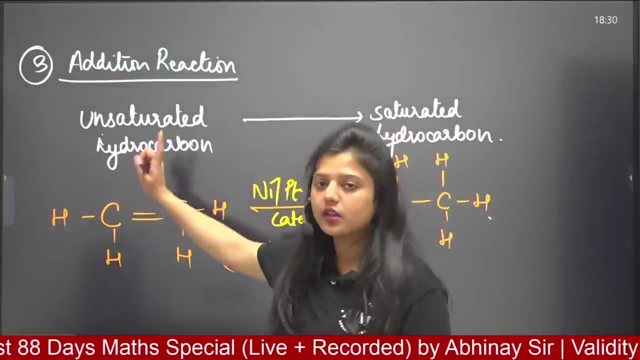 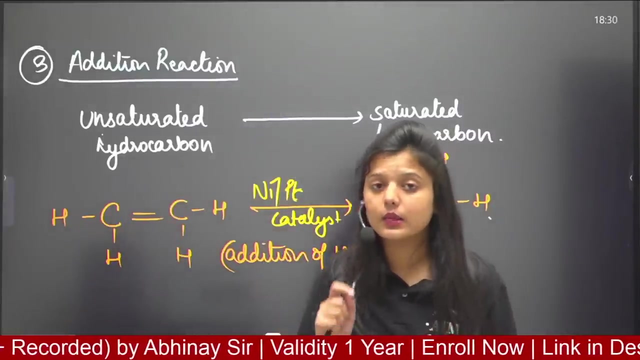 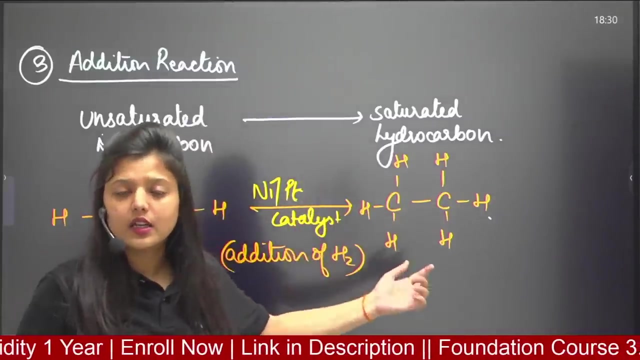 When we take nickel platinum as a catalyst. here, what happens? We are adding, we are using that is to make every reaction. it is very important for me to have one or the other enzyme a catalyst. okay, so what we did here- this was the alkene I took unsaturated with me in unsaturated, I removed the double bond and here we did what we added a hydrogen molecule, which means we did hydrogenation reaction. we have added hydrogen, call it addition, we are joining it ultimately, or if we are adding hydrogen, then what will be the specific reaction? 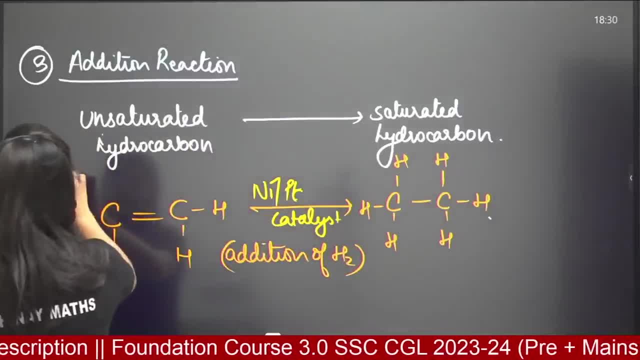 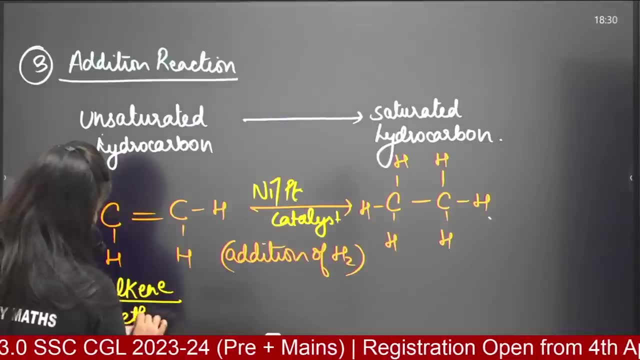 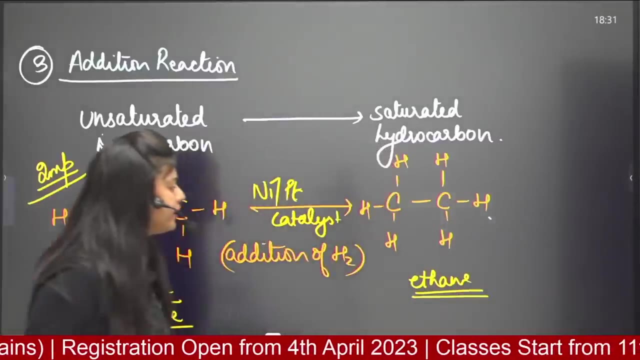 Reaction, and this reaction is very important. I repeat, I tell you once: pay attention and understand it. What is this? It is alkene. we will tell you its name. it is ethene. we have made this from ethene. we have made ethane. we have made an alkene from alkene. it has been made. 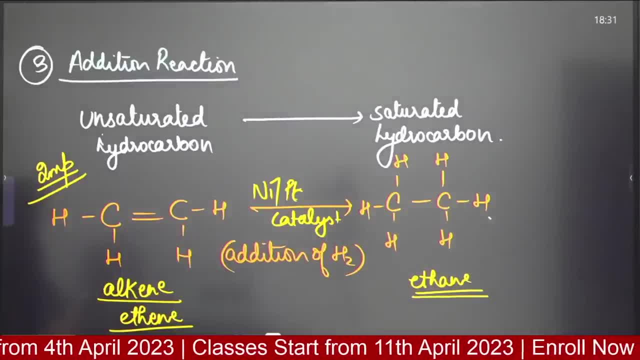 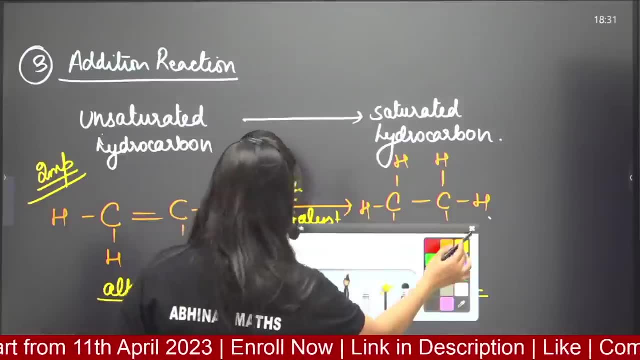 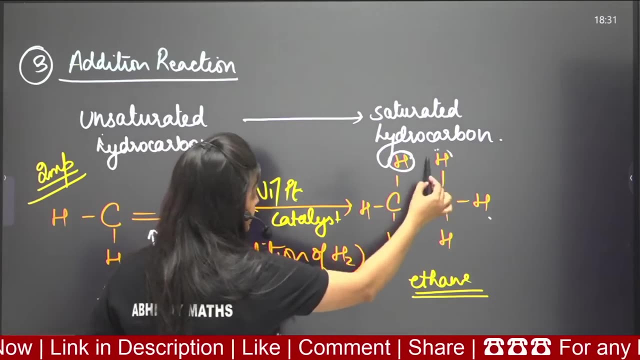 Please note it quickly. Alright, once you will note it here quickly. What do you call this? This is lithium. This is lithium. This is potassium. This is hydrogen. This is lithium. This hydrogen went and added here and when it was added here, its bond was removed and these two hydrogen came here and hung here. 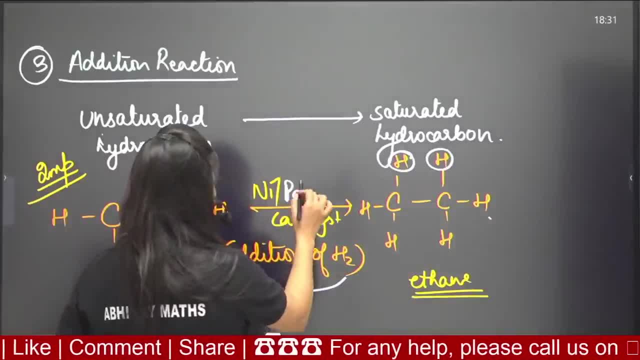 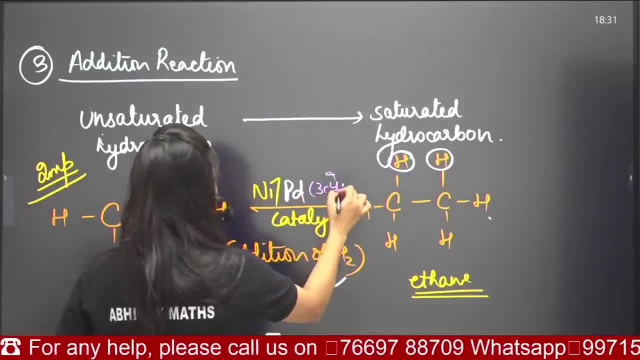 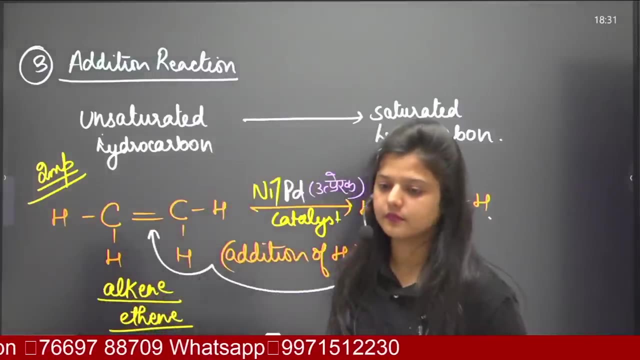 Here, nickel and palladium are working as a catalyst. Okay, how are they working? Ut prerak means like a catalyst. Okay now, if you are done with Ram Ram, Good Evening Pradham, then please write Quickly once. 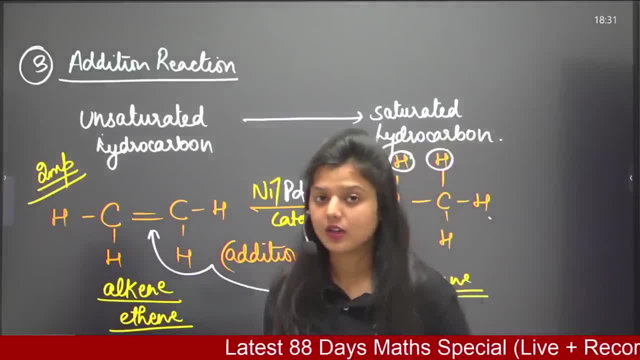 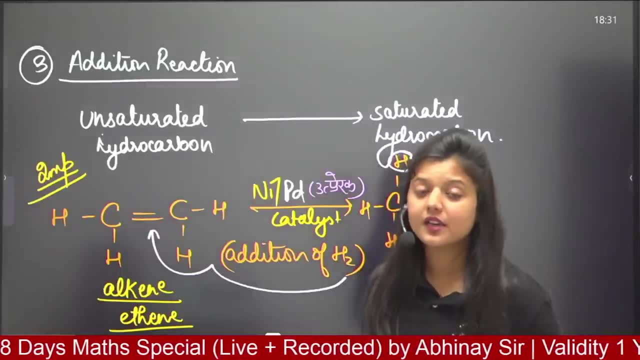 In life. the struggle was everyone's and will remain. There is no fun in living a life without struggle. You think that you don't have to work hard, you don't have to write, you don't have to revise, Just yes, let's study once and go for the exam. 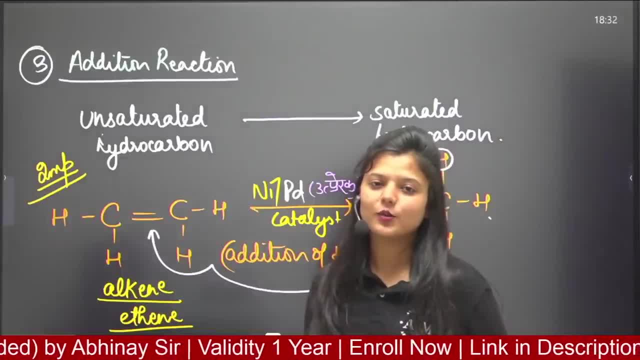 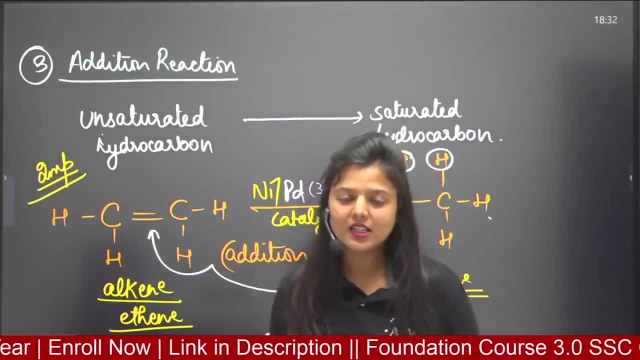 Without effort, without hard work, without struggle. if in life everything can be achieved, then today, by working hard, so many people are struggling. what is the need for all this? Everyone wants to press one button and all our work will be done here in a single click. 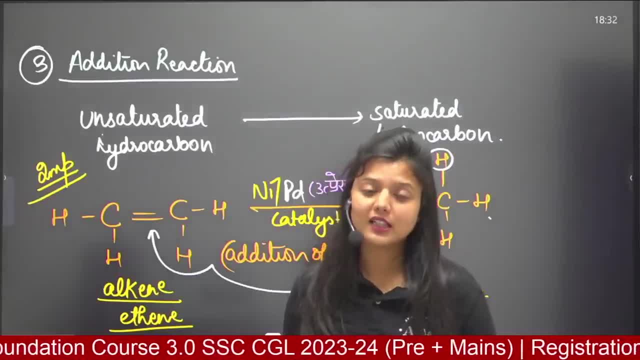 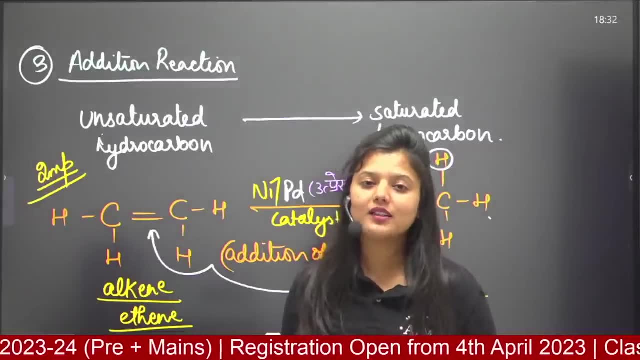 But it is not possible. you have to work hard for everything. But there are also ways of hard work. One is smart and the other is hard work. Now, what way do you choose from these? If it is about hard work, then Lord Ram did it, Krishna also did it, everyone has done it. 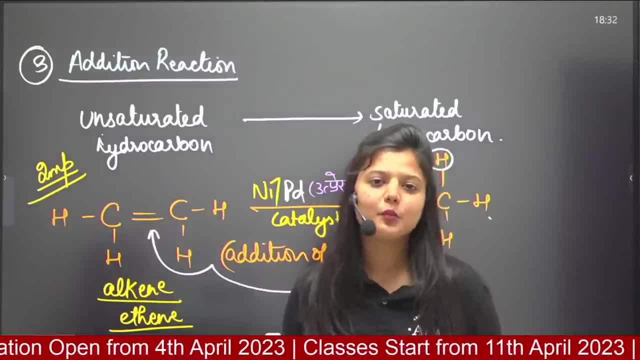 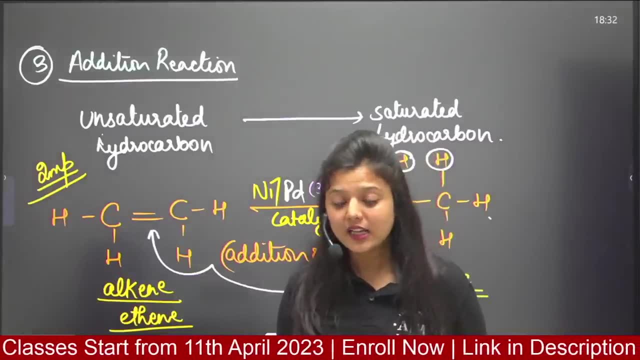 Then, brother, you will also have to do it, But the way is yours. How will you choose? This is on you. Until there is no failure, no difficulties, no obstacles on the way, then a monotonous life is going on, ma'am. 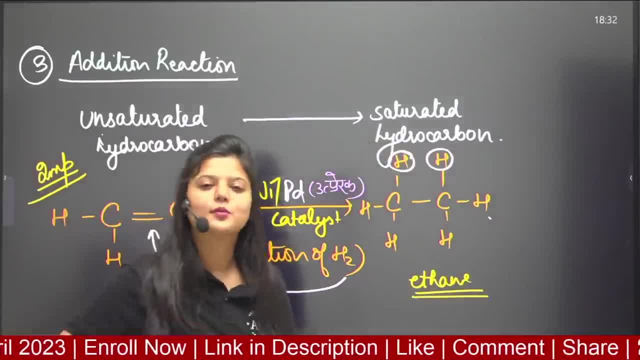 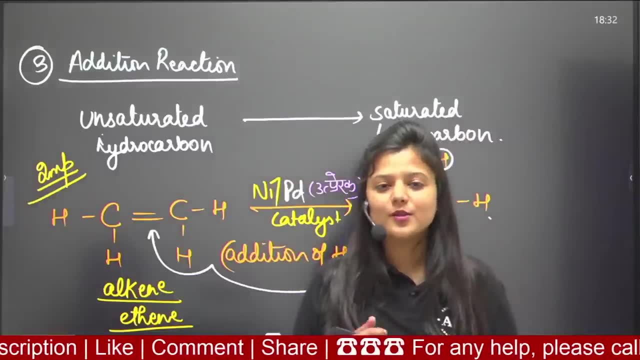 Then what is the problem? Then we will live, we will cut On one way. everyone can walk. Even if someone does not have knowledge, he can walk on one way with his eyes closed. It is fun when you have to use your intellect, use your brain. 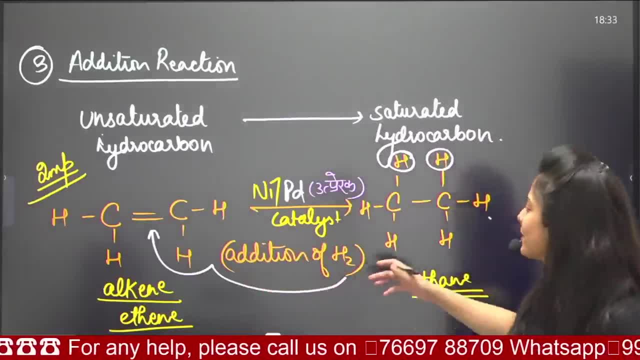 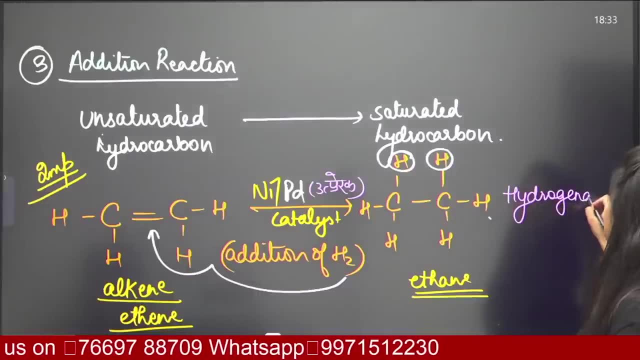 That is why you have to write, you have to do revision of all these things. We give it a name. What do we call such processes? Hydrogenation reaction. We are understanding by name Hydrogen's addition. Hydrogenation reaction. 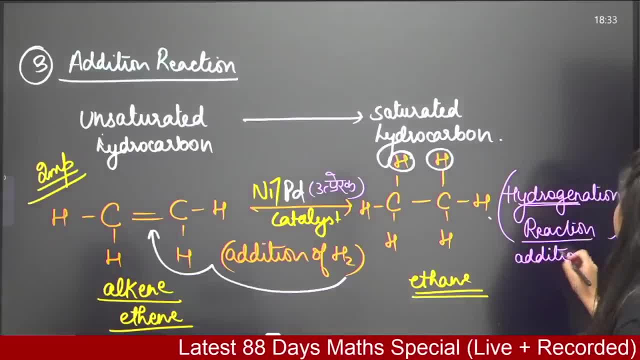 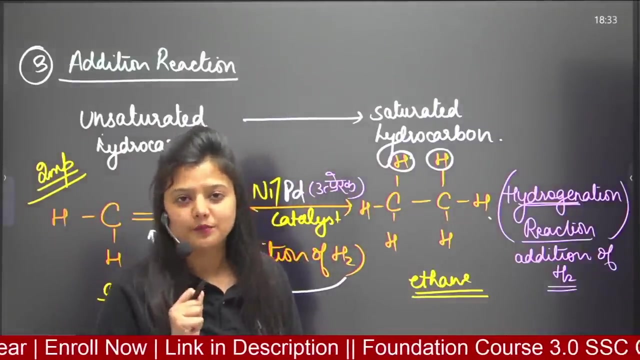 Addition of hydrogen. Did anyone face any problem in it? Addition of hydrogen is called here. If you talk in daily life, then have you seen any example of it here? Yes, brother, Have you seen any example of hydrogenation here? Ma'am see one thing. 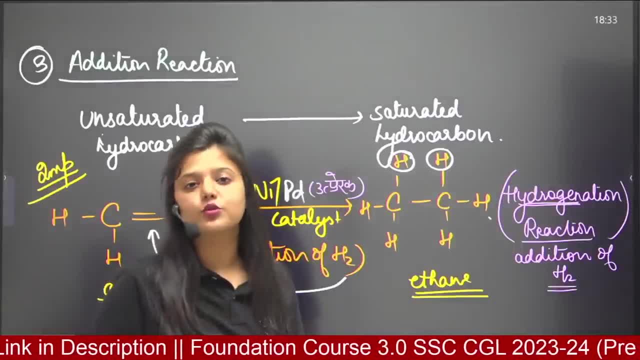 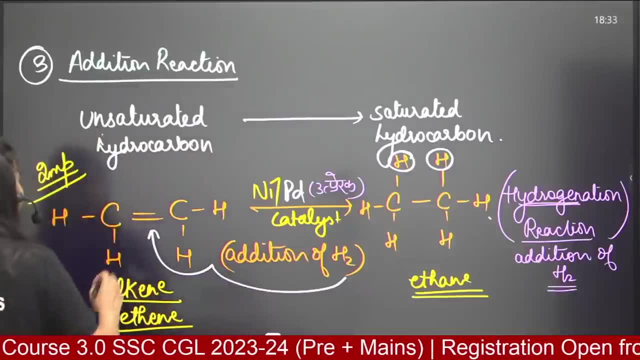 The oil we use in our homes and the ghee we use. If I want to make ghee from oil, it can be made. If I want to make ghee from oil, it can be made. That is, in unsaturated hydrocarbon we can keep vegetable oil. 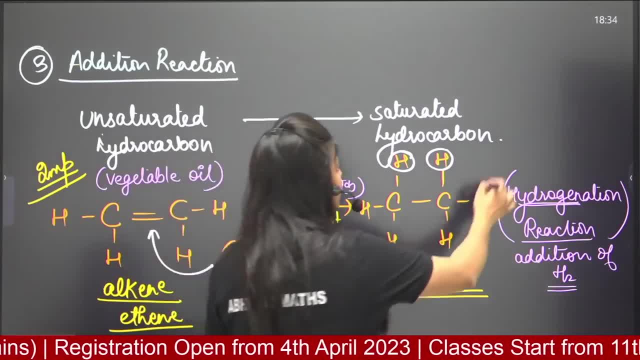 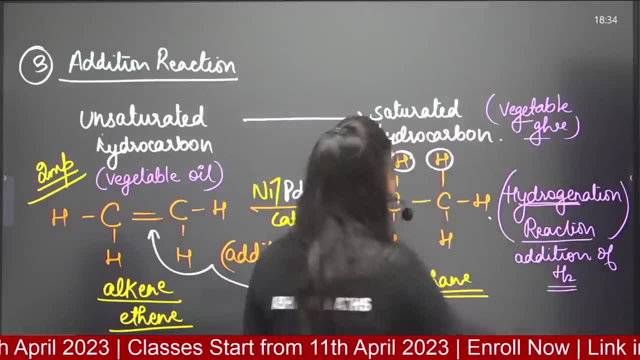 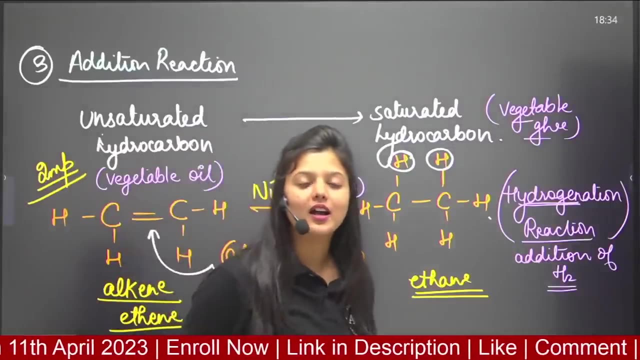 And what can we make with this vegetable oil? Vegetable ghee can be made Vegetable ghee. This question was asked that if you make ghee from oil, then which reaction will be seen here? So you can say that there is a hydrogenation reaction happening there? 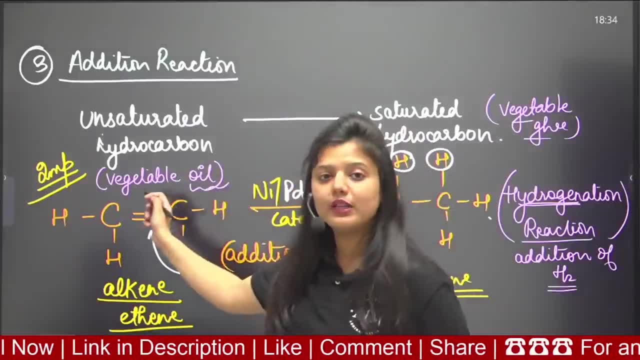 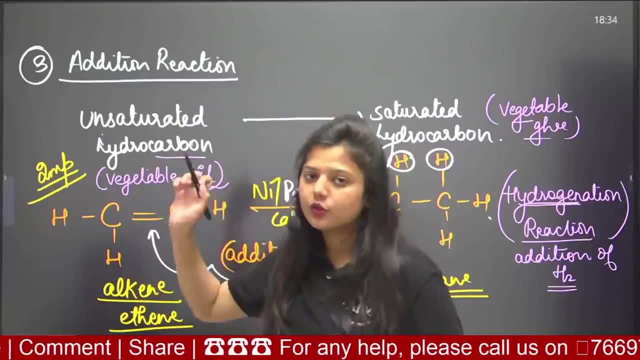 When we talk about oil, then oil also comes in polyunsaturated hydrocarbon. It comes in unsaturated hydrocarbon. Actually. look here there is hydrocarbon Here. we are using the word unsaturated hydrocarbon Because we are taking alkene and alkyne. 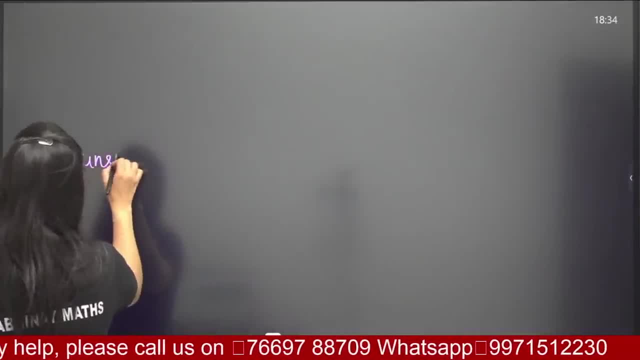 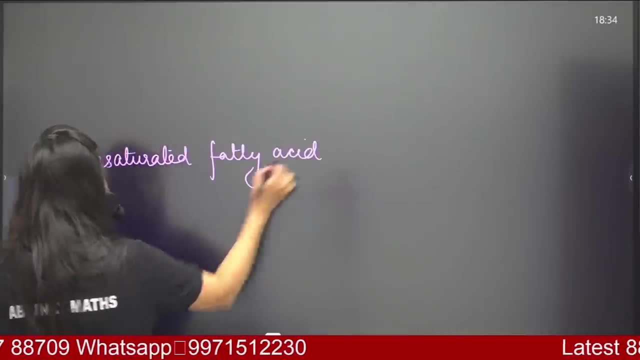 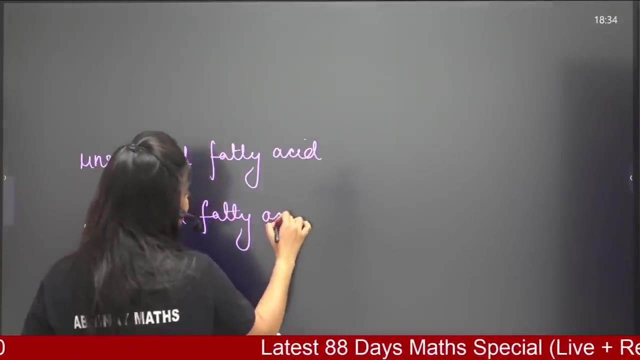 If I tell you that any fat is also seen as unsaturated fatty acid and saturated fatty acid, That means the chain that will be attached here is the chain of our fatty acids, What It is, the chain of the amino acid. So there are two different types. 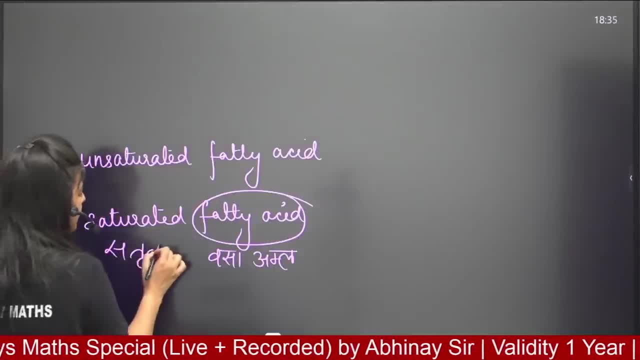 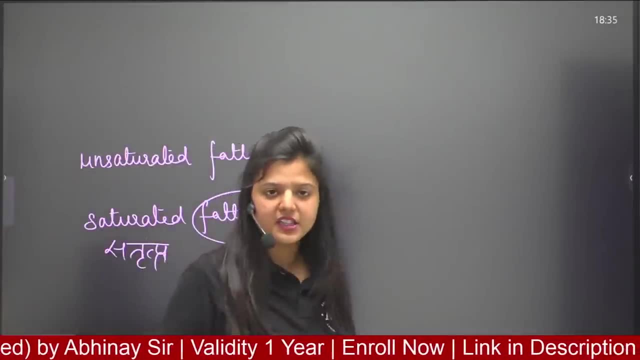 The point is that this one is saturated and the other one is unsaturated. The point is that this one is saturated and the other one is unsaturated. The point is that this one is saturated and the other one is unsaturated. You must have heard in the advertisement that what is good for your heart. 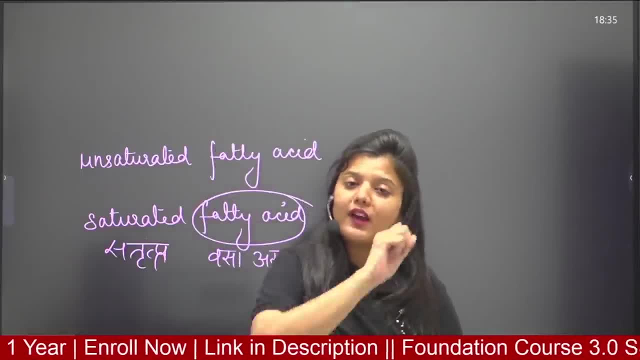 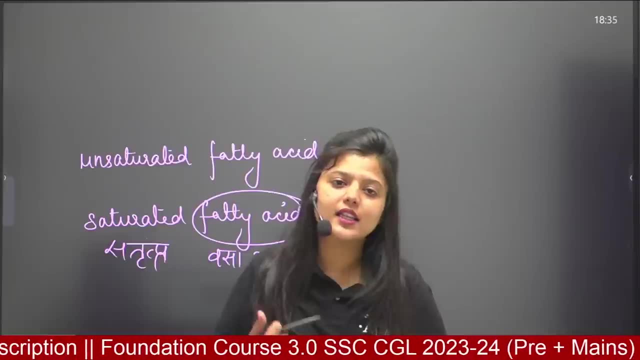 What is it? Poofa Mufa? you must have heard such names. We had also read fat. We had also told you that when it comes to this poofa mufa, then what oil, ghee, is good for your food, for your body? 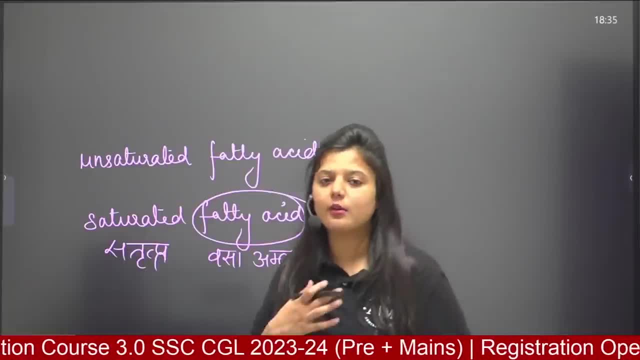 What should you eat? Pure desi ghee. people eat and say that our health will be fine. If you eat desi ghee in winters, then it will be a problem. You are eating oil in summers. You are eating desi ghee in summers. 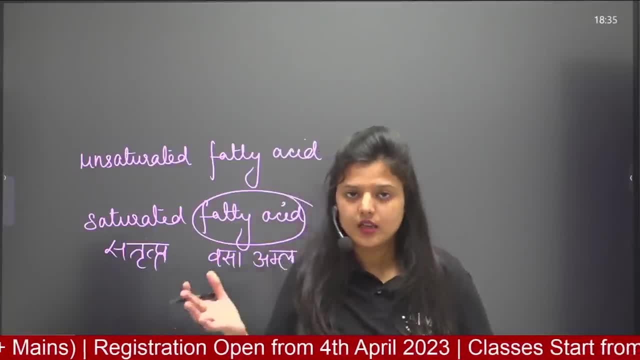 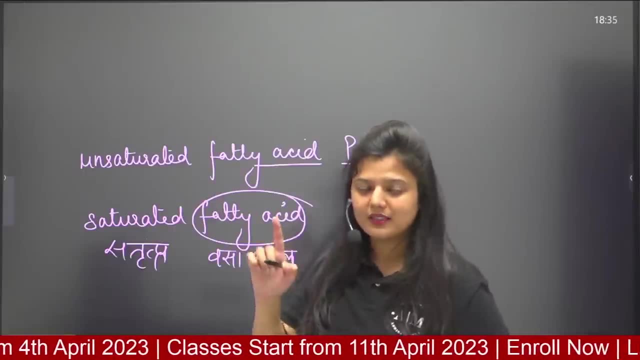 If you are eating desi ghee in summers, then you may not have that much problem. The point is that all these polyunsaturated fatty acids are called poofa. You have read about refined dalda ghee. If you have seen the ingredients on the packet of all these, 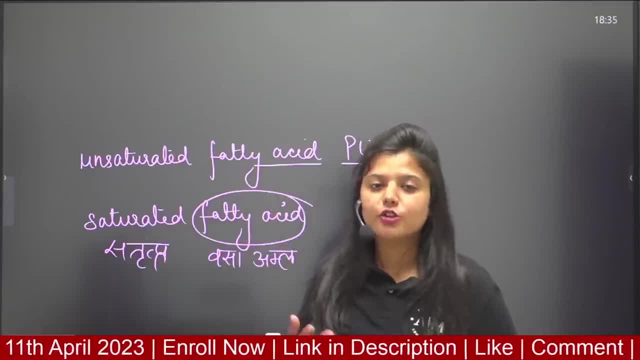 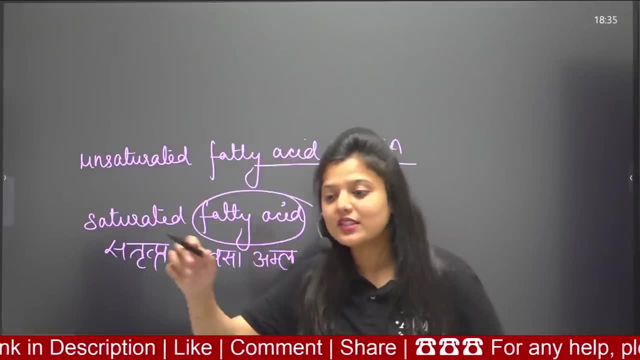 then, what is here? What are we eating, after all? Why are people having such a heart attack? Why is the cholesterol increasing in people? What is the reason for this cholesterol? Have you ever wanted to know that? which oil, which ghee should we eat? 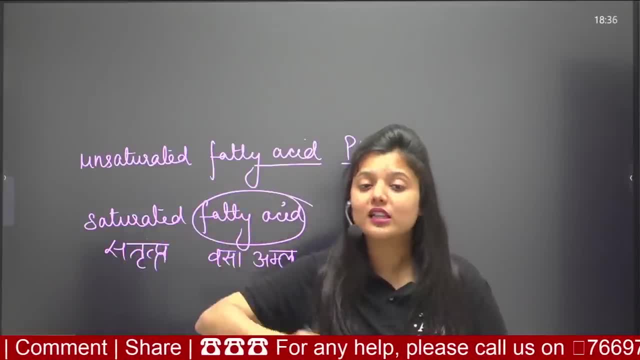 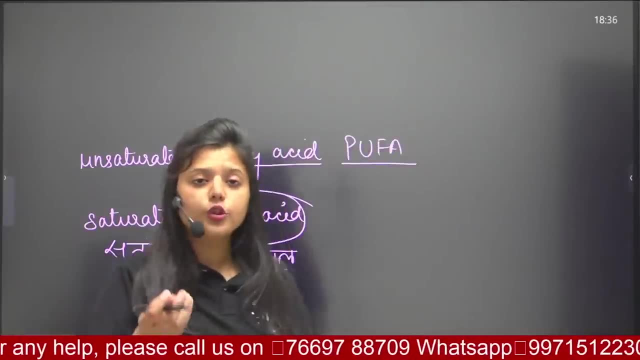 Dalda goes into refined, But it is the most harmful for your health. If you can eat any oil- that means any oil in which you can make vegetables- then our unsaturated fatty acids come in it. Talk about poofa. talk about moofa. 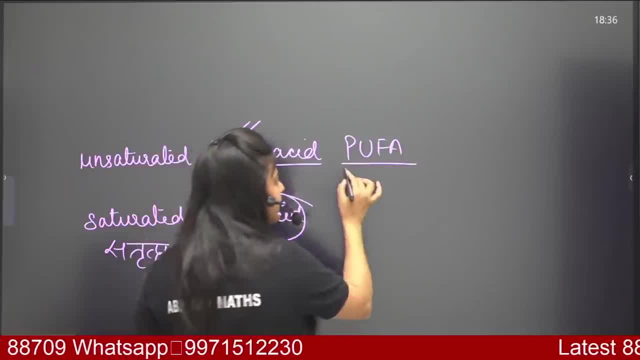 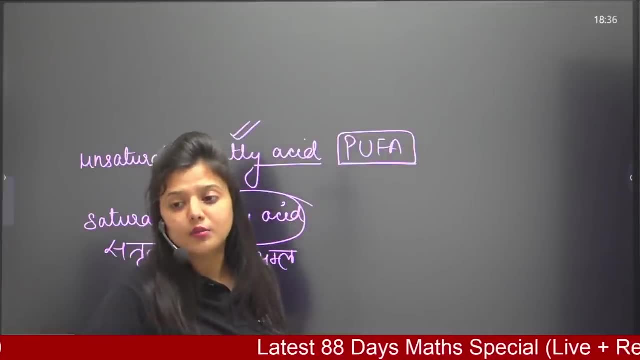 In fact, if you look inside them, then the chain is our own chain. Fat is always there. Fat is in everything: It is in milk, it is in ghee, it is in oil, it is in butter. The point is that whose chain is so long and it will take the same time to break it. 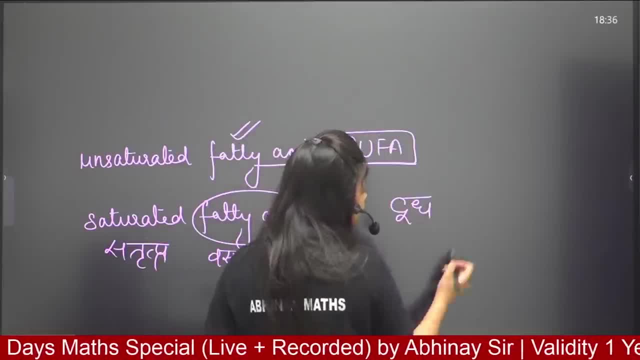 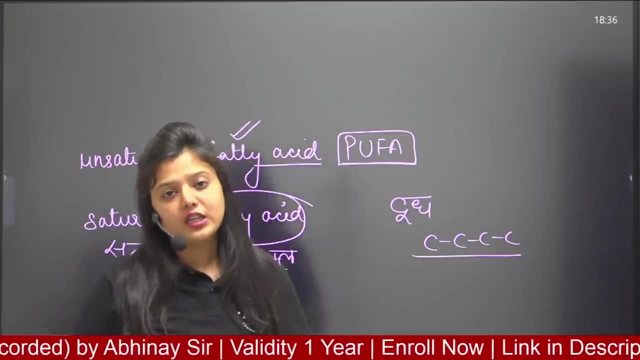 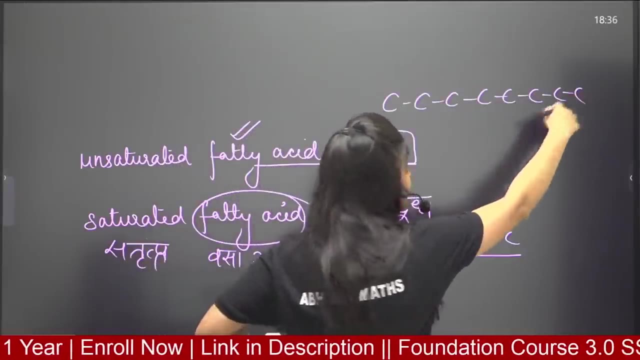 But if you talk about milk, then the chain of carbon in milk looks like 3 to 4 carbon. Now tell me one thing: on one side I have a chain which has 3 to 4 carbons and on the other side I am bringing a chain from 1 to about 17,, 18 or 20 long chains. 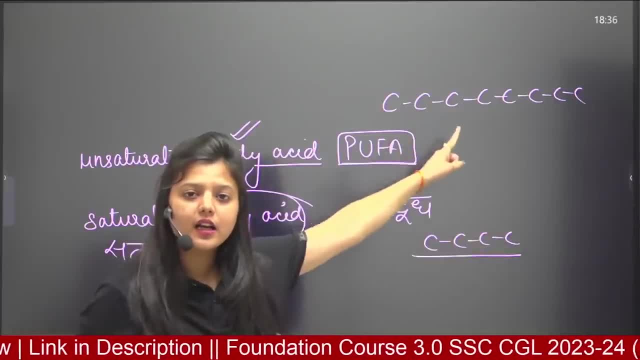 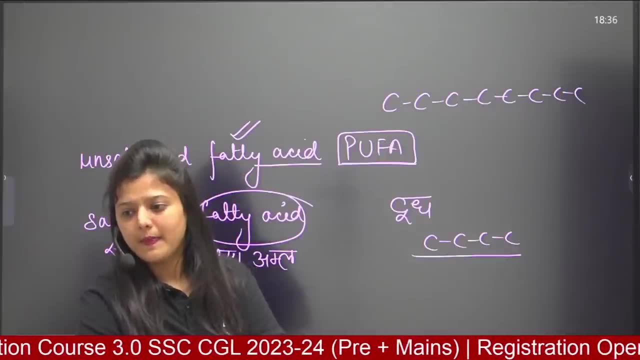 So we ate both things in the body. On one side we ate oil, we ate refined, on the other side we drank milk. Who will take more time to break? Who will the body digest quickly? Tell me quickly once. Yes, brother. 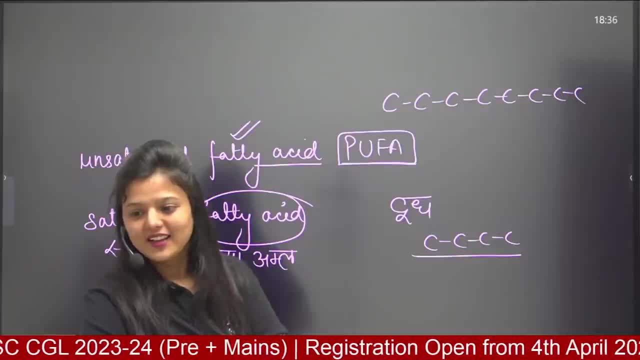 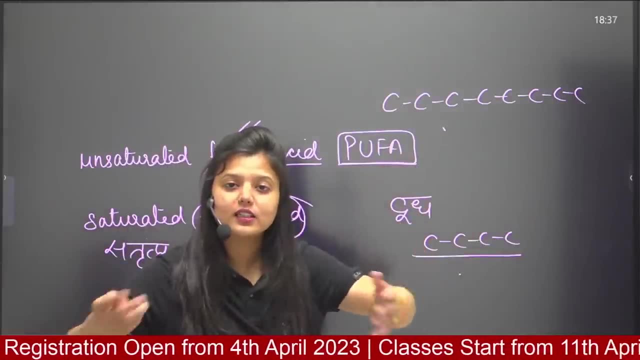 Yes, brother, Now no one eats dalda well, So who will take more time to break? It will take less time to break this. it will take more time to break this. The longer the chain is, the more energy it will have to give. 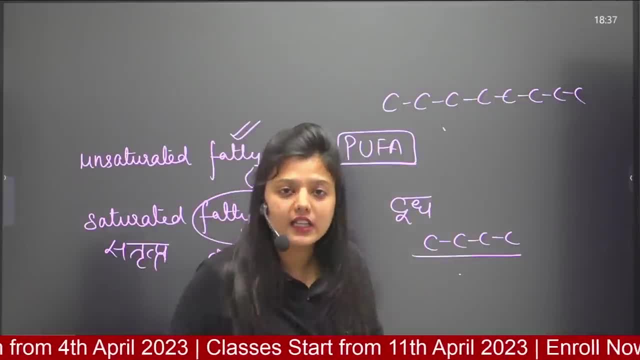 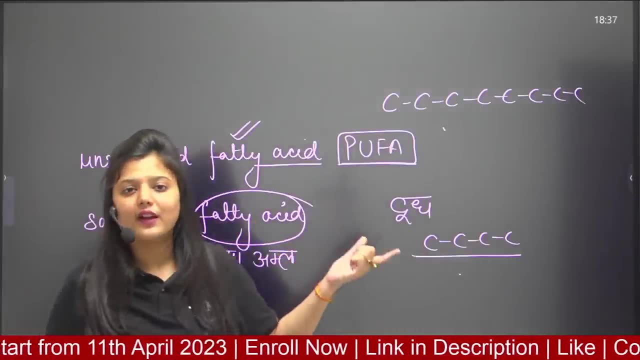 Your body will have to work as much to break it. So that is why it is said that, sir, what you are eating, see what is in it. Actually, all these unsaturated fatty acids are said to be good for your health, Because if I talk about them, then somewhere. 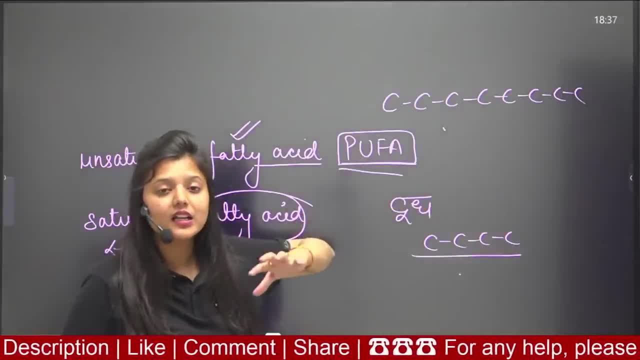 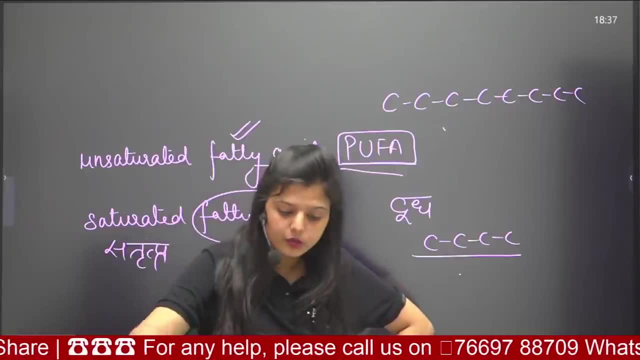 which we use mustard oil, not refined dalda, which we are using mustard oil somewhere. it is considered healthy for our body. If you have to do an experiment, then see the boxes of oil ghee at your home, which box will easily remove all its oil when washed with water? 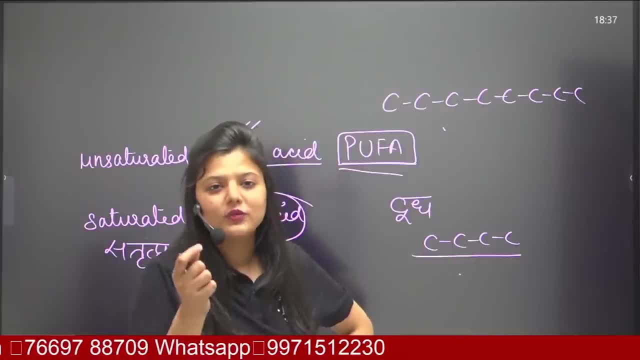 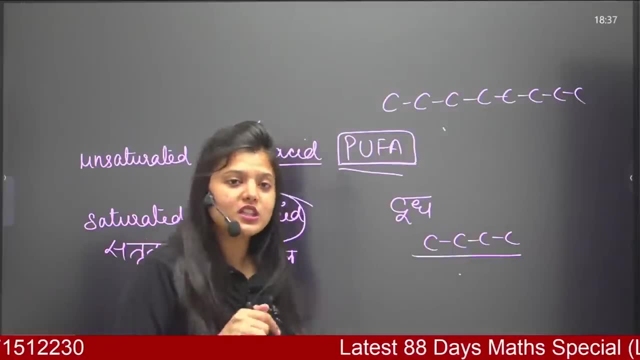 If you have a refined box, you will not try to remove oil from it until you heat it. And this is the reason that when the same oil goes into our body, goes into our lungs, you say, ma'am, I have eaten a deep-fried potato tikki full of oil. 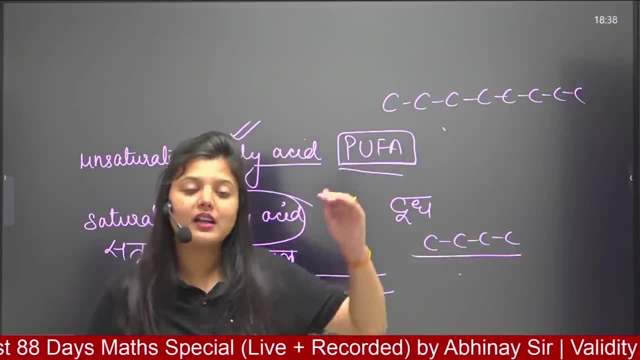 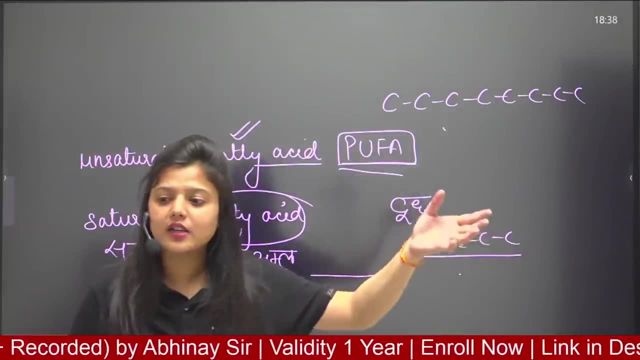 And after that, my cholesterol level is increasing, my triglycerides are increasing. You have consumed fat, right, All your fat will go into it and it will get stuck. It is not moving away from the boxes kept in your house, So how will it move away from here, ma'am? 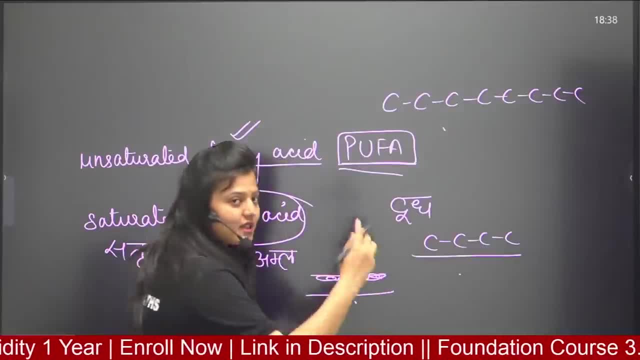 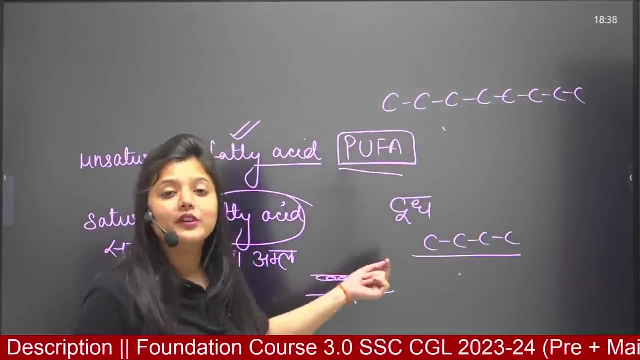 It sticks here Now as people do in Japan. brother, what are you drinking on it? You are drinking hot water, You are consuming hot things. you are drinking tea or coffee. it makes a lot of difference. But what will we do after eating pizza, burger, potato tikki? 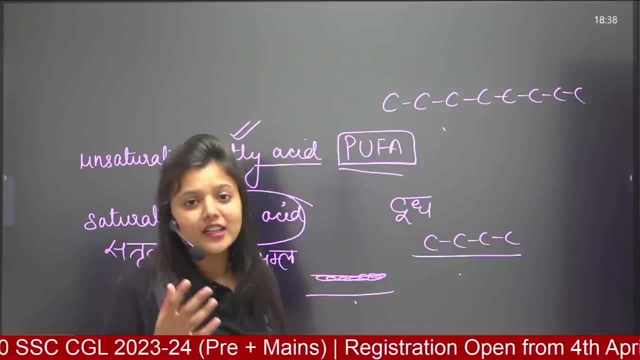 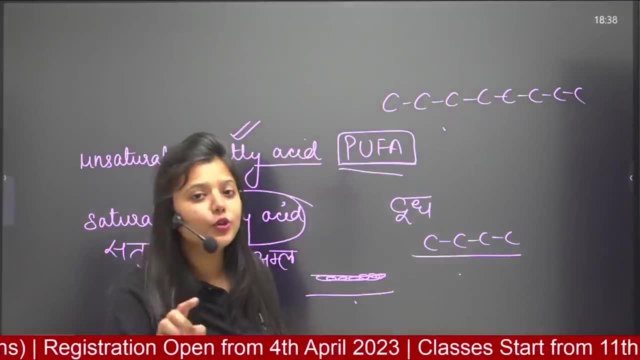 Ma'am, we consume more cold. drink on it. Bring it cold, completely chilled brother, Even if it is not a little hot, And when it goes inside it gets stuck more. Then what happens to this oil in your lungs? It gets stuck completely. 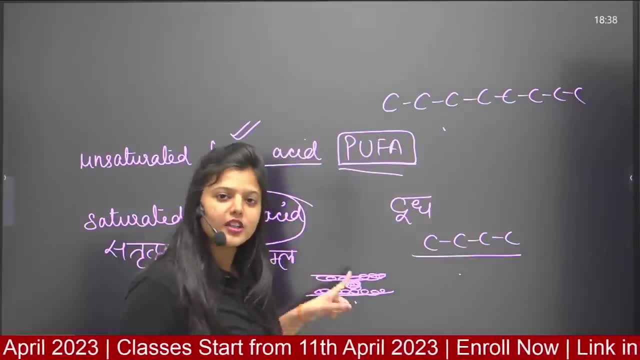 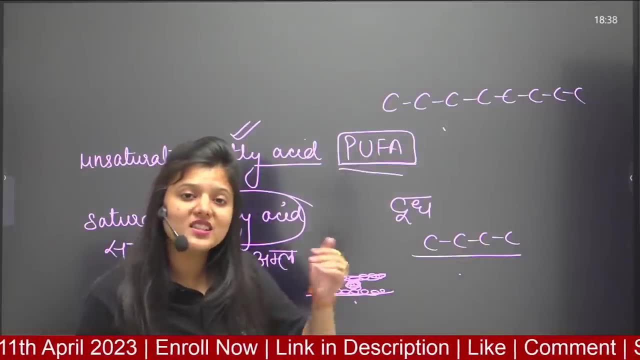 And slowly, potato tikkis are made here in the lungs and make this heart attack. This causes all the problems of your heart. So ultimately, remember that all these things are for your health. All these things are harmful for your body. All the saturated ones are the same. 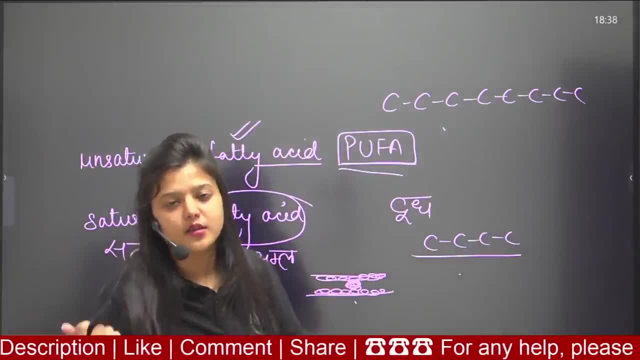 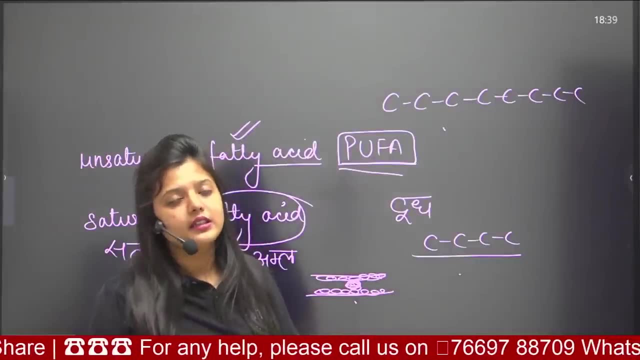 Even when saturated, the animal fat that we talk about is considered so harmful for our body. But if you are talking about poofa, which is polyunsaturated, you can consume it, But that's the thing. We will have more harm to anyone at a higher level. 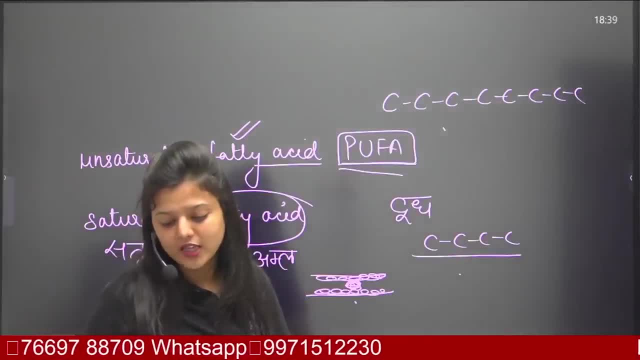 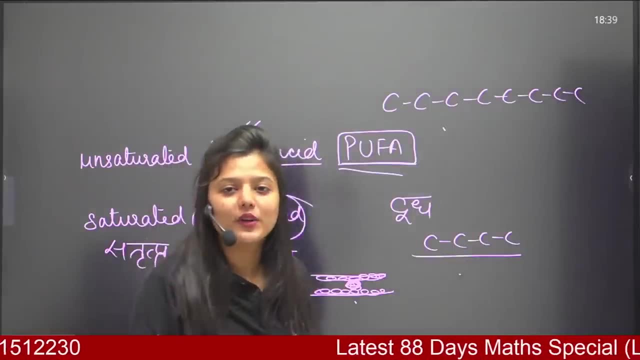 Okay, What is more high level for us? for everything Harm is said here, Is everyone clear. So, brother, What will you eat from now? This is up to you. You are very smart. You have to eat poofa. 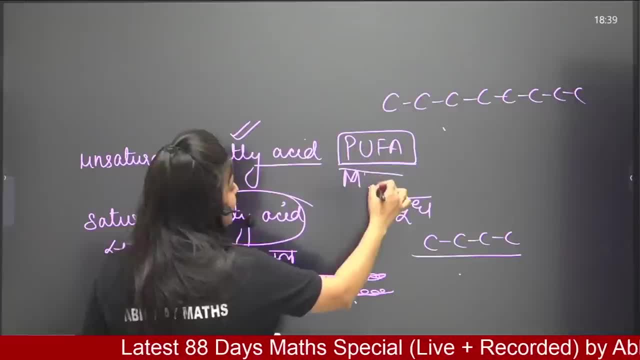 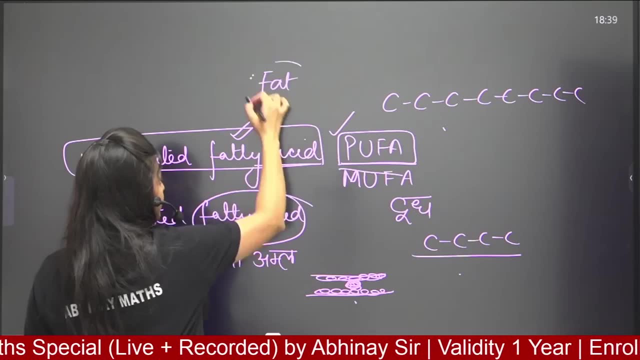 You have to eat moofa. Okay, This is mono unsaturated fatty acid, This is polyunsaturated And this unsaturated animal fat. When we were reading the topic of fat, when we covered biology, we read it in great depth. 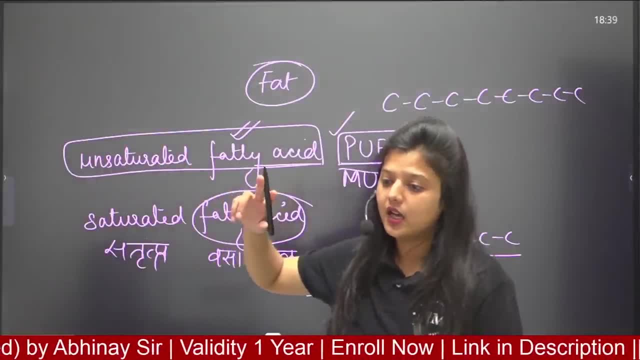 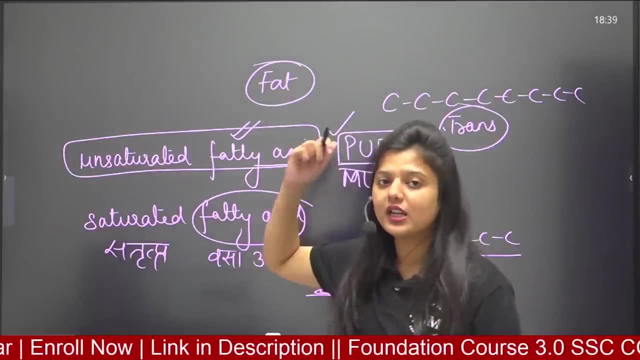 It also contains a trans fatty acid. Remember, Trans fatty acid is the most dangerous. All the pizza, burger and deep-fried fruits you eat. it contains trans And trans. Any Talk about its cake, Talk about cream? It is found in all of these. 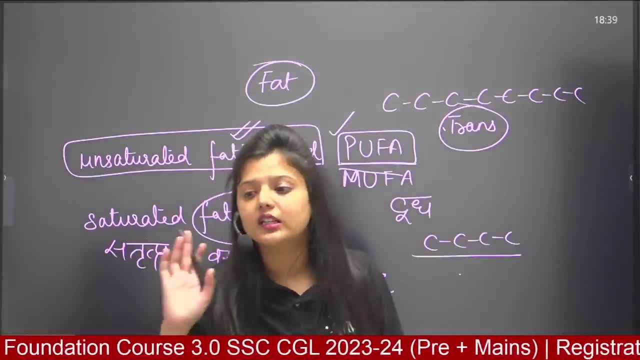 And it is not harmful, It is the most harmful. But what can the youth of today do? Can't improve, Can't agree That, ma'am? how to control this tongue? Can you understand the matter? Okay, Look, ma'am. 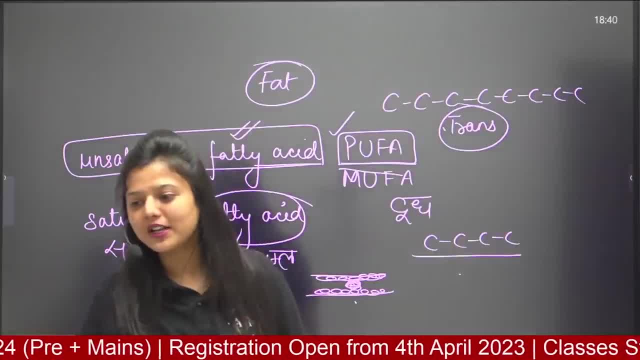 You have cold drink, You have cold water. You are alert to all these things. You drink A little. What is its limit? What is its quantity? Keep that quantity in mind. Drink, Not that ma'am wakes up every morning and evening. 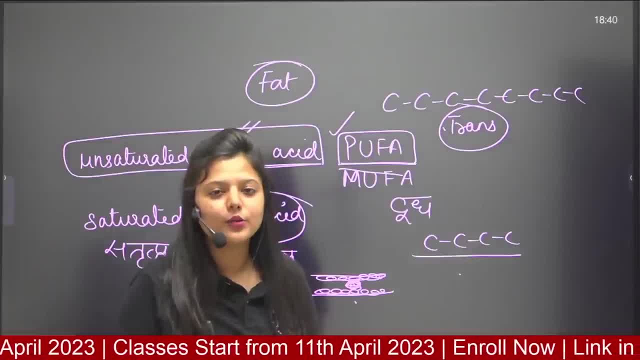 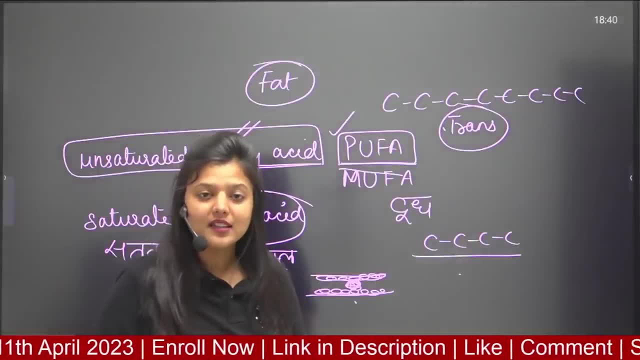 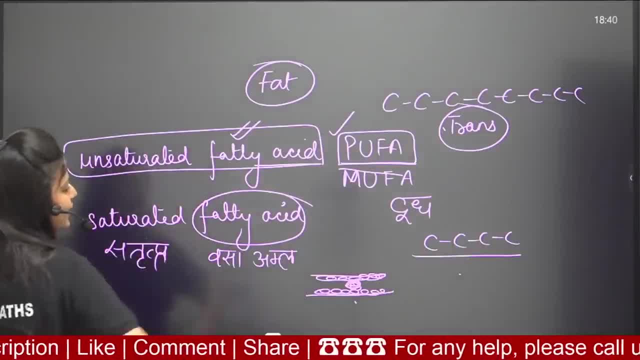 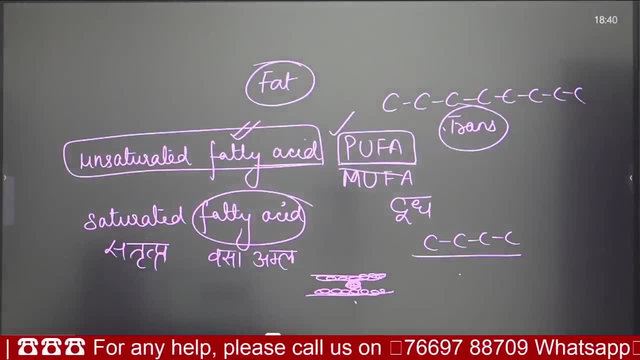 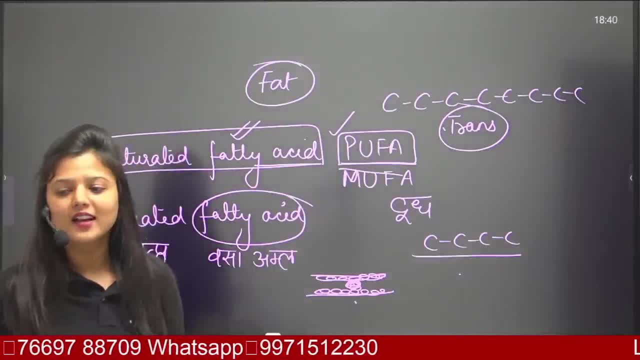 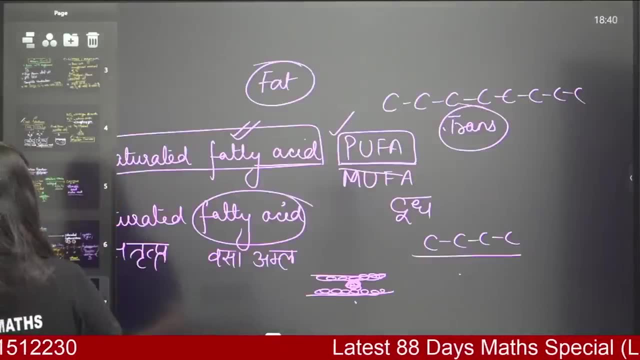 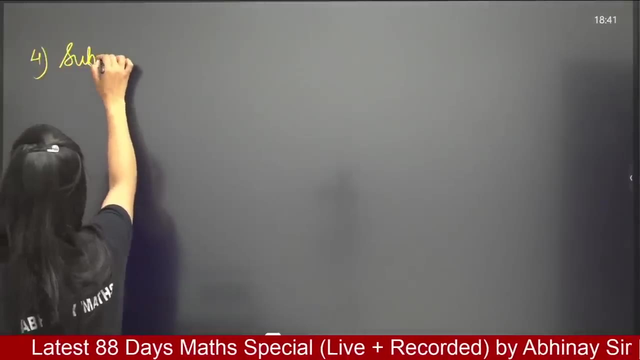 Idiot, Idiot, Idiotic, Idiotic, Adi Adi. Now, after this, we have read 2-3 reactions here. we talked about oxidation and then we talked about addition. Now let's talk about substitution reaction. We will put the fourth number of substitution reaction. 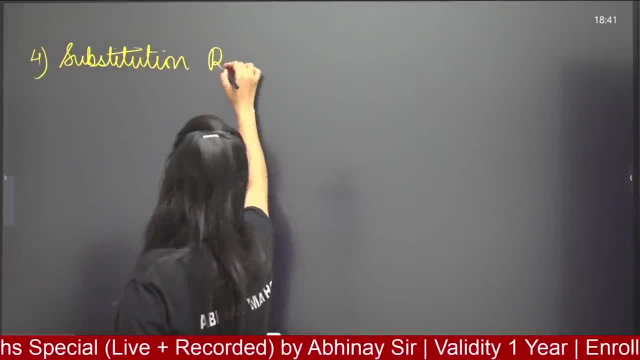 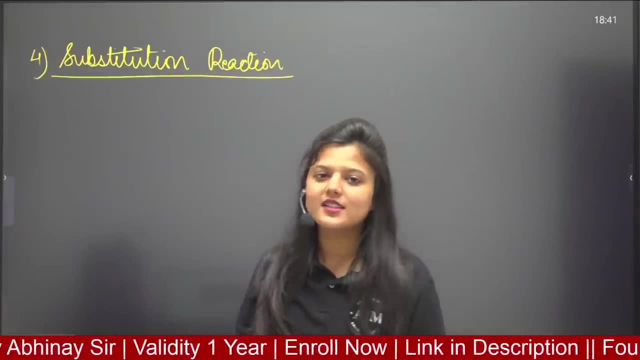 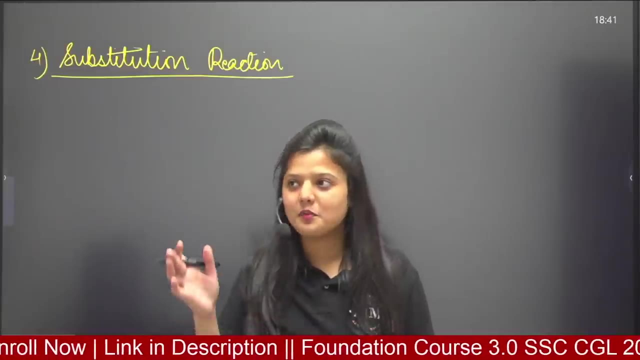 Substitution. Substitution means substitution. I told you an example: The one who has more power in life, he will easily come and displace it. The same power is more. the job is good. the money is good. It is said that these things are very high these days. 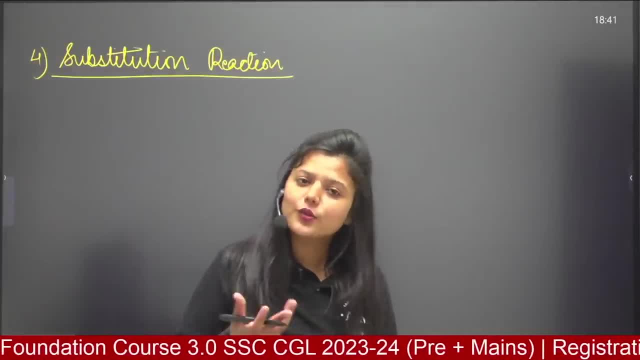 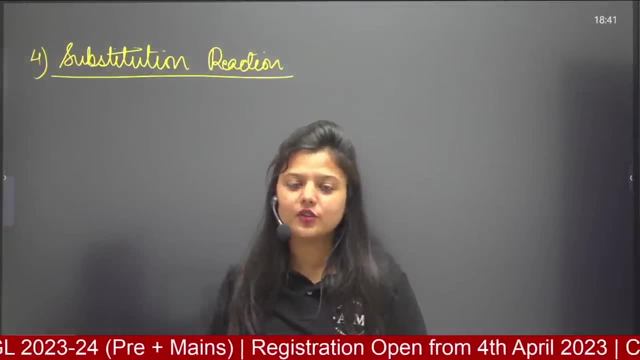 The one who has power. he is the one who speaks in the world. So the same story will be seen everywhere. In chemistry, if I talk about atoms and atoms, then it is established The one who has high reactivity. he goes and reacts. 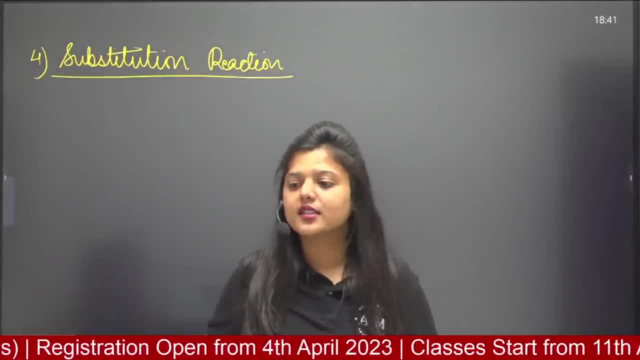 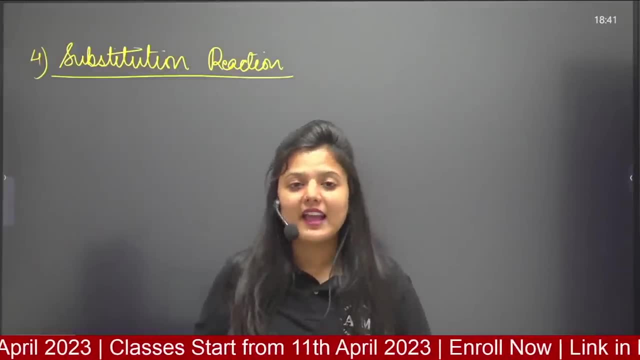 And what does the one with low reactivity do? He says that, brother, you move aside a little, Your here, It doesn't mean anything, Your here, doesn't mean anything. This is how it happens in our organic compounds. Now tell me one thing: I had methane. 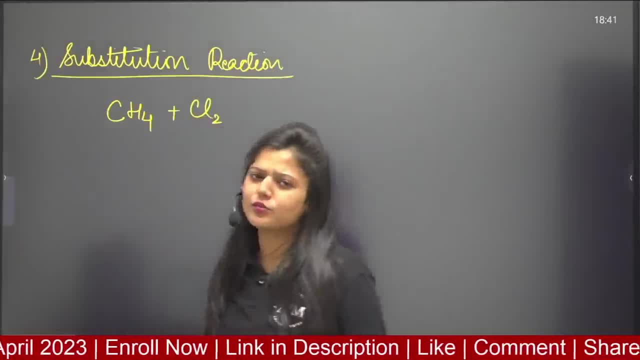 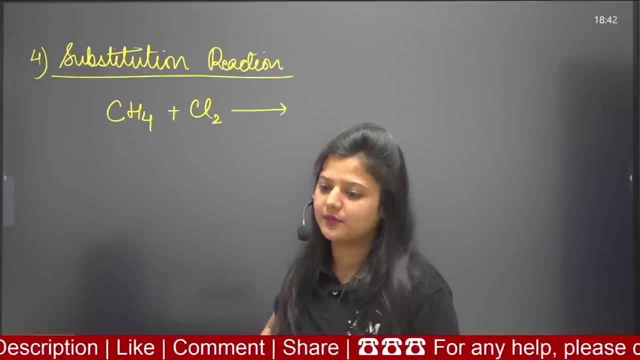 Now I have reacted methane with chlorine. Just tell me understand- and what will be the answer to this- That if these two will have a reaction, then who will substitute this? Who can reach whom? Okay, let me tell you one thing. 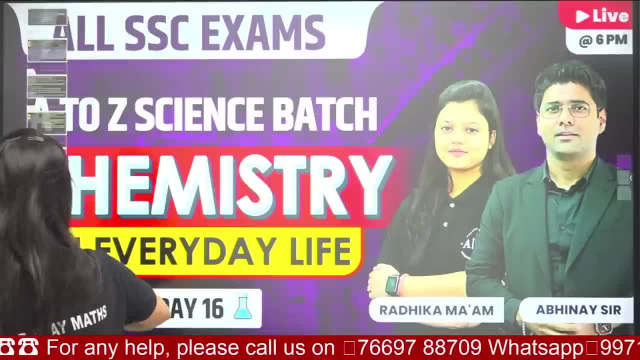 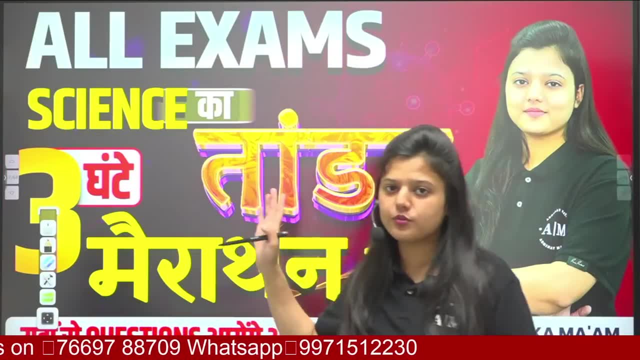 What you people are saying is that you have an exam, children, But we are on this Saturday. We are bringing a marathon for you In which all the important questions of your science will be in the marathon for 3 hours, Like we do daily class at 6 pm. 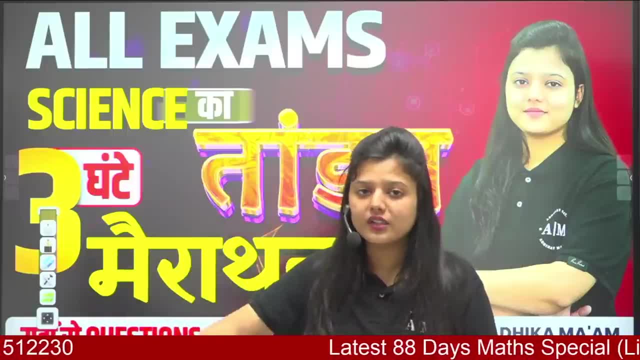 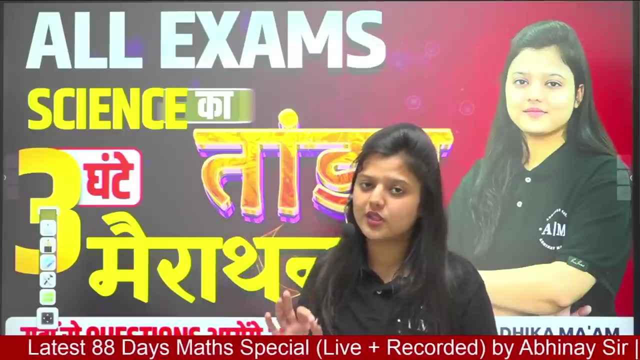 In the same way this Saturday. the Saturday that is coming now will be a marathon of 3 hours from 6 to 9 pm on that Saturday, And in this marathon we are focusing all the expected questions of your science for your SSC exams. 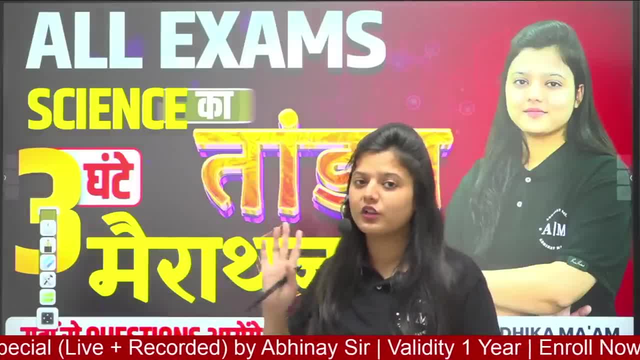 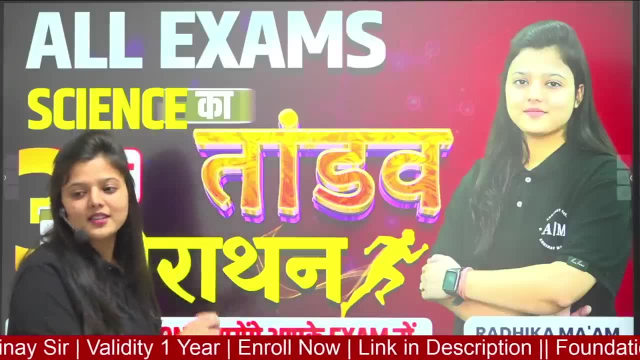 So I have already informed everyone in this session to attend you and do your practice. well, here You are doing revision. you are very smart. So, brother, on Saturday evening at 6 pm, your 3 hour marathon of science is going to be here. 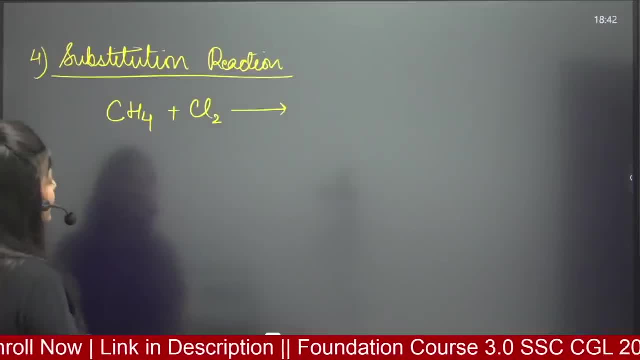 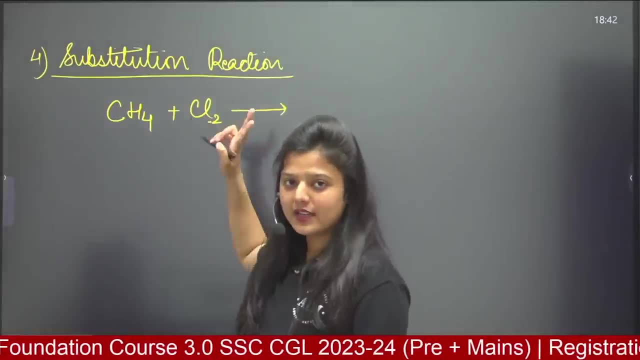 If you are ready, then it is a very good thing. And with this, come on this reaction. Now, madam, what will happen here? CH3, Cl plus HCl: This is chlorine, right, It is Cl2.. There are two in it. 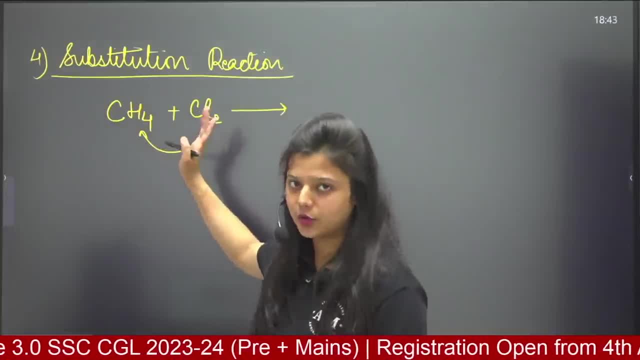 One chlorine will go and will push this hydrogen away. That brother, adjust a little. How will it be adjusted? If one hydrogen of this is removed, then it will remain CH3.. If one chlorine is gone, then Cl Plus one hydrogen which was left. 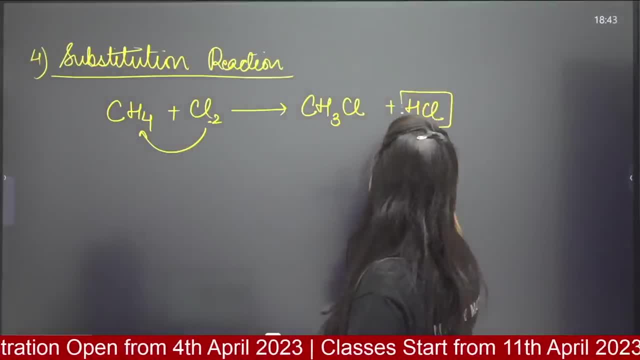 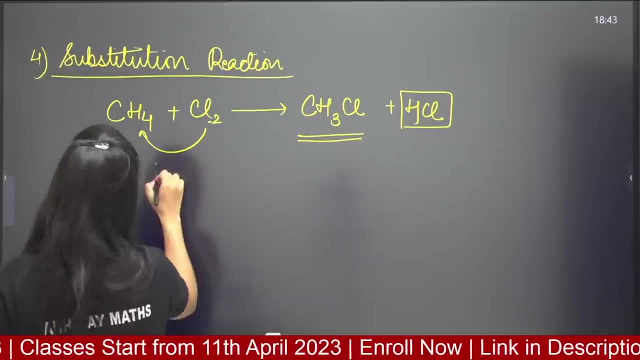 What will it make? by reacting with this Cl, It will make hydrochloric acid. This is what we call expansion. What is happening here? Expansion, Tell me, did you understand or not? This is the law of nature. This is still going on. 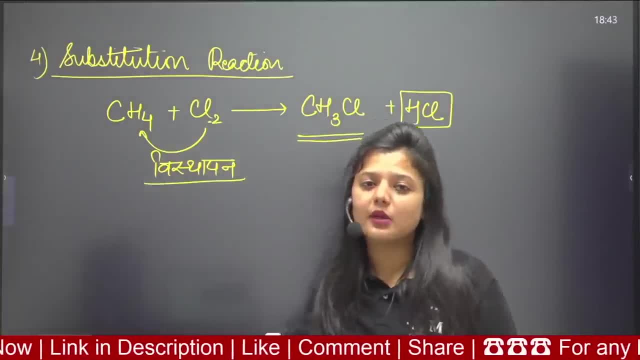 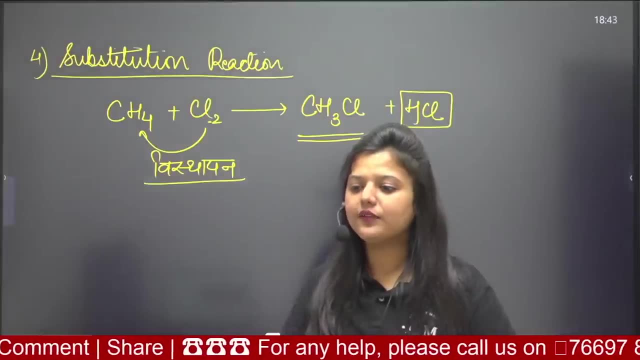 Because of this, your whole evolution story was seen. That brother, the one who has more power. what did he do? He displaced. He displaced, Sunny. that is different. Okay, As you can see, your time is going on. 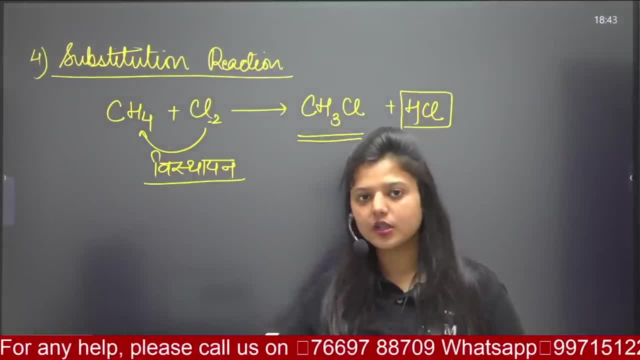 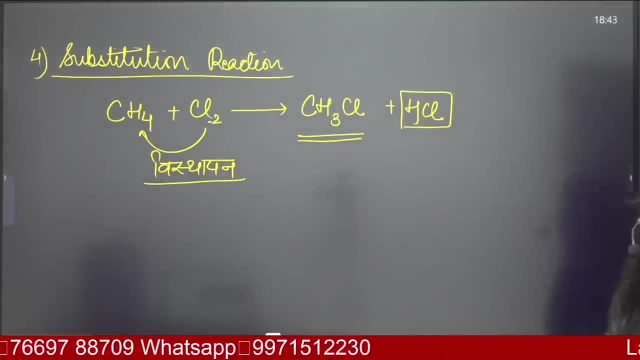 It's going on separately, But this one will be the physics, chemistry, biology, complete. Your class will go here continuously for three hours, Right, This is called expansion. When will this happen? When the sunlight will be present here, That is, you see it happening in the presence of sunlight. 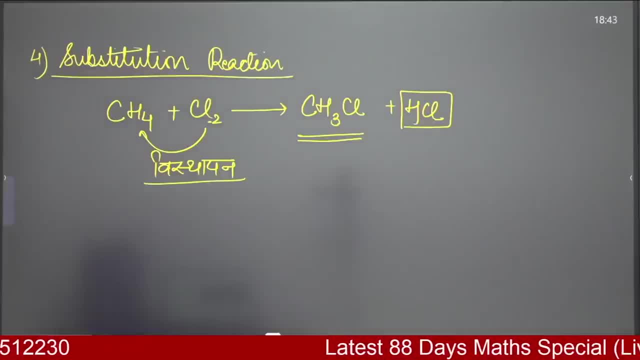 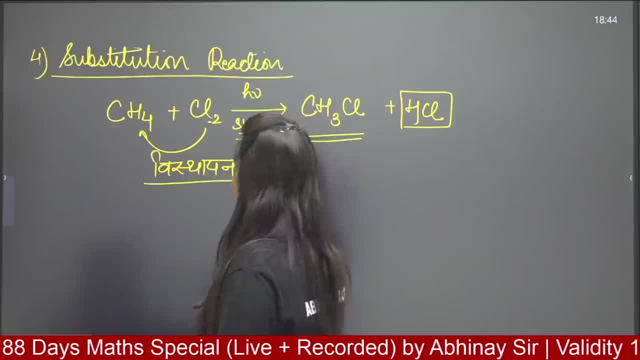 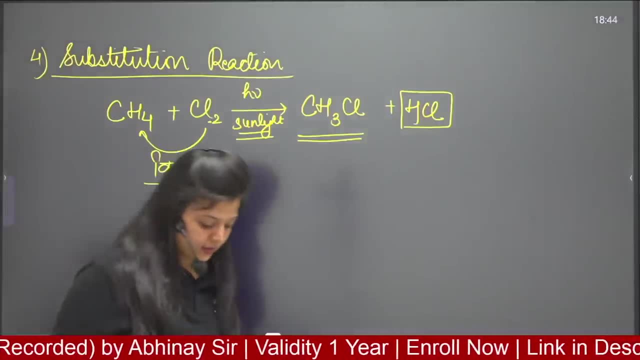 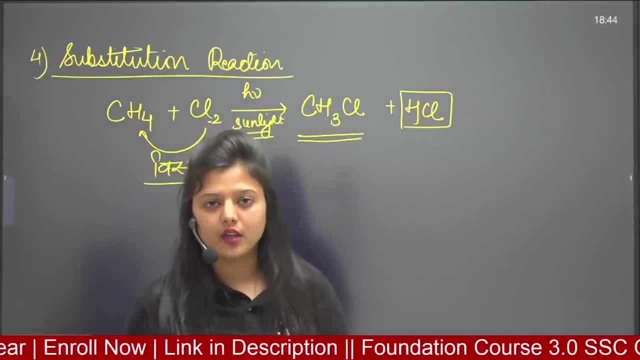 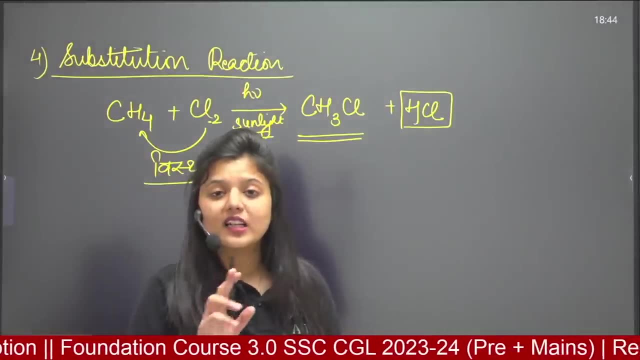 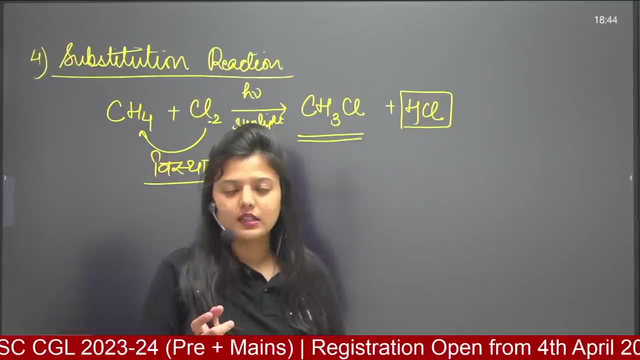 But if you bring chloroform outside in sunlight, If you have seen it- it is kept in brown bottles so that there is no light on it. Chloroform bottles. Now, this secret should be between us. listen carefully first When it is talked about chloroform. then chloroform is kept in brown bottles. It is saved from oxidation. Suppose someone has not studied, No one knows. a thief took the chloroform bottle. He knew that I will smell this chloroform and steal it in his house. And what will I do after going? I will easily steal my stuff. 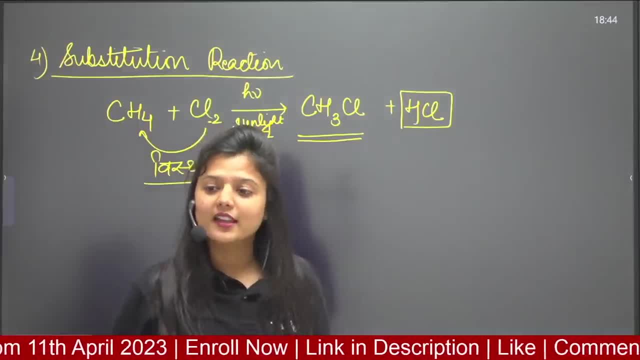 The goal from which he had gone. that goal can also be unsuccessful. How can it be, ma'am? he had gone with chloroform, But he forgot that if I oxidize chloroform, If I keep it in an open place for a long time, then chloroform will not remain. 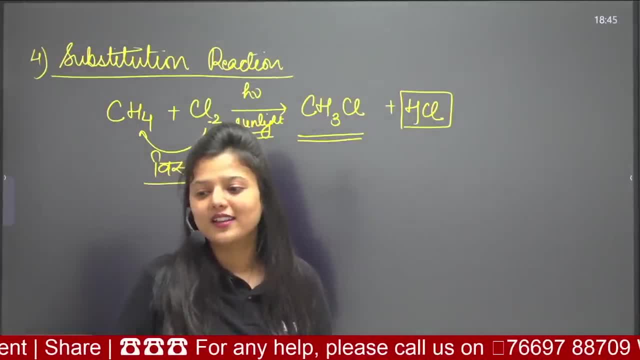 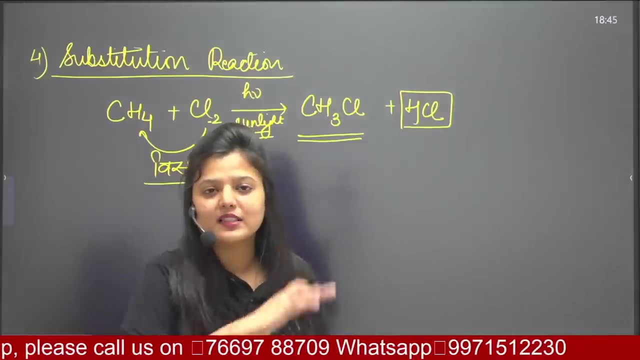 It will become poison. Right, It will become poison. Chloroform is what it is, And the same chloroform becomes your poison. So some people went to steal And later it turned out that the person who smelled the chloroform died. He said: I didn't think about it. 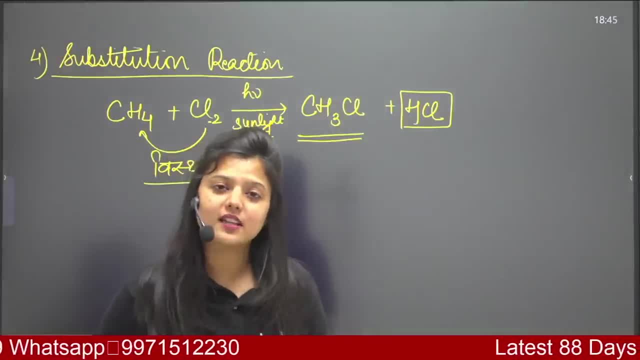 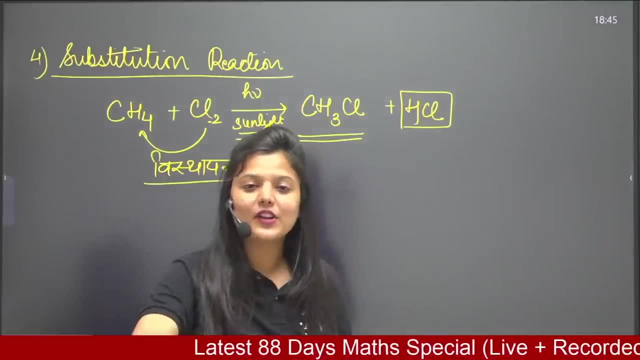 I smelled chloroform. That person should have been unconscious. How did he die? He died because he didn't have chloroform. It was oxidized. It was oxidized. So everything will be studied according to science. So you will know things And things are done according to that. 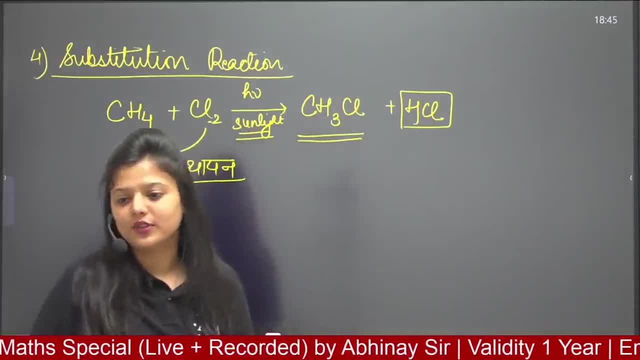 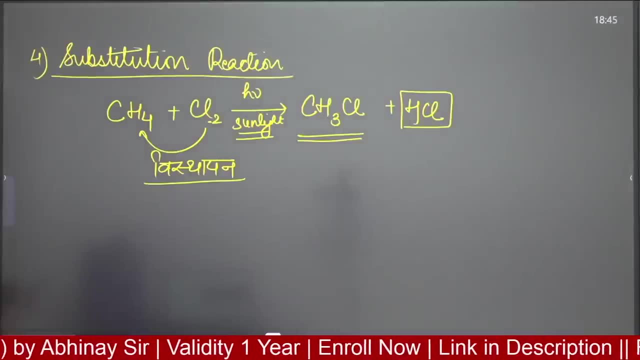 Before the time of operation. This is what happens. Do not do anything, Because it is like that. Over that he lost all his life. It is so untreatable. Here we are Like いねぇ, Even if you have not given you, If we are oh. 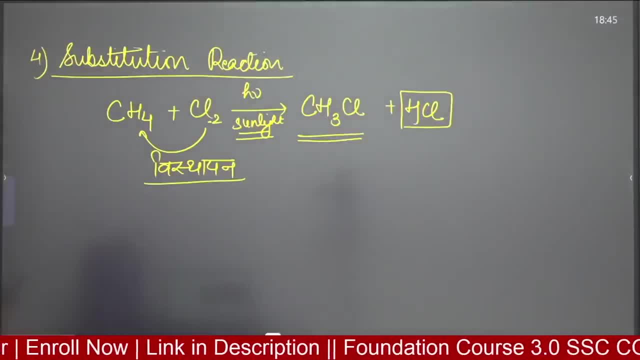 I 전에. So as something like this: Next brzy You can do. That's an incentive, Do you like this? If you have there, Let everyone go. Let all of you tell her, Let everyone know, Say yes, Work. To say haar, There is anything wrong, Don't go. 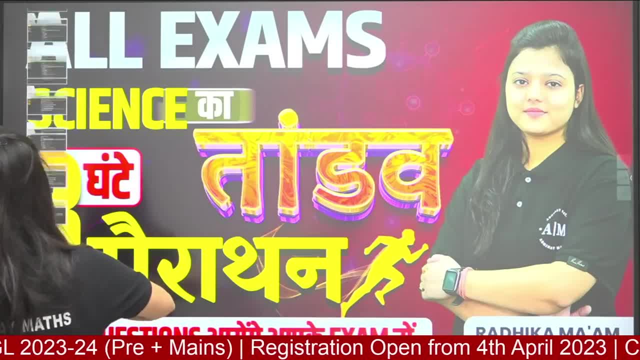 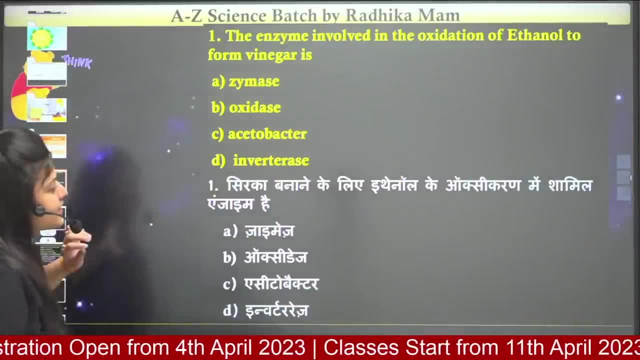 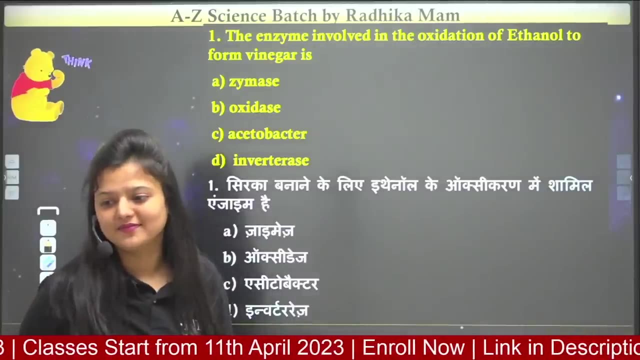 Then, heiden, Don't give anything, brother. Ask a these brother, and let's see what you guys are going to do here. First question on your screen: which enzyme will be included in the ethanol's oxy-current to make the vinegar? Everything is being noted in the mind, very good. 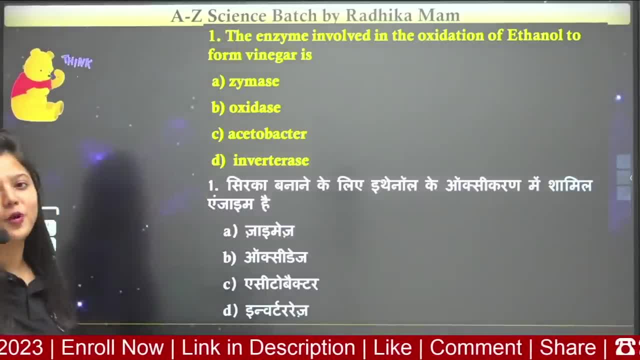 He is asking you which enzyme is called the enzyme which is involved in the oxidation of ethanol to form vinegar, Zymase, Oxidase, Acetobacter or Invertase Or Invertase. Which enzyme is shown to be working here? 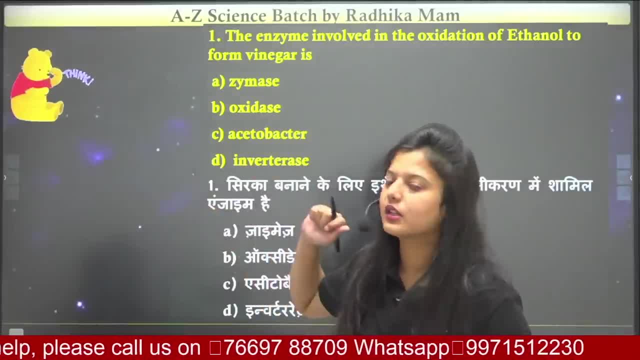 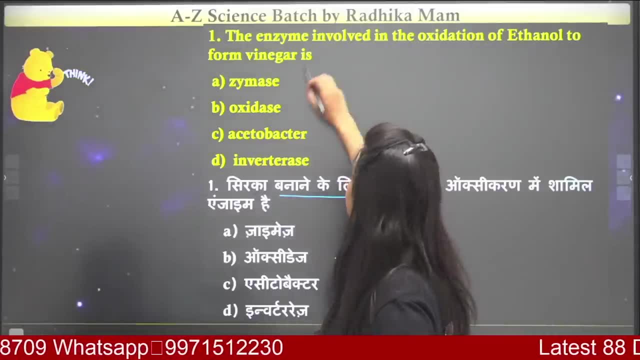 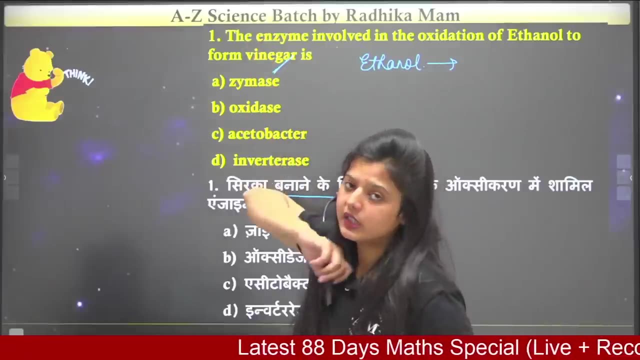 Questions can be made in any way, so we will take all kinds of questions. Now here he is telling you that you have to make a vinegar. which is making vinegar from your ethanol's ethyl alcohol. Now I remember a word for vinegar, that is Acetic Acid. 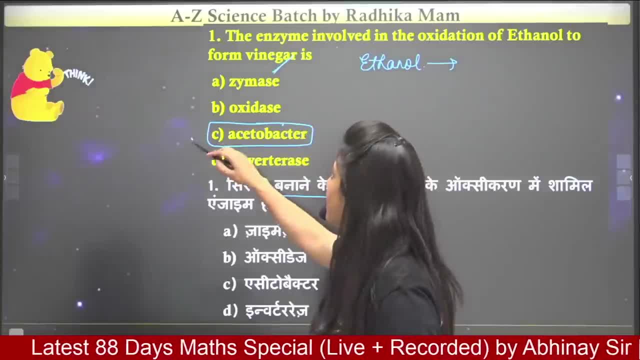 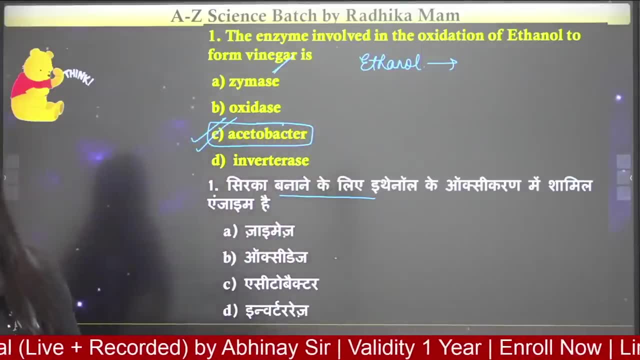 This was working and at the same time, our Acetobacter Acid. it will work as an enzyme, because what are we making with this? We are making vinegar with this, So we have to do the oxidation of ethanol here and what we have to make. 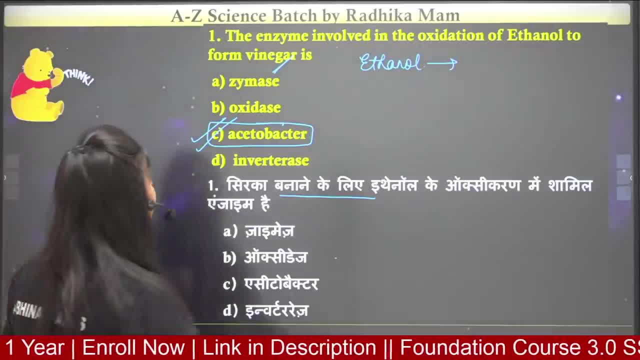 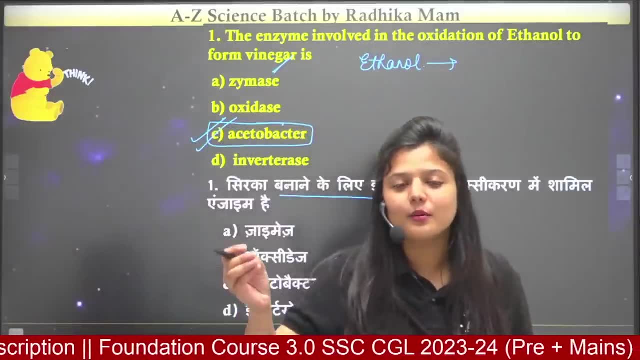 We have to make vinegar. So the answer that will not work will be that if oxidation is happening, then I will bring the enzyme named Oxidase. Remember one trick: that everyone has washed their hands in the flowing Ganga, Brother, if you do the same work at the exam center. one has asked, one is wrong, everyone is wrong. 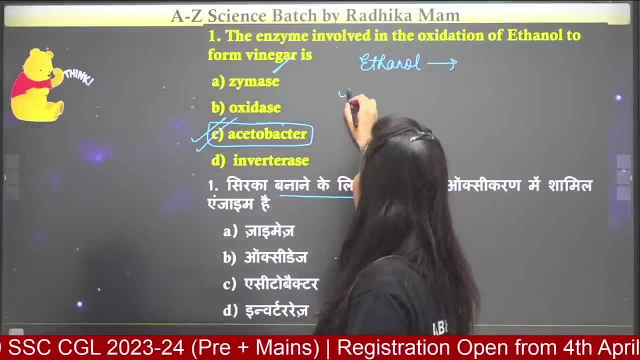 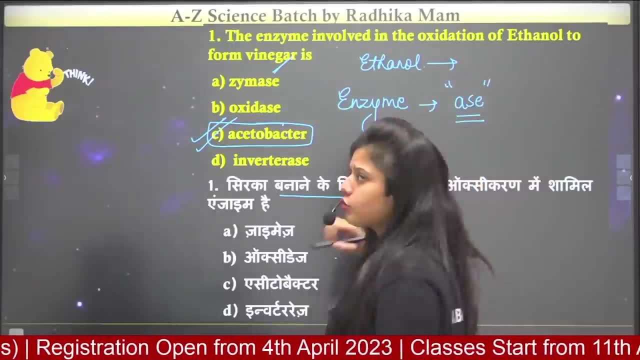 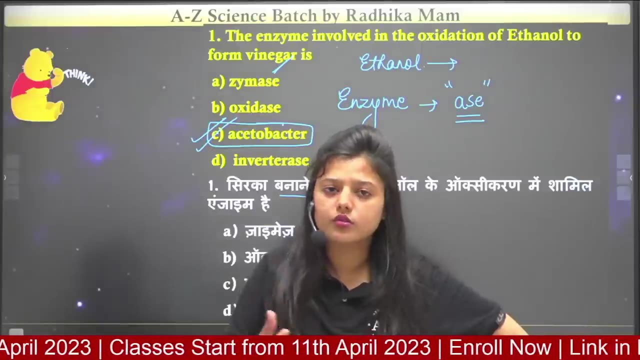 We don't have to do that work. Usually, when you see the enzyme, then the name of the enzyme is attached behind it. See, these are small words. they become mnemonics which will help you further. I tell you that all the carbs, all the sucrose, glucose, galactose, lactose, maltose, 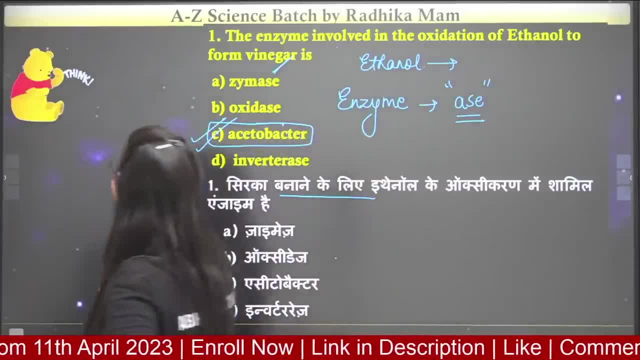 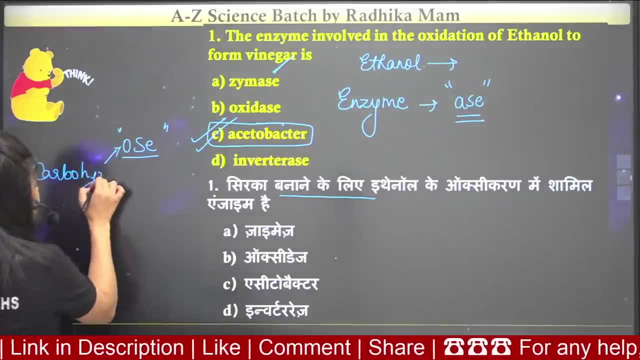 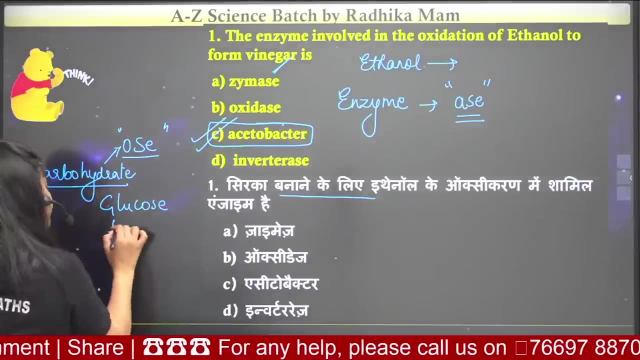 what is coming behind all these names? OSE is coming. What is coming, OSE? Who is this coming behind, Behind the carbs? Usually you will see that behind the name of the majority carbohydrates, OSE is attached. For example, if I talk about glucose, if I talk about fructose, 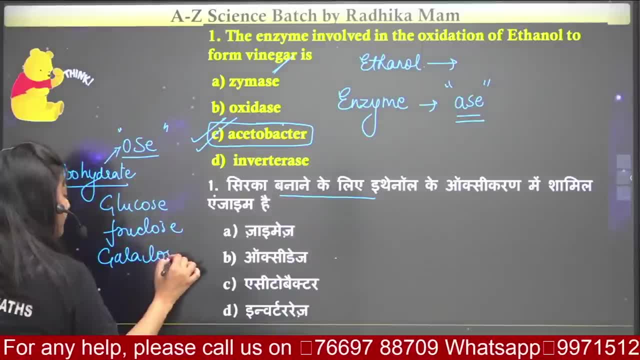 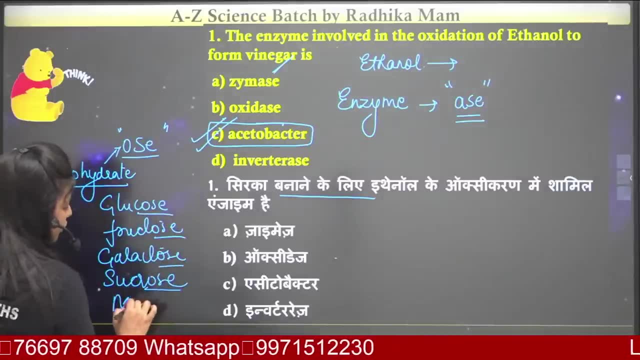 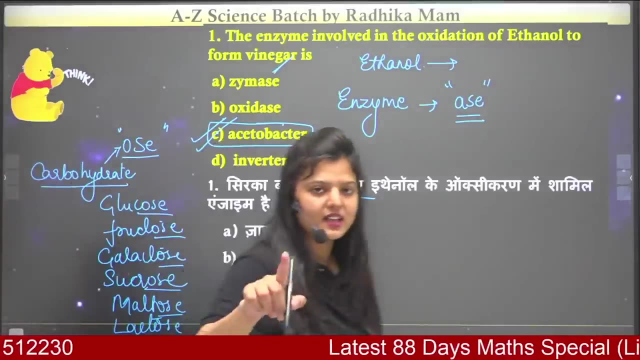 if I say like this: there is galactose, Okay, then I said, brother, there is sucrose, there is maltose. So what do you see behind all these names? OSE is visible. There is lactose, So this becomes a property to find that OSE is coming. 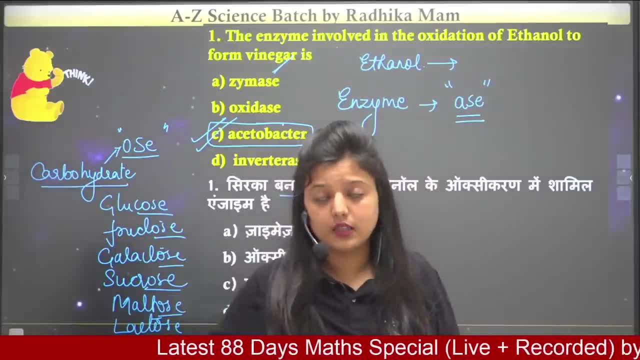 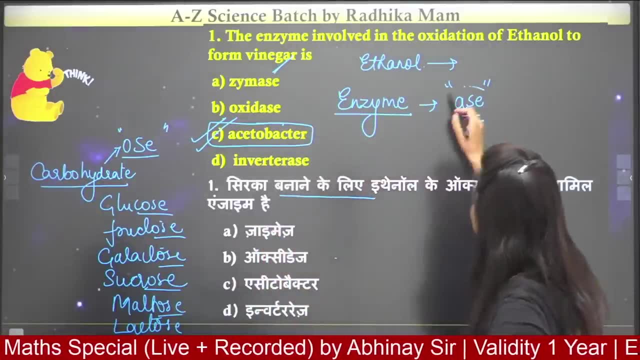 So somewhere it can relate that it could be a. what is the name? Carbohydrate or carbohydrate, we can call it. Now you are drunk. what did you do? All the enzymes. you see, there is ASE behind it. Remember this trick too. 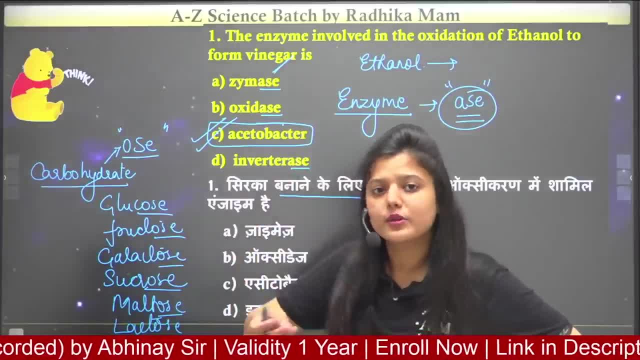 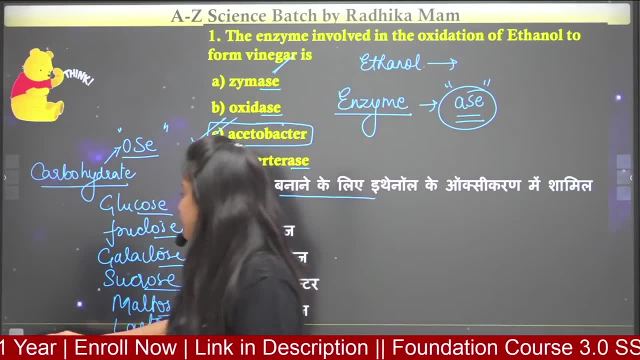 ASE: oxidase, zymase, invertase, lactase, maltase. When enzymes are formed, then ASE is formed behind it. Now here we have, oxidized in ethanolic acetic acid. Come here, I just taught. 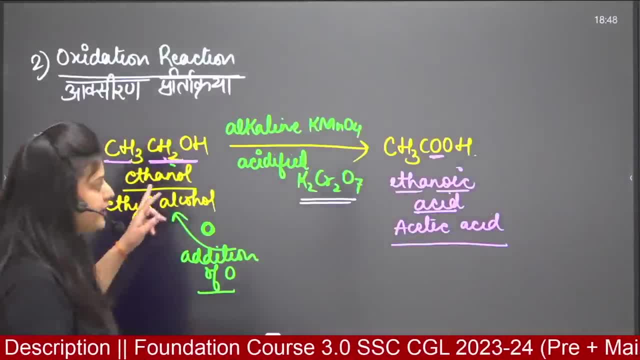 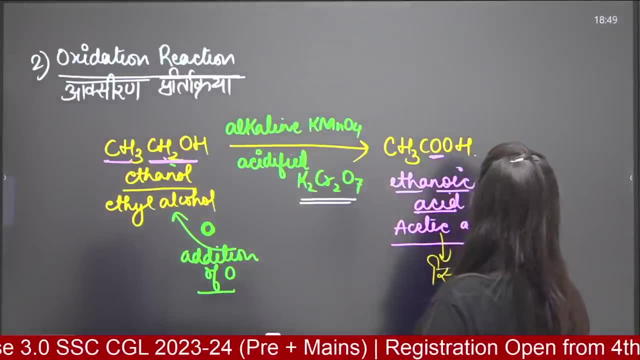 I just taught oxidation reaction. Look here carefully. what is this? Ethanol? What are you making? Ethanolic acid, acetic acid And, ultimately, what do we get from this? Can't we make vinegar, Vinegar? Can we make it or not? 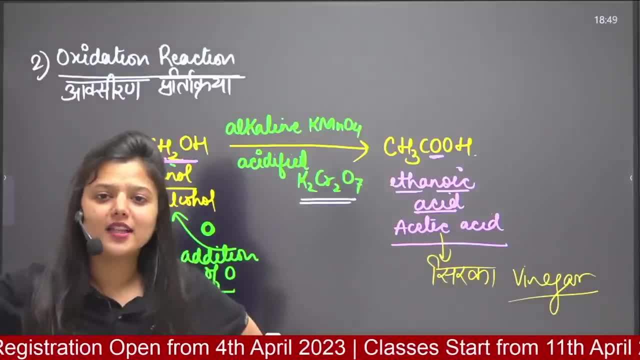 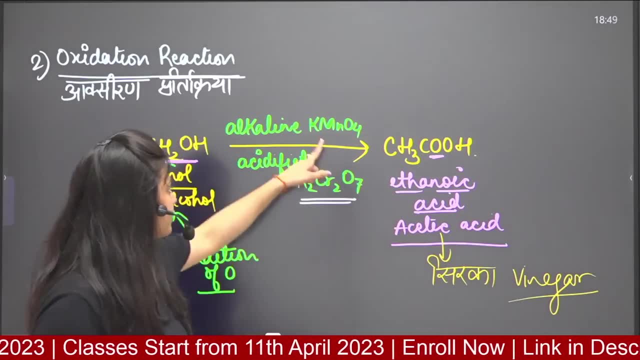 Now this is the story, ma'am. Someone must have given the answer. We all have oxidized with B. Which enzyme did you make? Because it is working here then? either it is alkaline ammonophore and potassium dichromate is given here acidified. 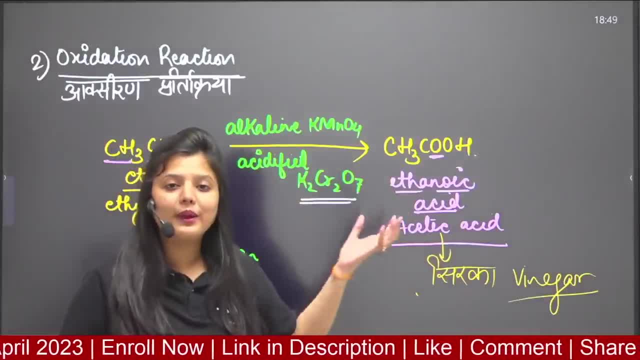 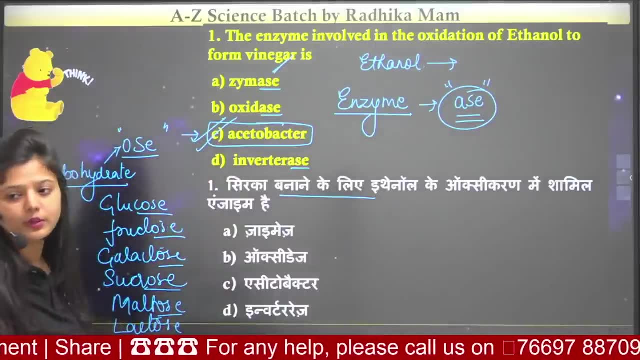 Or because it is becoming acetic acid, then acetobacter In this question, what will happen? Option number C will happen. Does anyone have any doubt in this? Tell me quickly once This works in inverted sugar, invertase When we do conversion with sucrose. 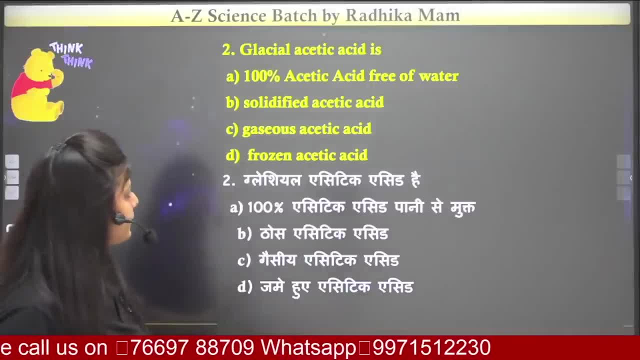 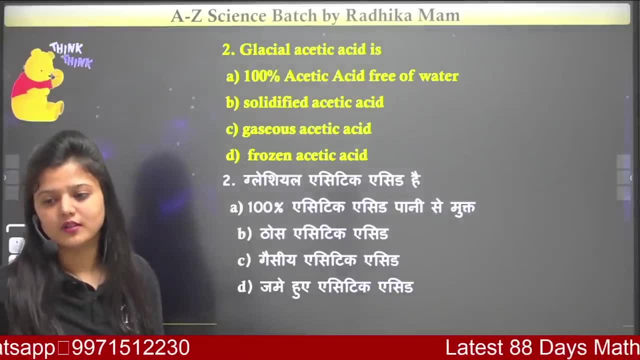 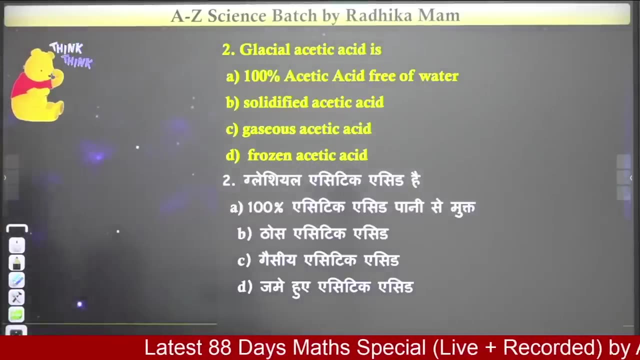 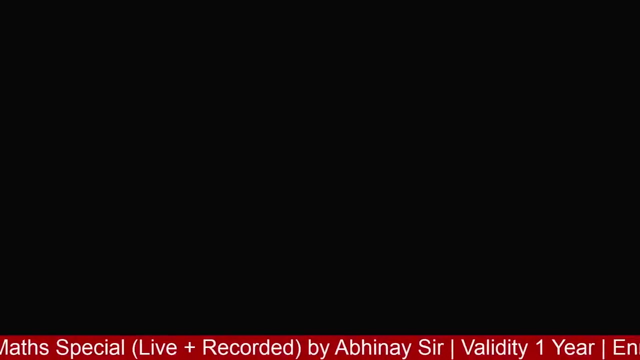 Next question will tell what is glacial acetic acid. Is it solidified, Is it gaseous, Is it frozen or what? Come on, Answer once quickly What is glacial acetic acid. Answer once quickly What is glacial acetic acid. 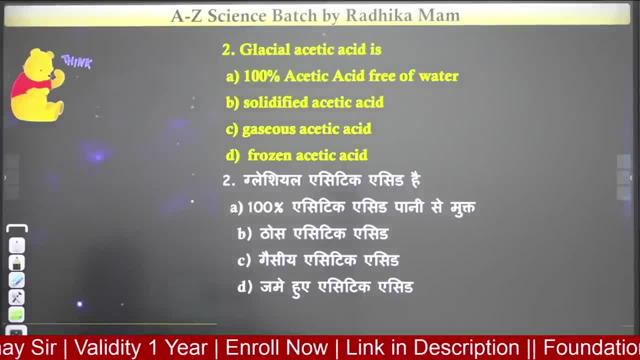 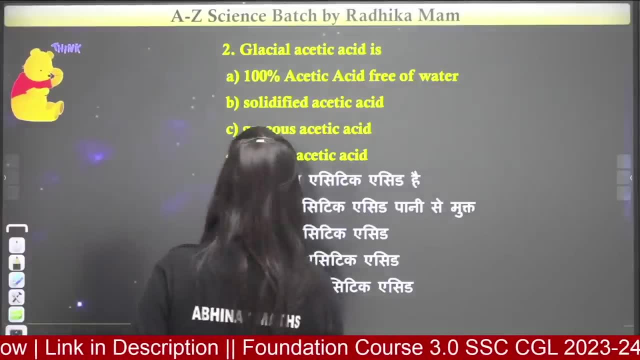 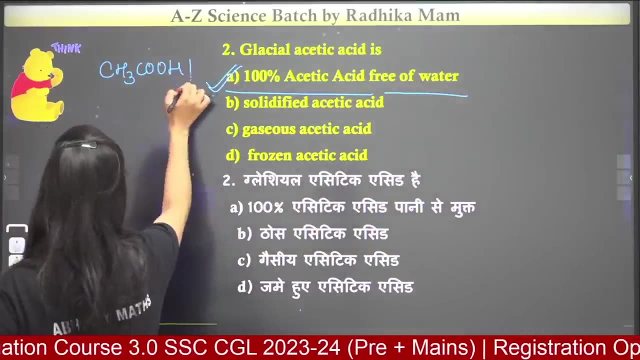 Answer once quickly. He is asking you: what is glacial acetic acid? Now, if I talk about 100% acetic acid without water, 100% acetic acid without water, Acetic acid means CH3COOH, CH3COOH. 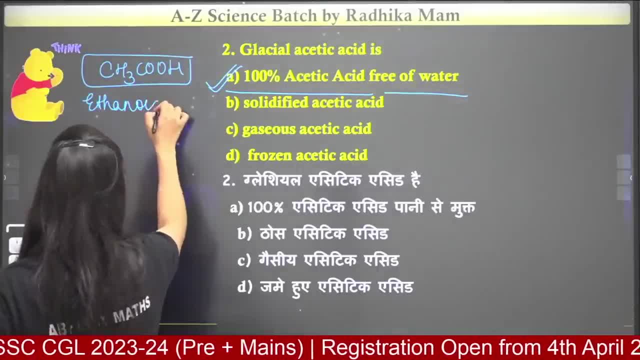 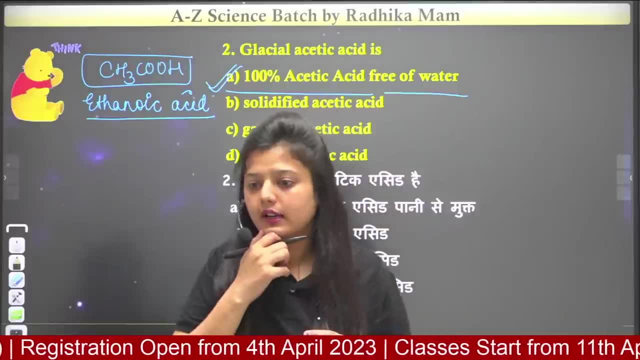 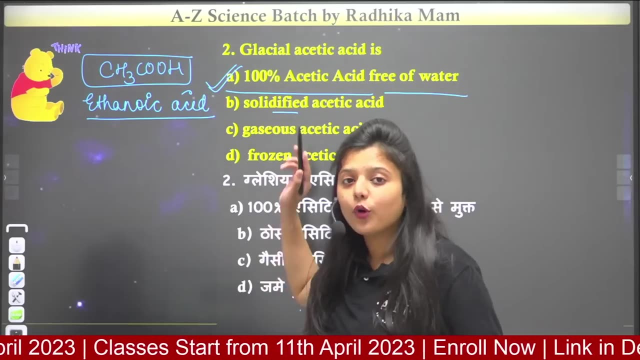 Ethanoic Acid. Ethanoic Acid means a solidified acid. This is called Glacial Acid. You thought it is a glacier word. It is made of ice. Glacial means it is pure. This is 100% acetic acid. 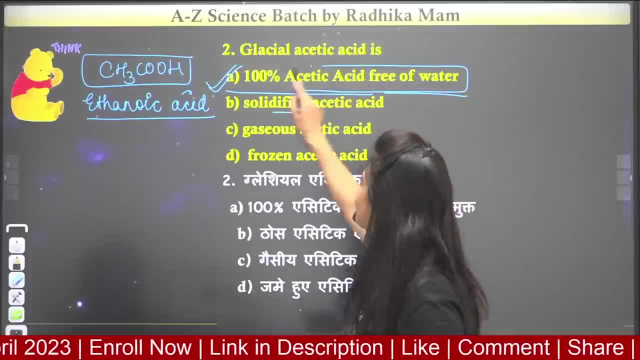 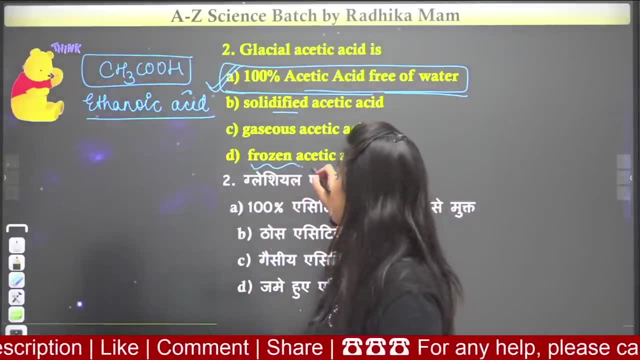 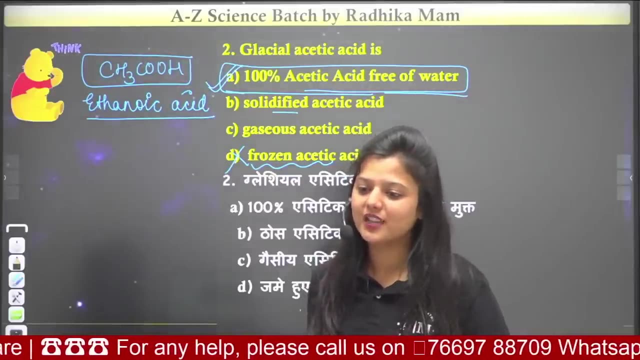 without water. It is called Glacial Acetic Acid. It is the game of words, You have to understand it. a little is also making frozen, and here only examiner will judge you that in how much water you are. all things are getting clear and whatever friends are new to us, brother, if things are, 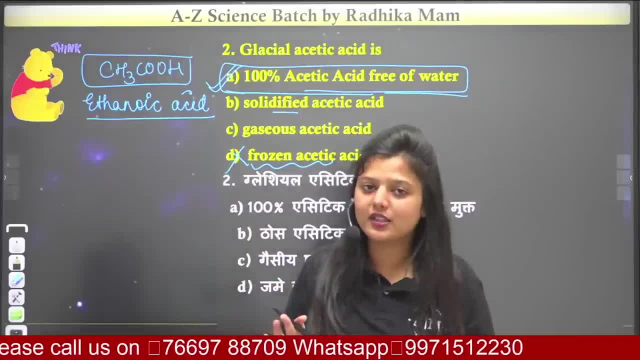 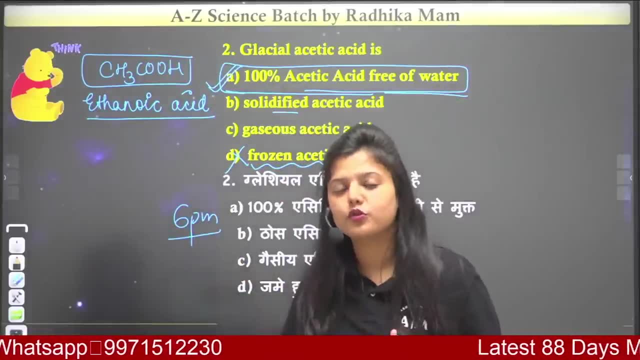 coming to understand, then like the session and share it quickly once plus. daily class is at 6 pm, so don't forget. and every evening at 6 pm you have to do the complete topics ahead of you. tomorrow we will study polymers and we will also study about soap and detergents. 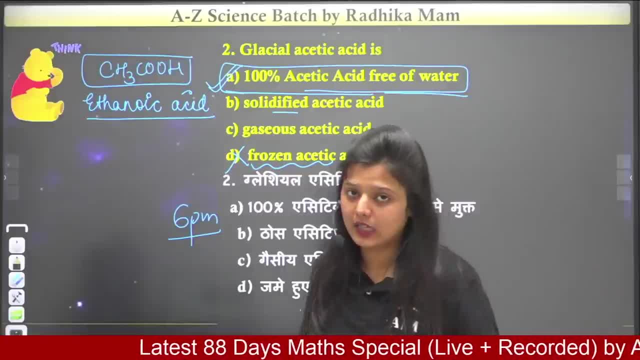 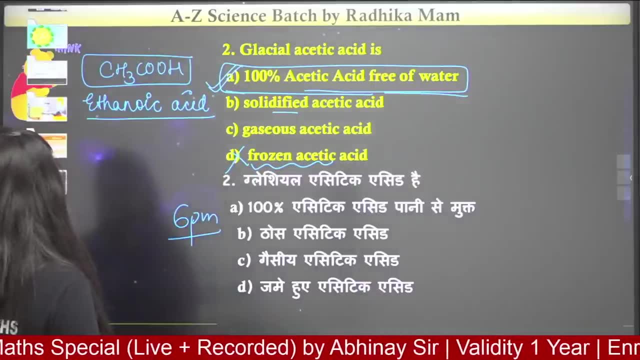 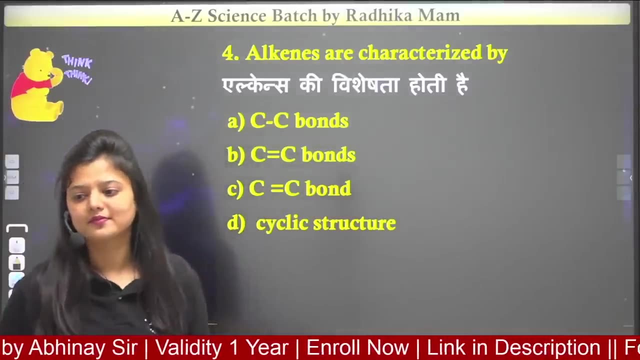 and what is hard water that makes what soft water is ok, yes. when not, then the question is hard. Let's see. the next question characterizes by the speciality of Alkene. Tell me to whom you can do salchow. 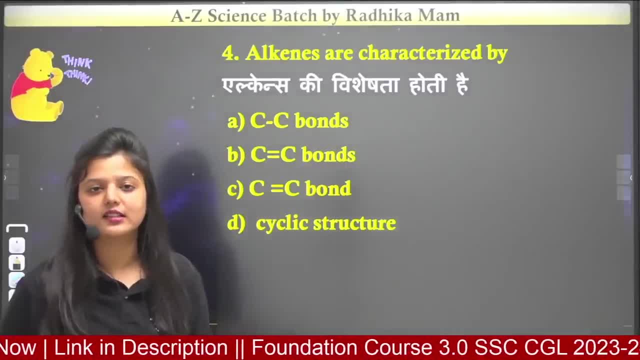 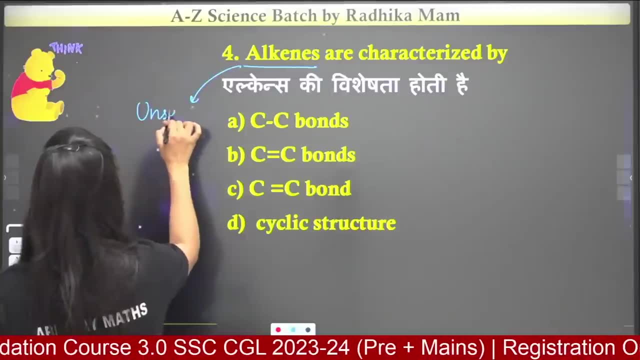 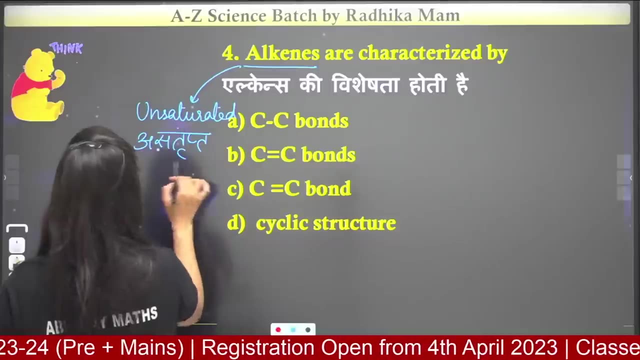 Who can make the speciality of my alkenes? I have Alkenes, So we know this is unsaturated water. Yes, that is right. Regarding the concept of salchow: unsaturated or I will say unsaturated, or I will say: 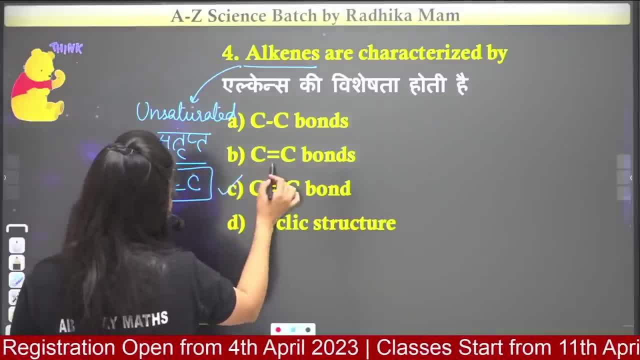 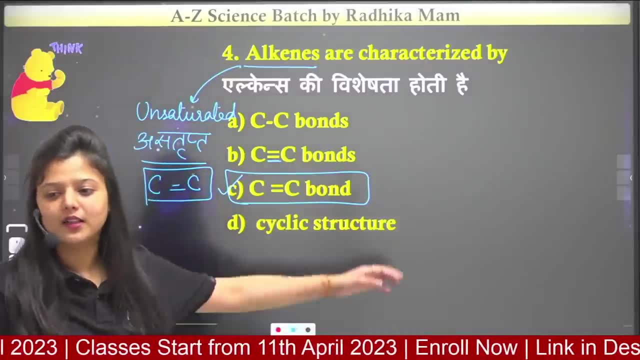 carbon double bond carbon. you can do it with whom. let's put triple here, let's call it carbon double bond, carbon bond. put B or C, it's the same thing. so carbon double bond, carbon is alkyne, second one is alkyne. this is our alkane. 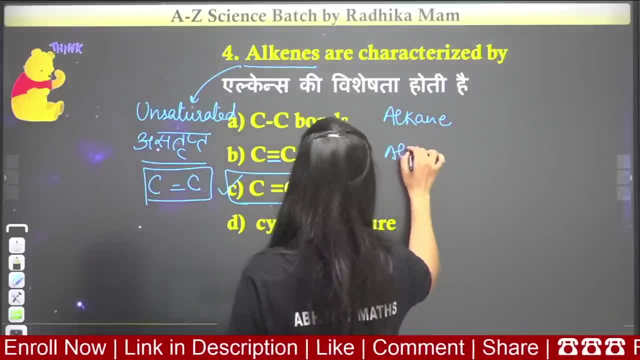 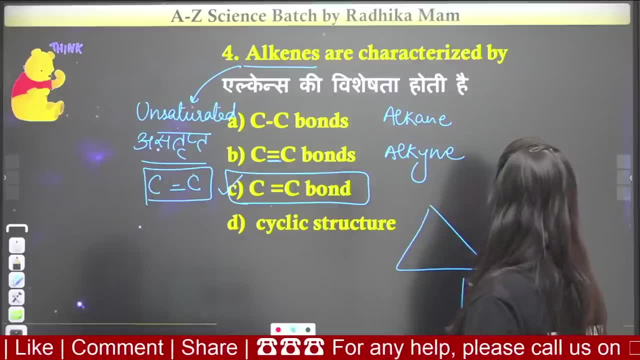 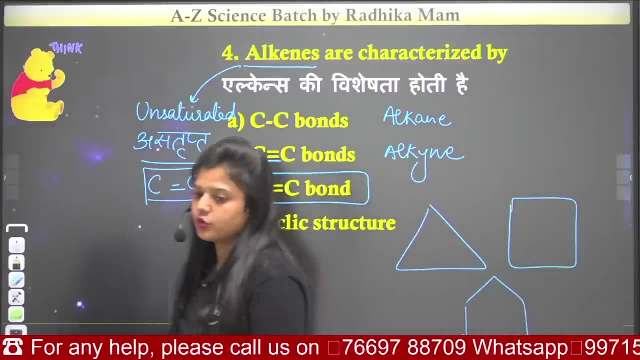 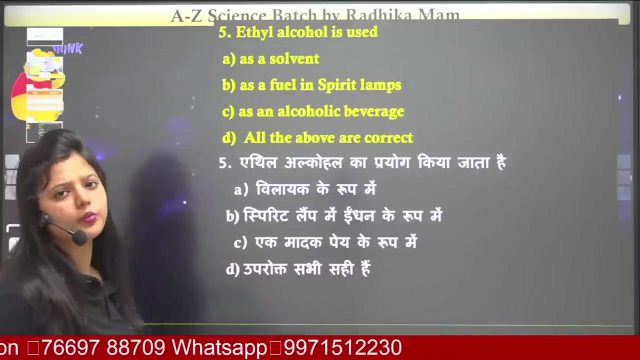 and what will be the cyclic structure? something like this: these are all cyclic structures. these are all cyclic structures. you can see. ok, which is our closed cycle. let's ask the next question, and I have asked you: how can you use ethyl alcohol as a solvent? 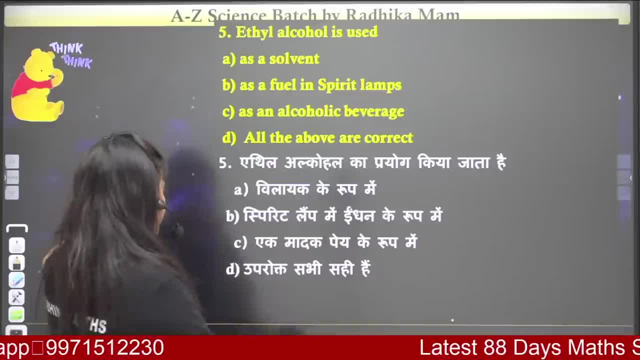 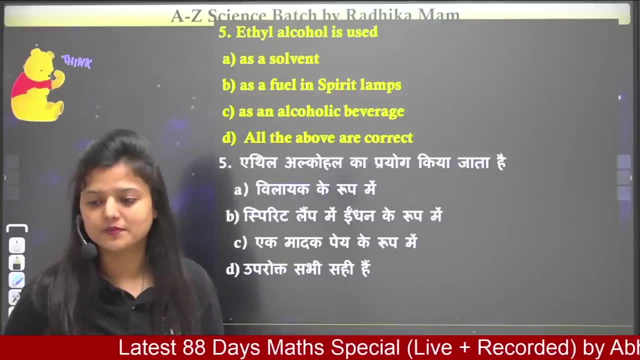 as a spirit lamp, as a fuel, as a glycerin, as an alcohol, as a human being or as a drink, an alcoholic beverage, as a saline. the all options here are correct. all the options are correct. we will tell you once: ethyl alcohol, ethyl alcohol. 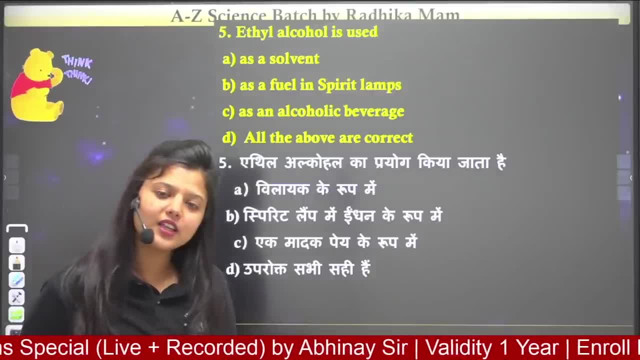 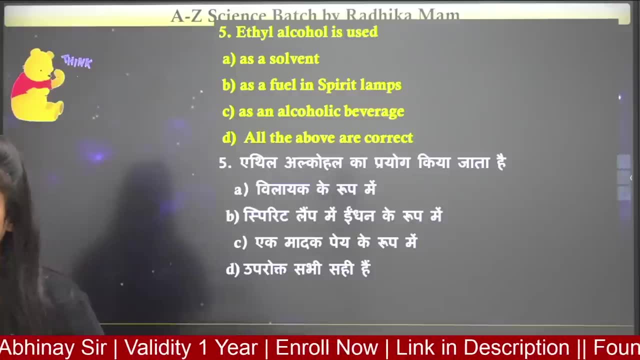 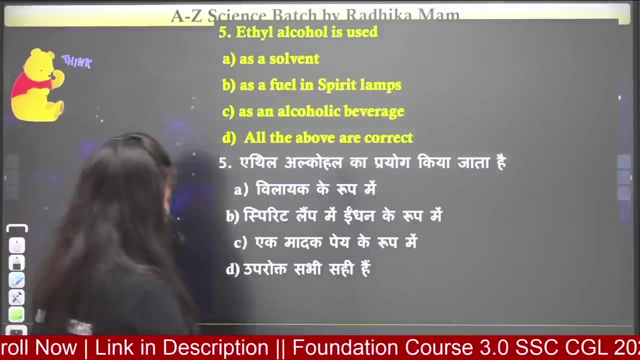 what will you think, madam, if we have made this liquor, then he will add it, but apart from that, can it do anything else? only you did the double bond, the triple bond now, now quickly answer this question, right? but if we are talking about this, 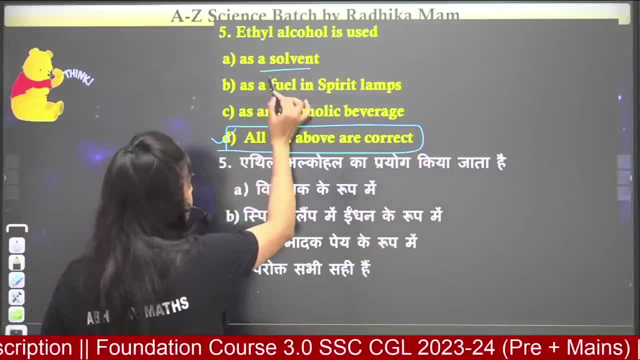 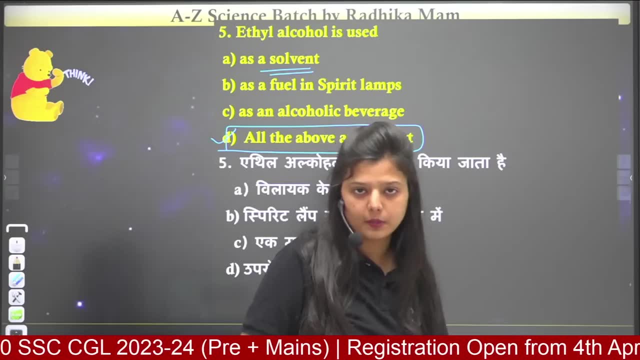 So all is the correct one, because as a solvent, you can see a lot of such things that do not dissolve in water. I also talked about benzene. Benzene is immiscible in water. it is not dissolving in water, then where will it dissolve? 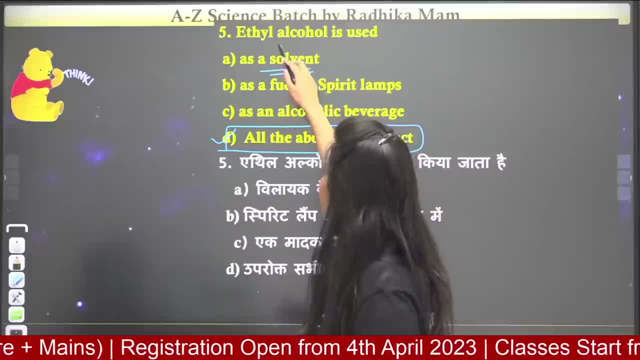 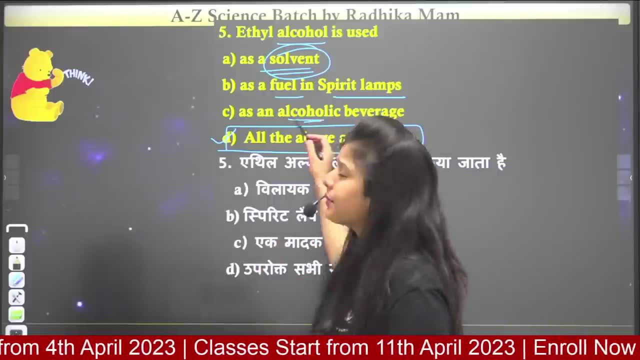 in alcohol. Okay, you will see it in alcohol then ethyl alcohol is also working as a solvent In spirit lamps. fuel also works as a fuel. Alcoholic beverages are seen in all the beer and vodka that are made. so all the options. 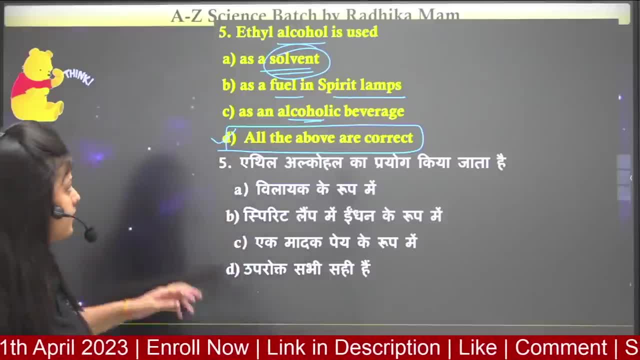 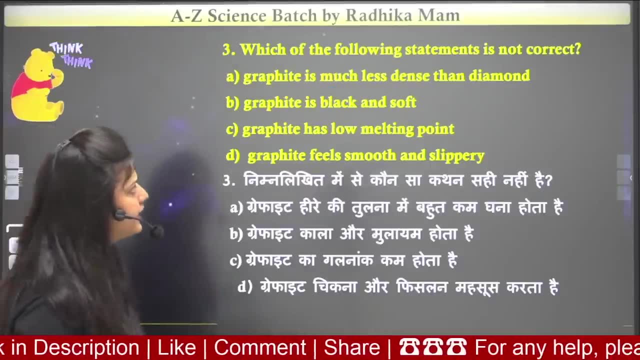 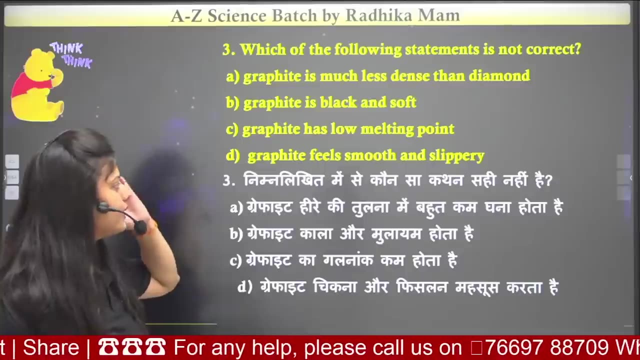 will be correct. that is, all of them are correct. what are all these? the correct ones are visible here. Next question: tell me which one of these is not correct. graphite is less you can see dents from the diamond. graphite is black and soft. it has a slow melting point and 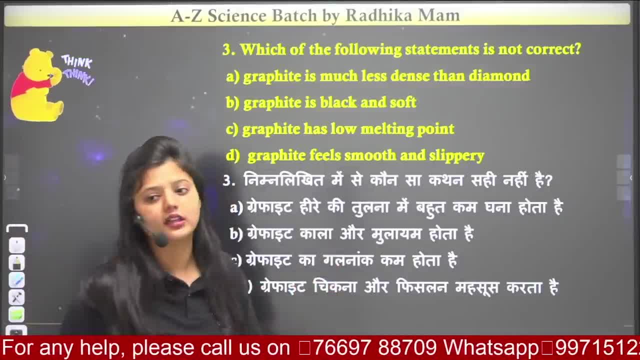 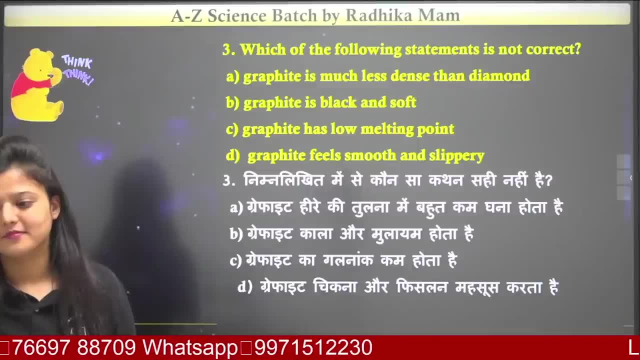 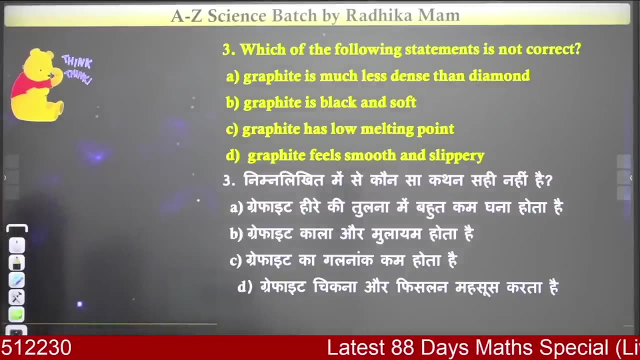 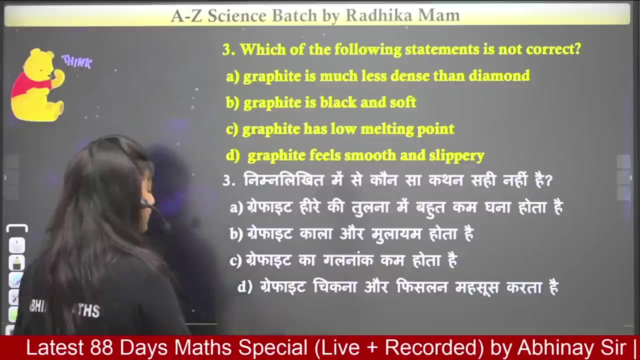 it feels smooth and slippery. which one is not correct? Come on, tell me quickly which one of these is not correct. which statement is wrong over here? Which one of these is not correct? which means it is wrong now, ma'am, you told me that graphite. 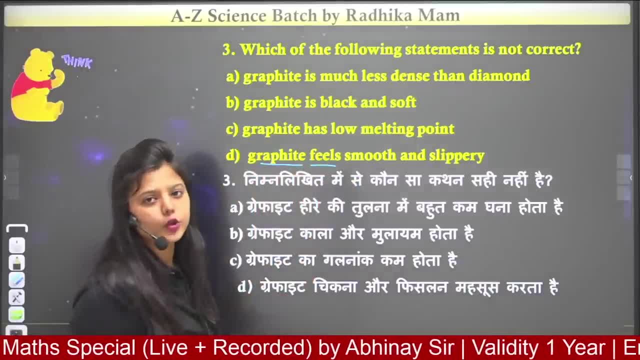 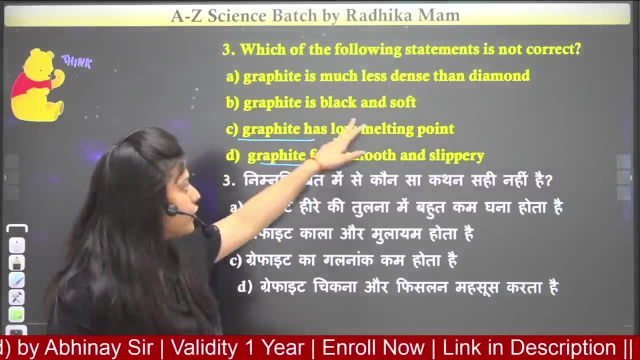 looks smooth and slippery. its layers are on top of each other, so it is very smooth and slippery. If I talk about its melting point, then the number is very less. it looks black and soft. it is black in color and soft, but if I say that it is very less, dense diamond is very 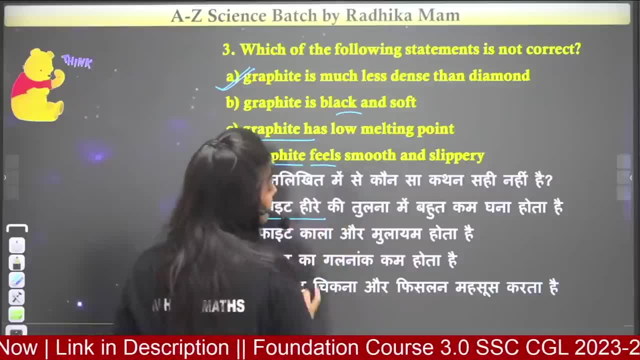 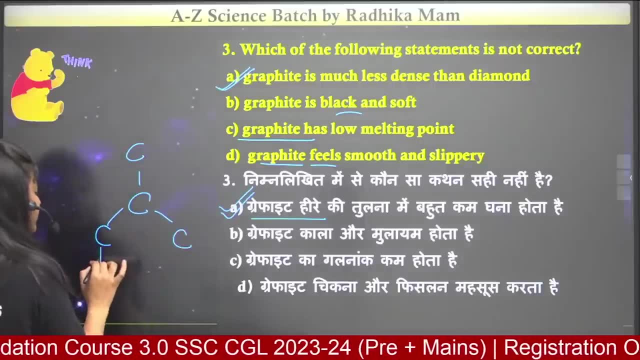 dense. So, brother, if it is less dense than diamond, then this thing will be wrong for us, because what we saw in the diamond is that the carbon is connected with four other carbons. In the same way, we saw the structure of the diamond that every carbon is connected to. 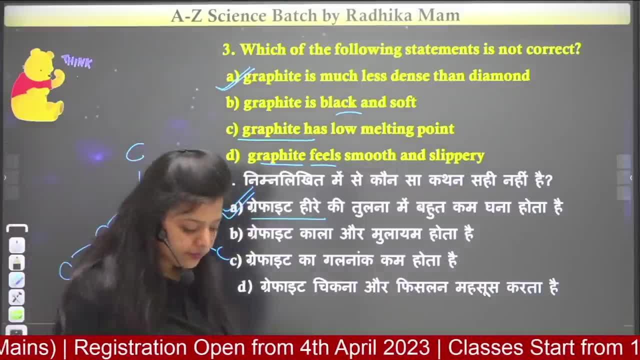 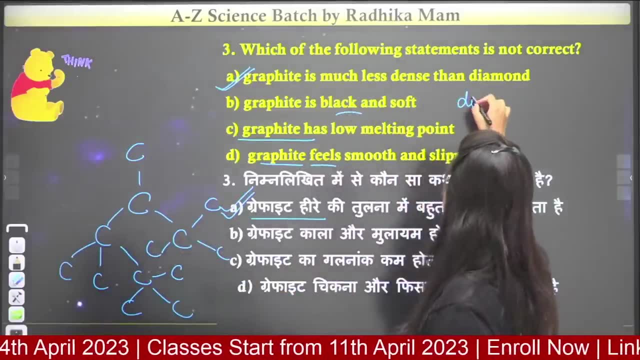 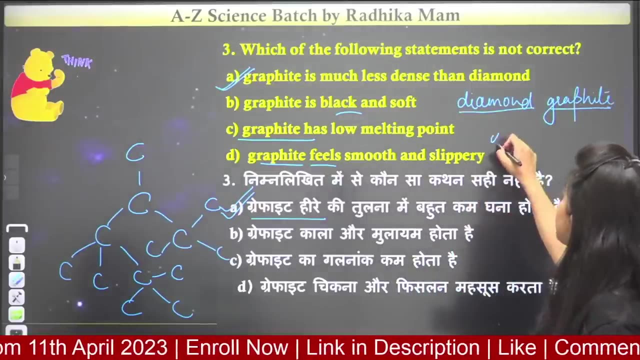 whom and with four other carbons. so if we talk about the density, then our diamond is more dense. graphite will be less dense if I talk about the diamond and graphite from both of them Talk. So which is a good conductor of electricity? tell me quickly who is the good conductor. 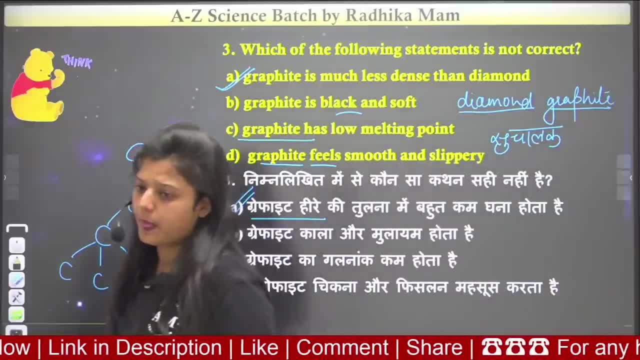 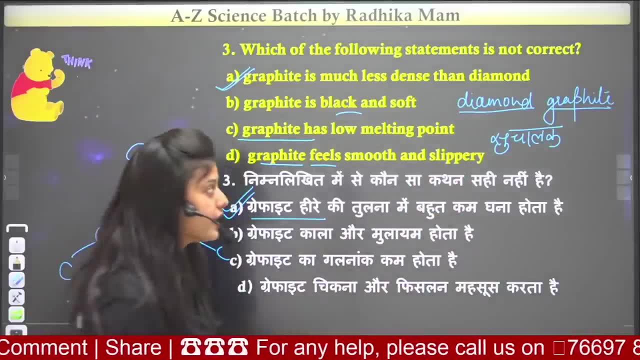 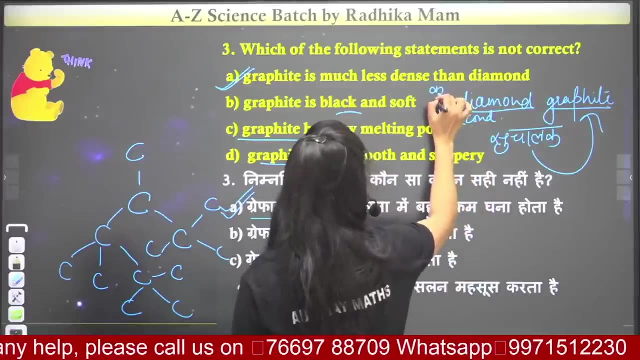 of electricity. is it diamond or graphite? Who can conduct electricity easily, ma'am, it is non-metal, it cannot do it. no, you have to understand here. graphite is a good conductor. what is diamond, bad conductor, which we call ku-chalak? this is called ku-chalak, this is showing its property, but graphite? 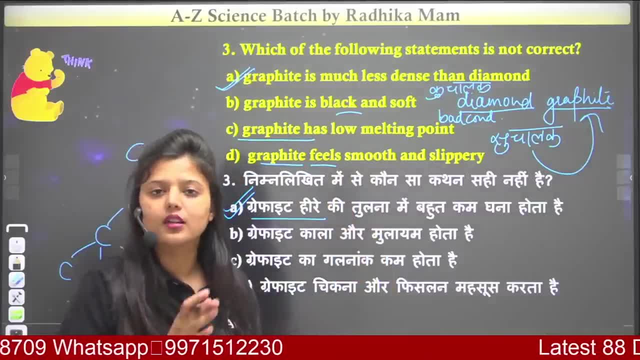 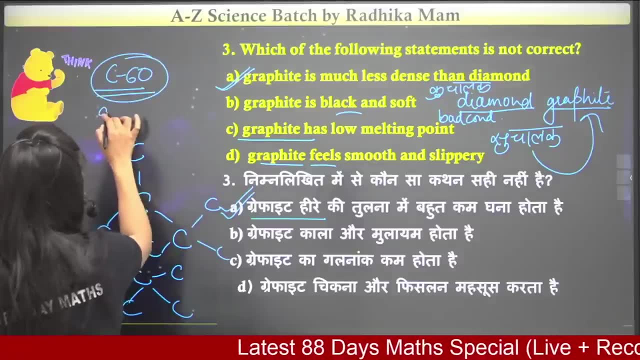 comes under exceptions. graphite comes under exception. I hope this is clear. and here, if we were talking about the C60 allotrope, then the C60 allotrope, which was in geodesic form, it was shown to me like a football. it was developed by a US architect, Buckminster. 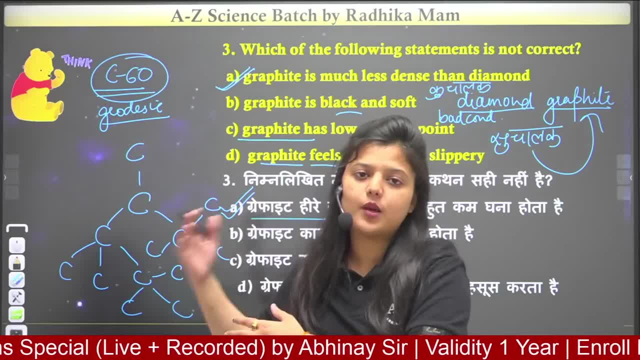 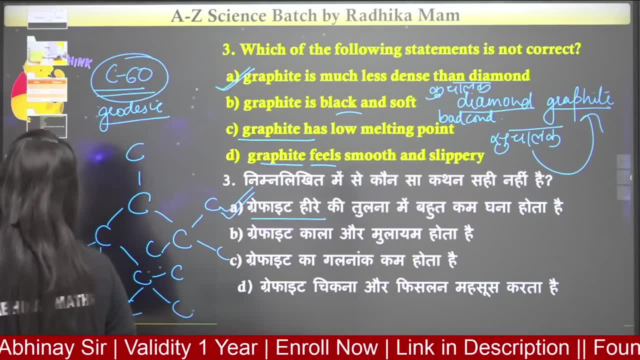 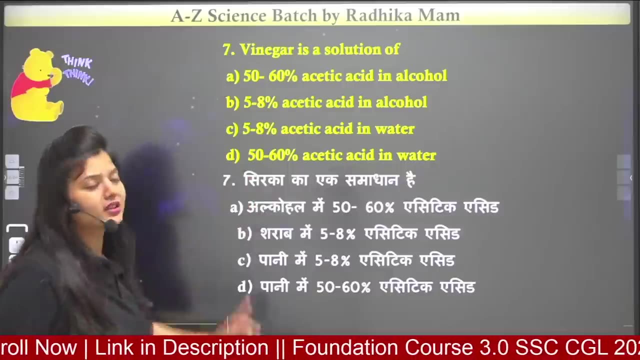 and that is why his name was, on his name, Buckminster Fullerene. so this is also a form of carbon we had seen. this is also a form of carbon which we had seen here. next question will tell vinegar, which is a solution, how many percent of acetic acid? 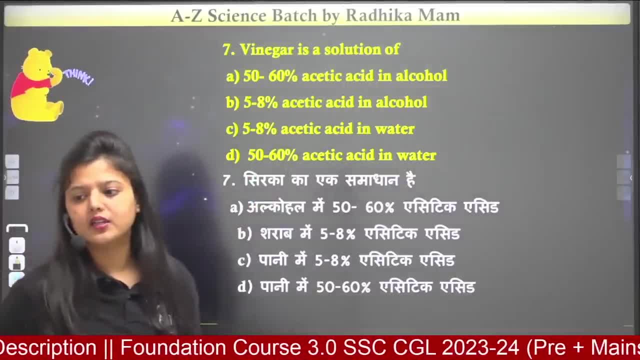 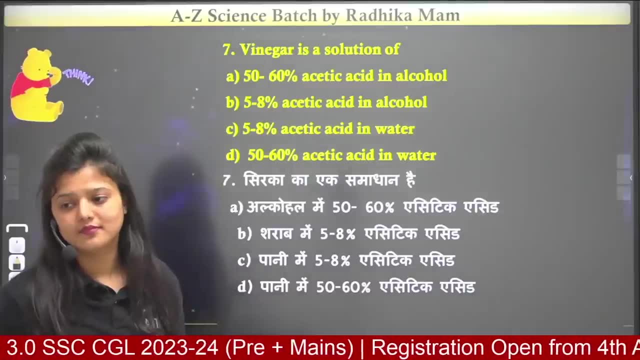 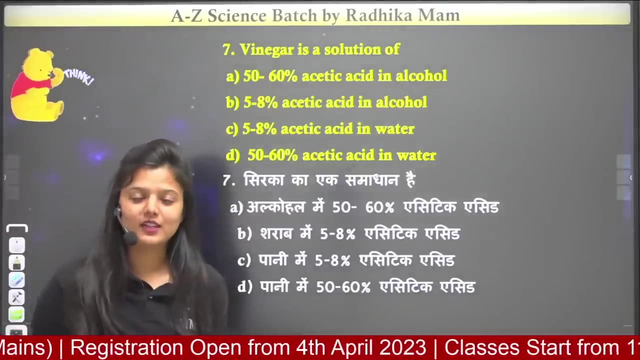 is in water. how many percentage of acetic acid is there in the water? come on, tell me quickly. you are all going to give a CGL exam, right? You are graduate enough, and then you will do such things. so it is also strange to scold. 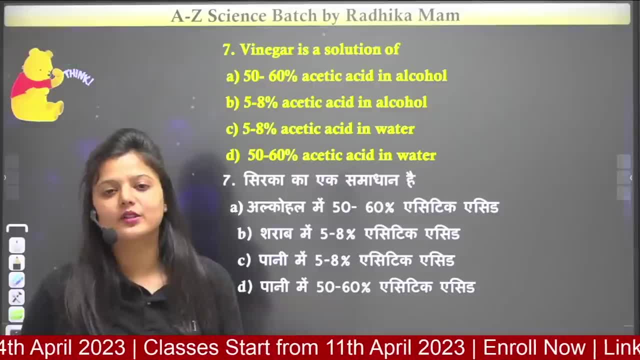 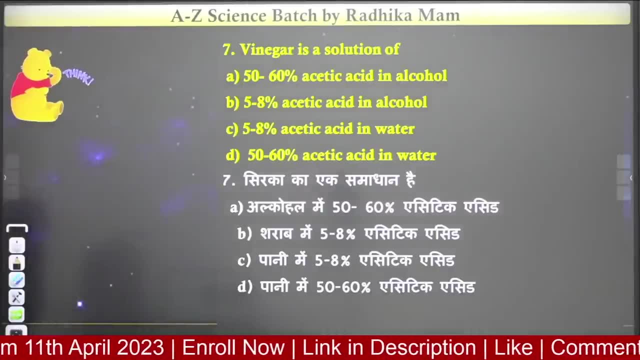 me that you are so smart you have to give the exam. then you will also tell me that you are going to look like an inspector. and then you do such things. tell me vinegar- we are talking about vinegar and the screenshot we are taking. we will also take a screenshot. 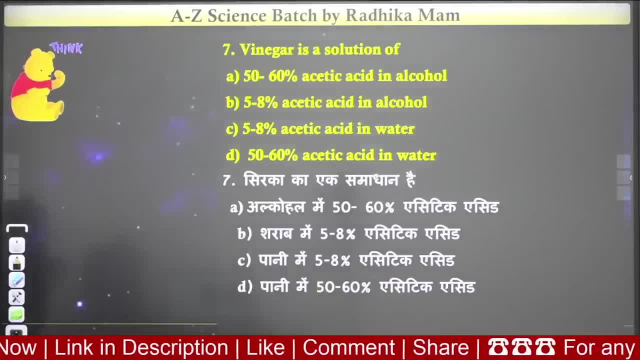 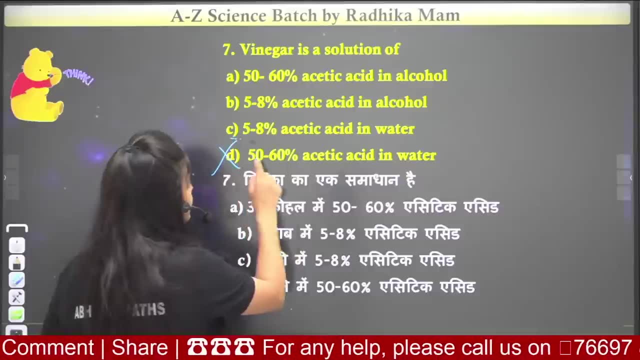 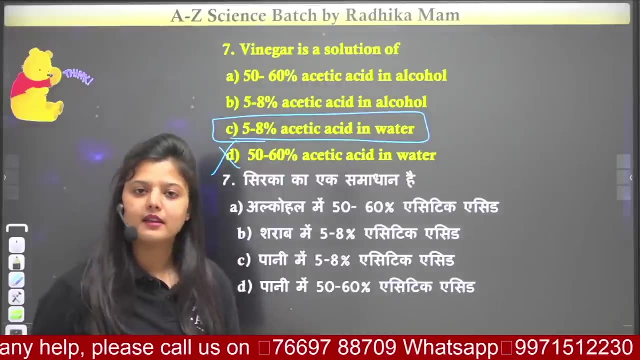 with us. The answer is coming if I say D is wrong. 50 to 60 percent is not there. only 5 to 8 percent acetic acid is in water. it is made in water. acetic acid is put in water only. 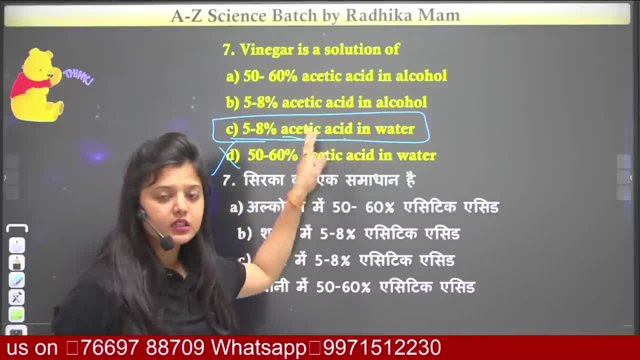 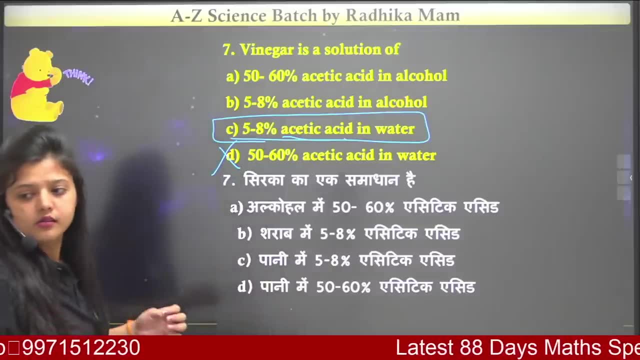 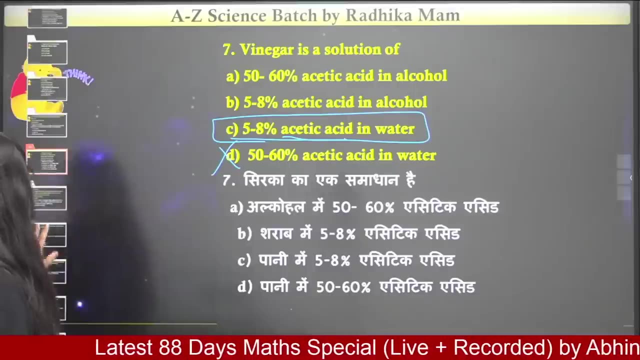 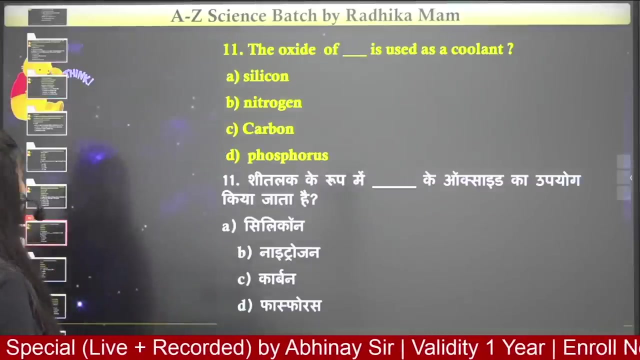 5 to 8 percent. I am saying this acetic acid. if you put this 5 to 8 percent in water, then vinegar, vinegar. it is visible to you. Okay, come on, tell me next. next is that the oxide of dash is used as a coolant: silicon. 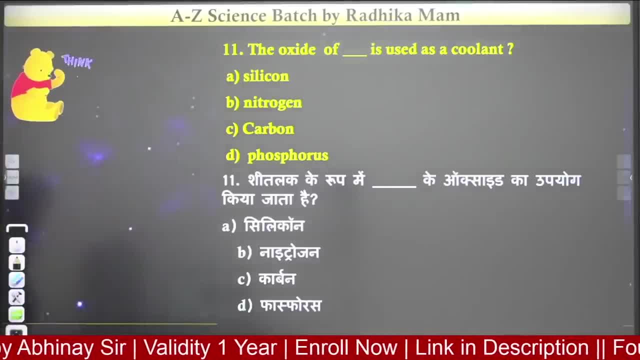 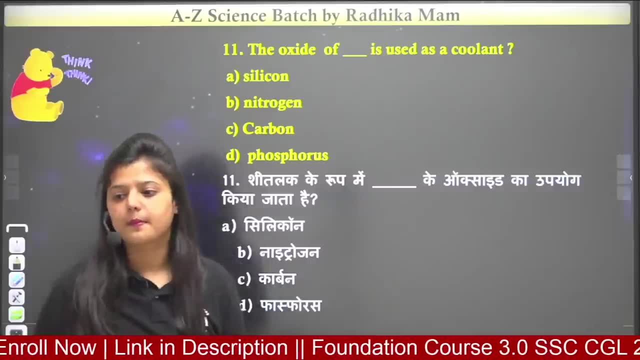 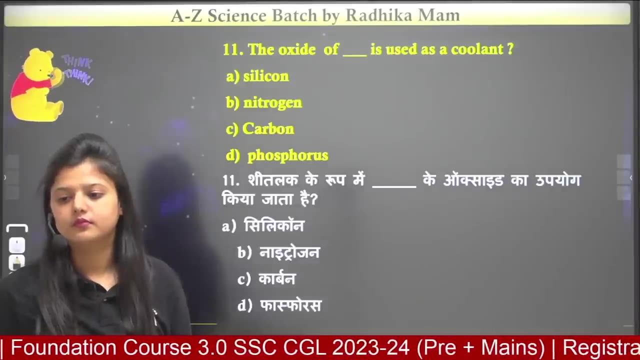 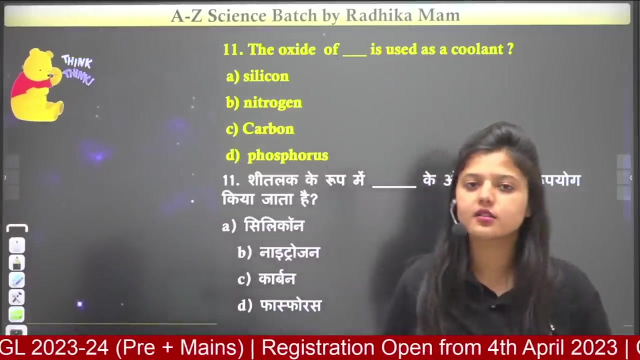 nitrogen, carbon or phosphorus As a coolant? What kind of oxide is used as a coolant here? which oxide is used as a coolant here? Okay, you will attend the marathon on Saturday, Friday, Tuesday and Saturday. You have to attend your paper on 2nd of MTS. it will be helpful for you all. 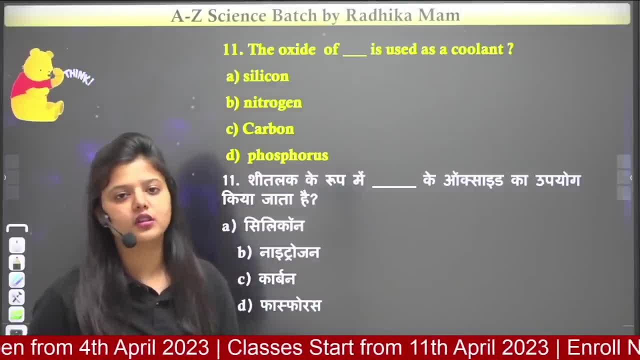 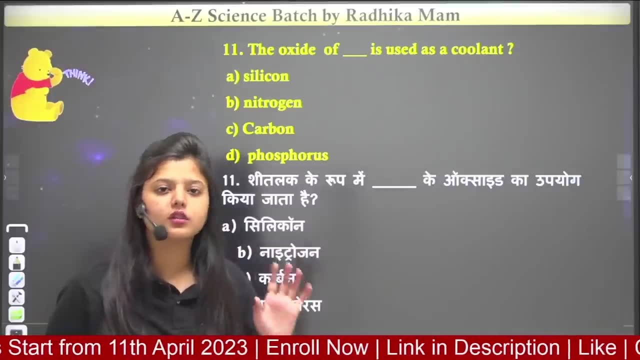 The rest of the regular sessions are going on. keep doing your revision And I will say this to you: keep applying all the mistakes in your important mock test. revision of those mistakes, That's it. their revision is mandatory because you must have read the theory to every extent. 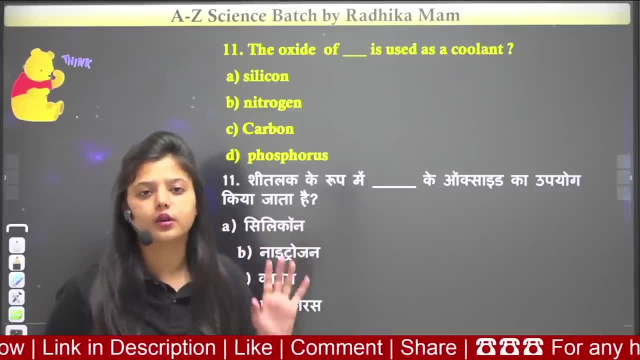 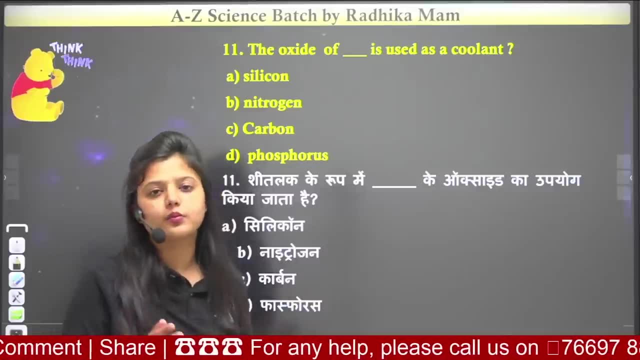 Now the point is what you are doing wrong. catch the wrong and pick up its theory. When this comes before the exam, then this work helps you a lot in those close moments. You start applying the test for a month and if you do not analyze the test, 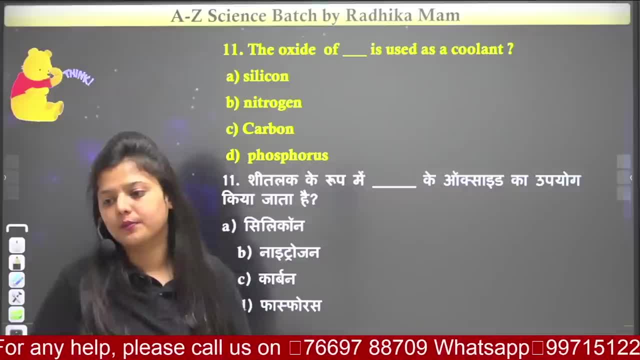 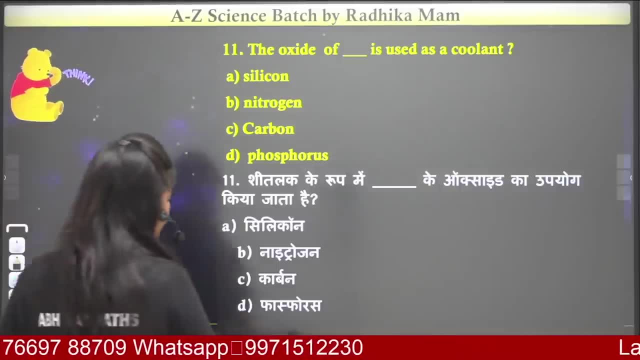 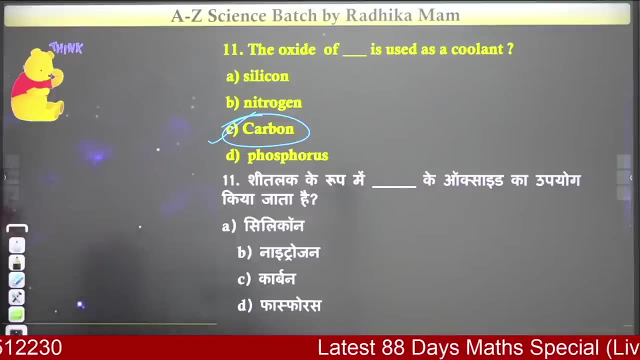 if there are no errors in it, then what is the benefit? Okay, Very good. Whose oxide works? The oxide of carbon works as a coolant. The oxide of carbon is seen to be working here. Next question: this is not an allotrope of carbon. 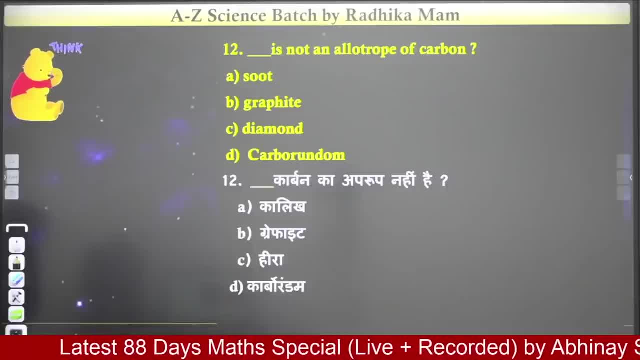 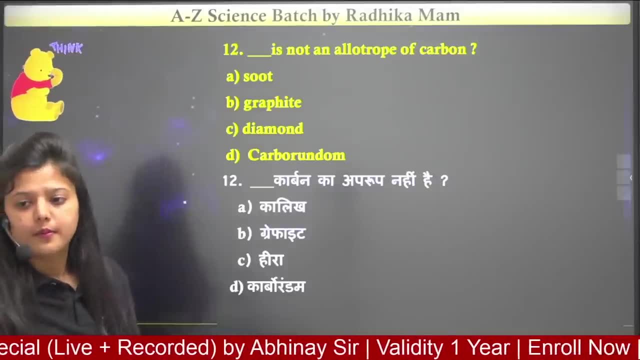 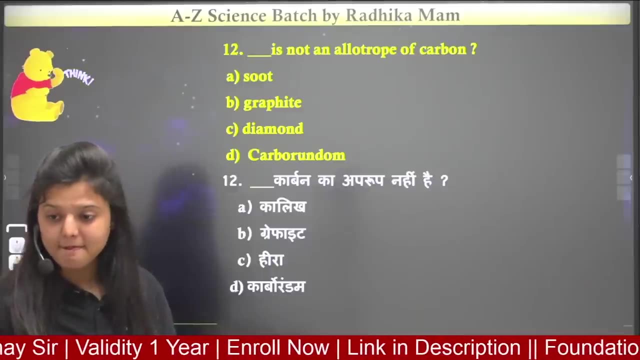 Which carbon does not have an allotrope here? Which carbon does not have an allotrope here? Tell me quickly, We will answer quickly. Which carbon does not have an allotrope. Can there be a simpler question than this, ma'am? 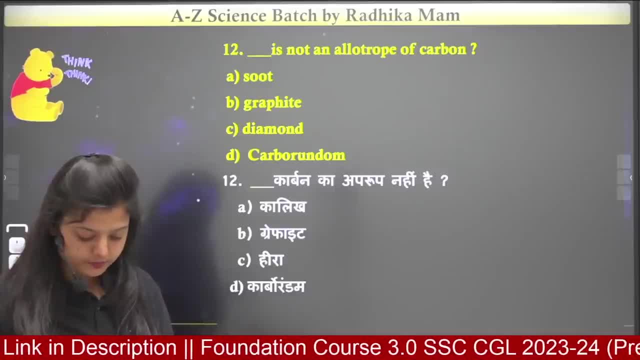 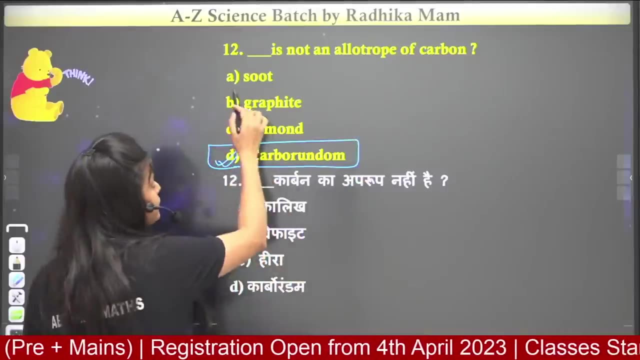 In which you are doing so much mess? Which carbon does not have an allotrope D? Let's go. What is this, ma'am Carborandum? Okay, This is not an allotrope of carbon. Let's talk about the suit: graphite diamond. 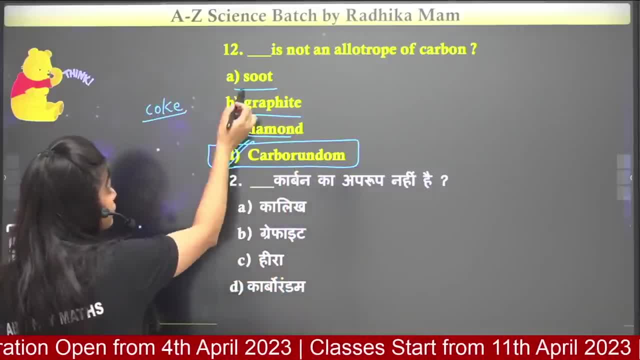 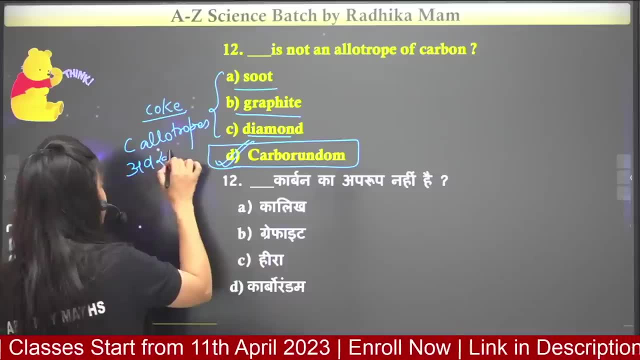 These are all. Cog can be seen Charcoal suit. These are all the allotropes of carbon. That is the allotrope of carbon, The allotrope of carbon. If I talk about the carborandum here, then this is silicon carbide. 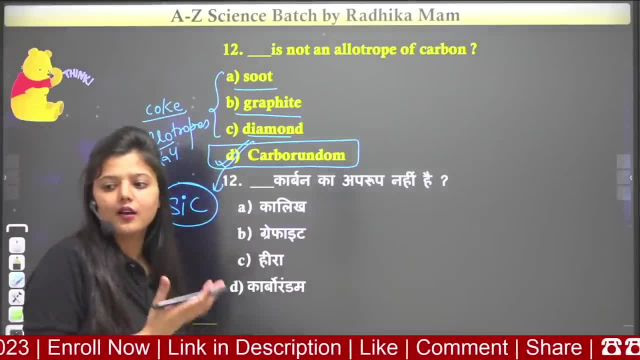 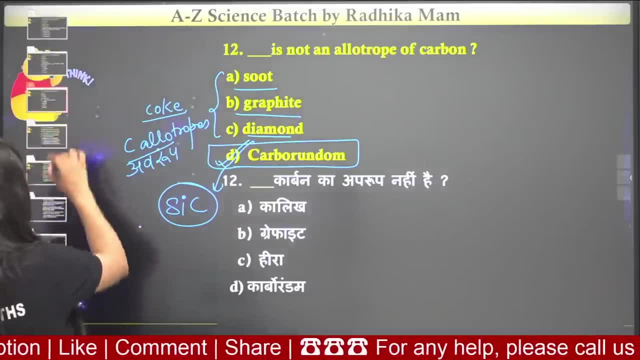 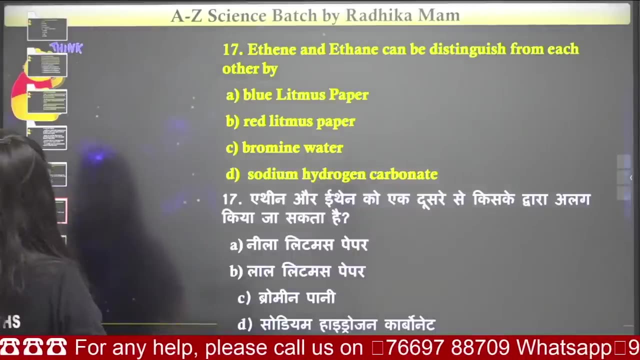 This is different. here The allotrope of carbon is not found. here We do not get to see the allotrope of carbon. Let's see the next question. Next question says what happens in covalent compounds. Covalent compounds have high melting and boiling point. 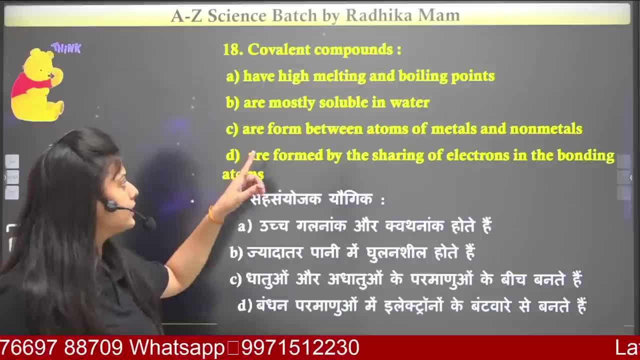 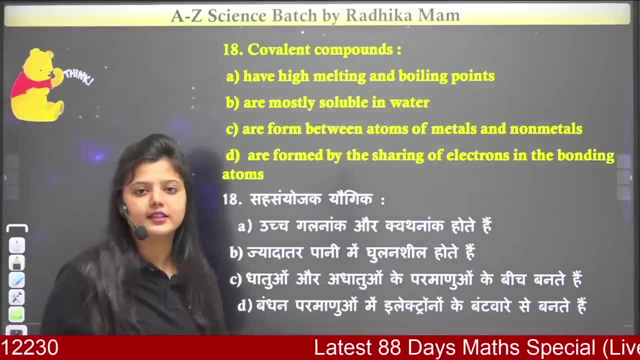 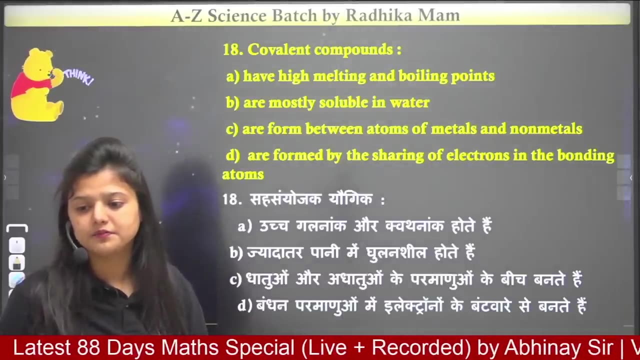 They are soluble in water. They are soluble in water. They are formed between atoms of metal and non-metals, Or they are formed between the sharing of electrons. What is your tolerable answer? Everyone's answer is understandable. Everyone's answer is understandable. 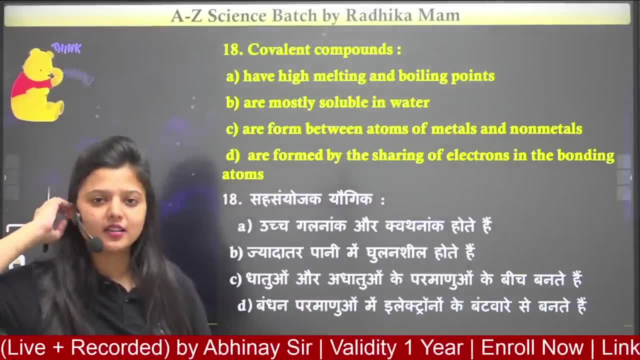 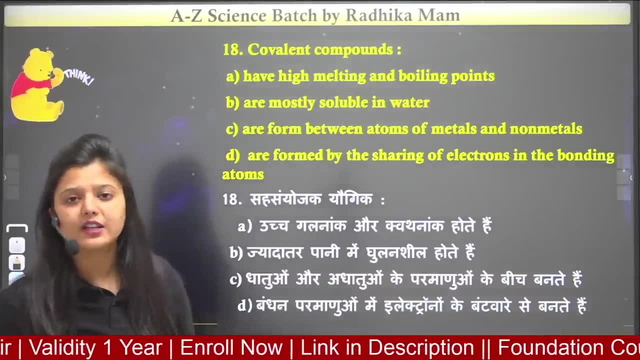 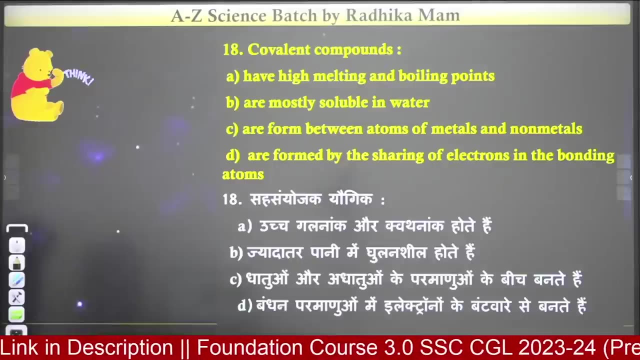 Which is the answer. You always have to work with eher fragile Scripture that talks about the covalent côngustibles, Not just the covalent one. the covalent covalent comes in various forms, Not just covalent: the covalent, whole covalent. 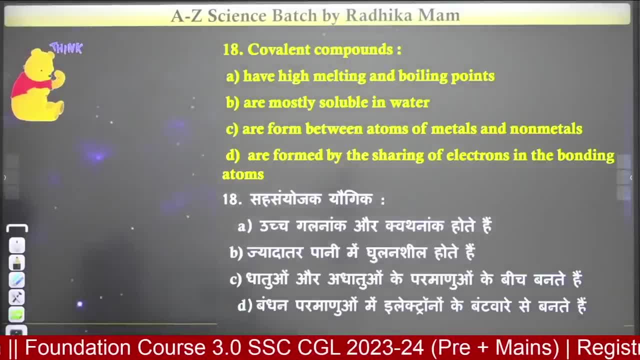 This is everywhere, And we should say that foi covalent covalent, Not just covalent, but covalent covalent is Frost. I will forgive you for me哪 Really burn by. Would you fire nigra covalent covalent? 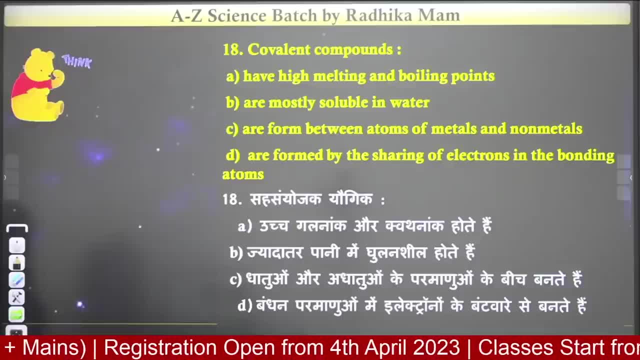 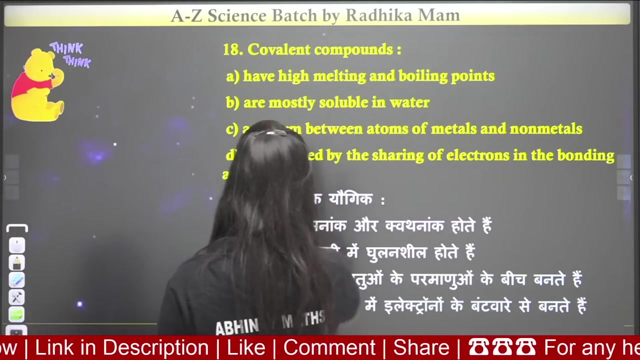 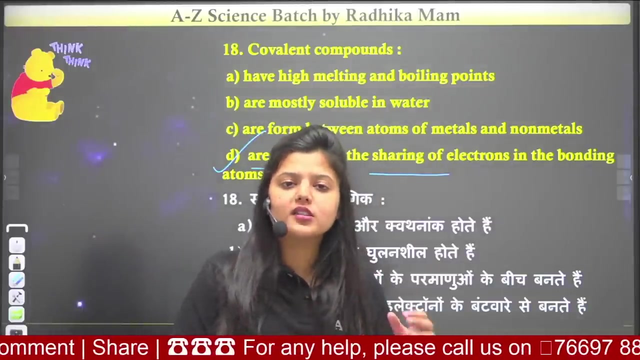 correct answer. kya ho jayega? they are formed by the sharing of electrons in the bonding atom. I mean, I don't have to think, ma'am, Our option d will be correct If there is a transfer of metals in non-metals. you are seeing that, brother, if there was a 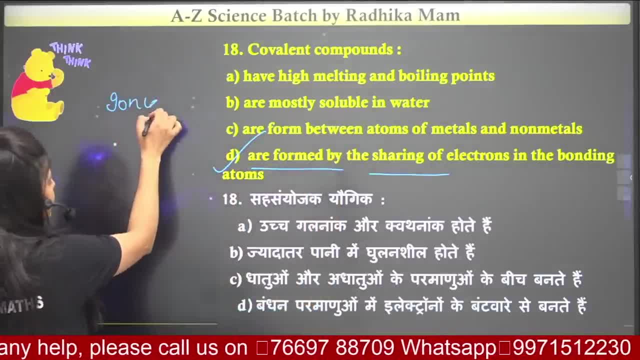 transfer here. then we say that an ionic bond would have been formed. So what do we say? Ionic bond would have been formed. Neither would they be soluble in water, nor would their high melting boiling point be there. they would have been less. 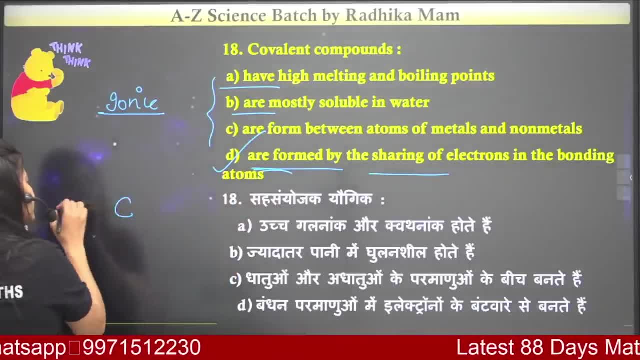 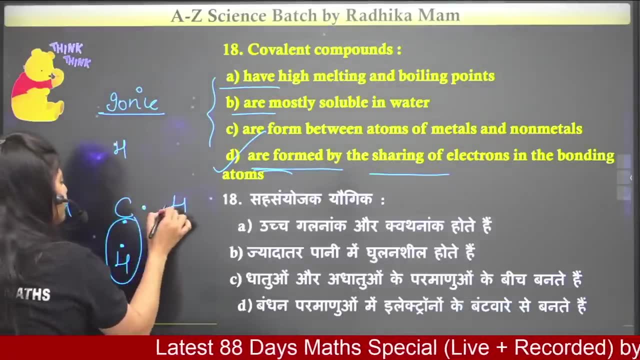 These properties are given the ionic one. What we are seeing is that if four hydrogen is visible along with carbon, then what will all four of us do? We start making our bonding here, And it is said that if the four hydrogen is visible along with carbon, then what will? 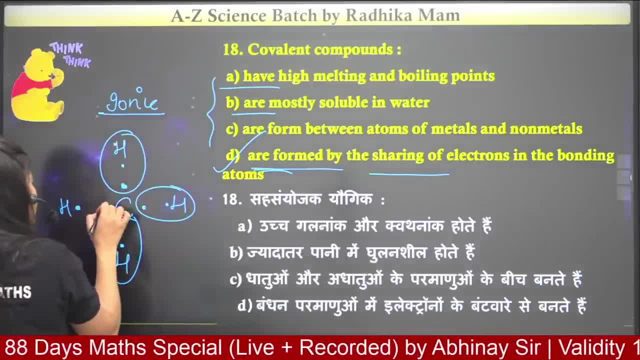 happen. Well, the one thing I do is that if it is visible along with carbon, then this is the bondage, But if the bondage is one turn, then it is considered to be an ionic, So this is called shattering of electrons. 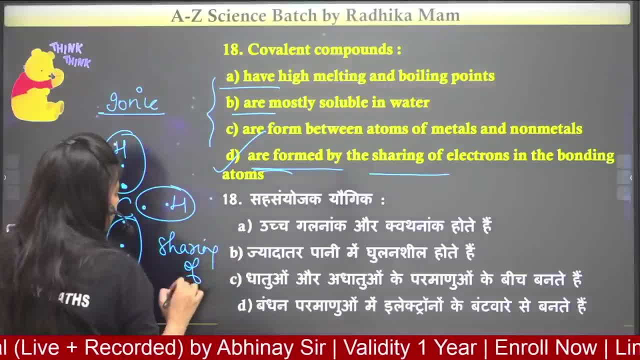 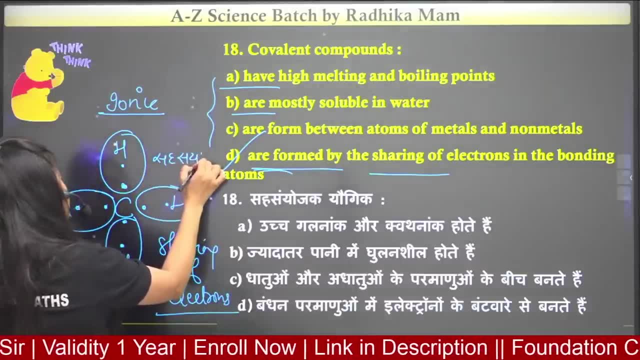 In some way our methane is made, and it is made by the sharing of electrons, and when such bonds are formed, then it becomes co-operative binding. If I tell you that nitrogen is being formed, ok, then it is becoming n2, then tell me: is? 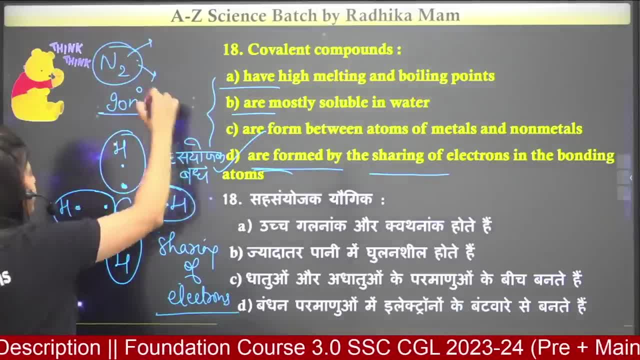 it an ionic compound or a covalent compound? How does the bondage between a molecule of nitrogen being formed feel? So this is a covalent compound and this is a covalent compound. So it is a covalent compound. 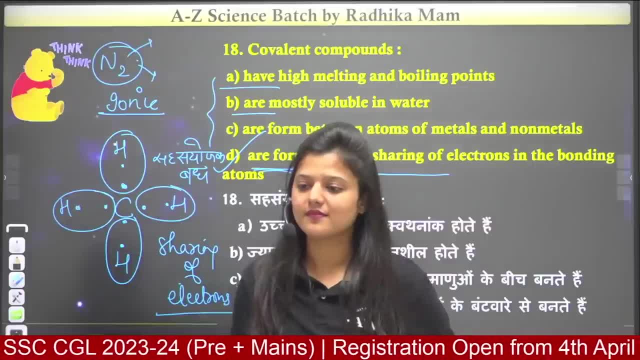 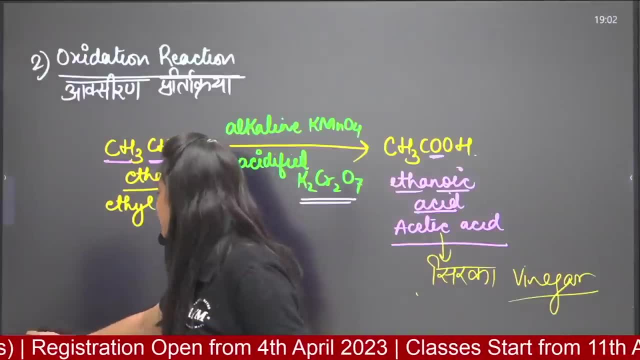 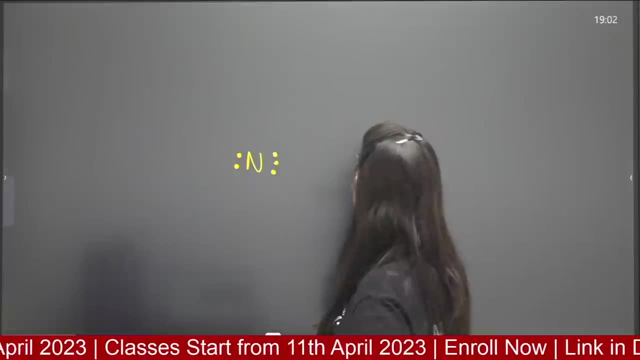 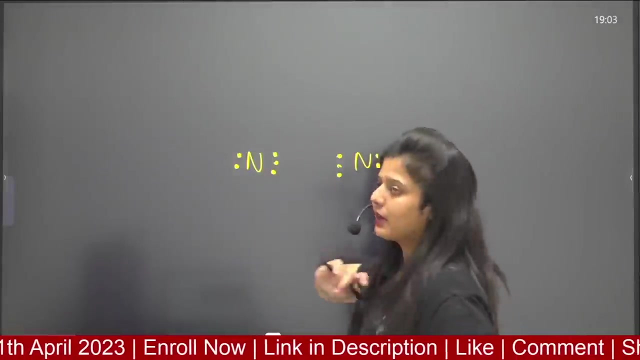 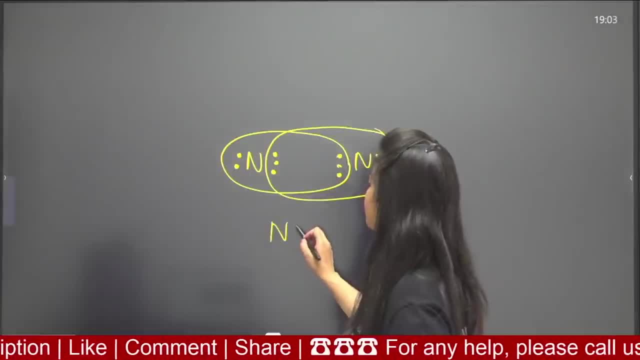 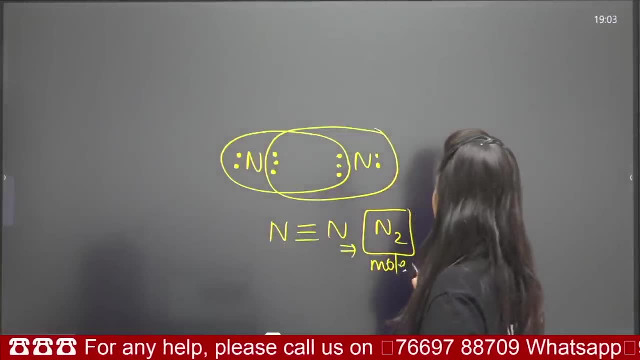 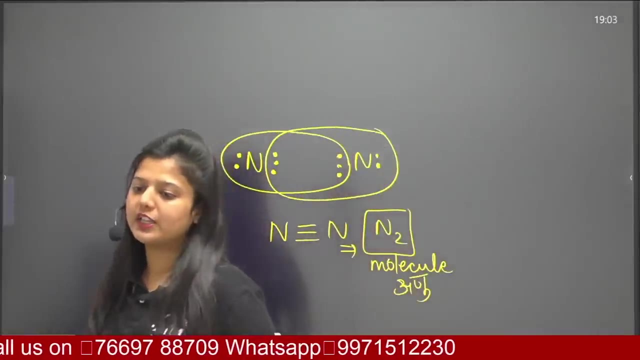 Then the third one also does it in this way because 3 electrons are sharing. so here it goes. here, triple bond, and it becomes a molecule of nitrogen. alright, molecule, a molecule of nitrogen. how did it become? Covalent bonding? with covalent bonding, these bonds which are coming inside it, these are hydrogen bonds, these are hydrogen. how do they become? 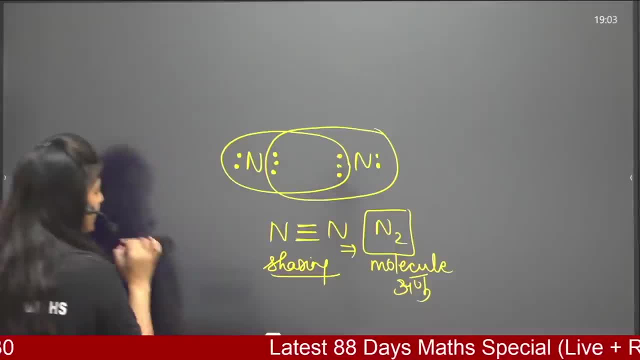 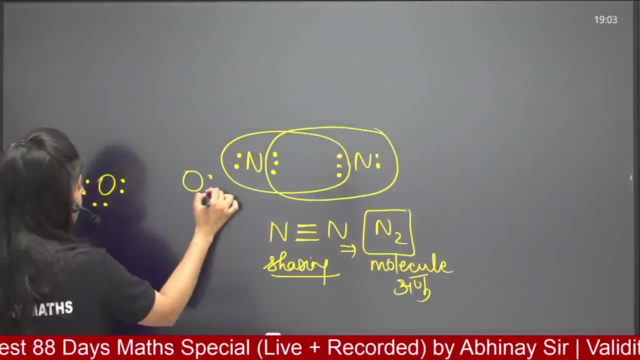 In the same way, if I talk about oxygen, then we can see that oxygen has 6, 1,, 2, 3,, 4,, 5, 6.. Now, what will it do with 6?? It took 2 from here and took 2 from here. 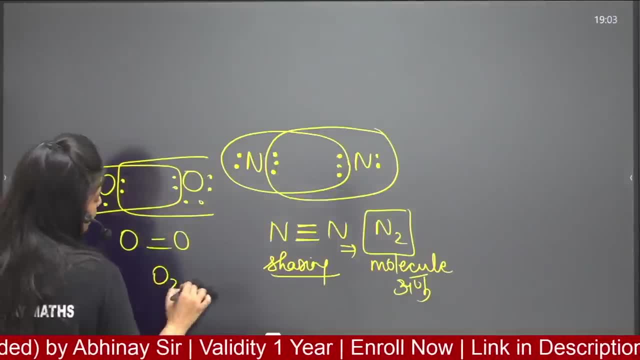 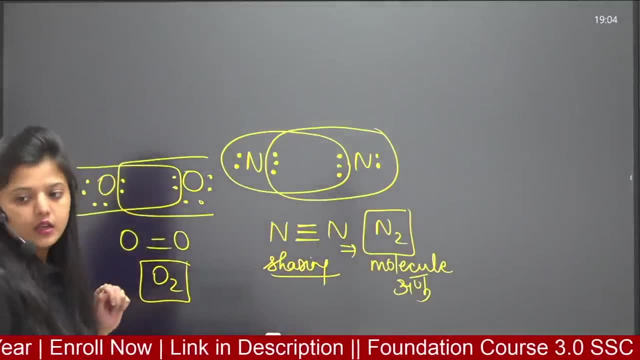 What happened to it? 8 were completed O double bond. this became O2.. What do we call all of them? They are getting ready to be our covalent compounds. All bonds have to be made of love, right? Make some compounds here too. 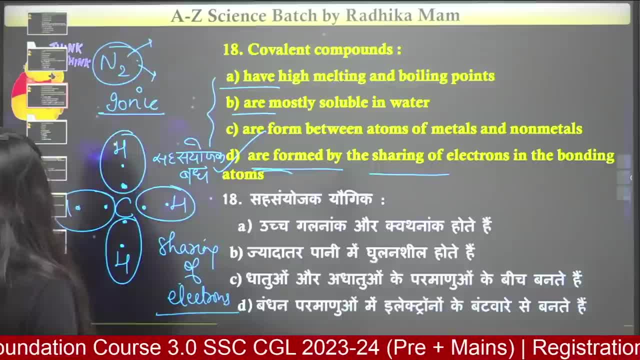 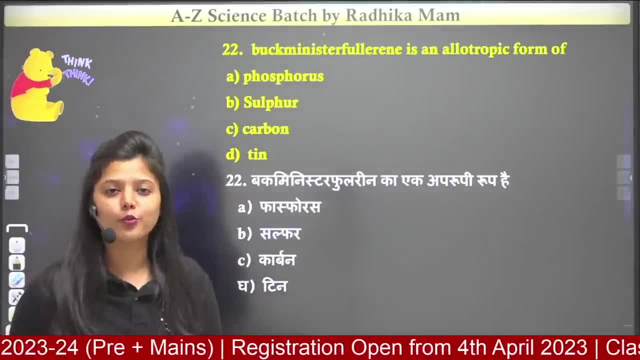 Bond of love. Next question: Buckminster fulrine is an allotropic form of phosphorus, sulfur, carbon or tin. Whose allotropic form is Buckminster fulrine? Look, madam, I have read the new chapter. now I will correct the answer. 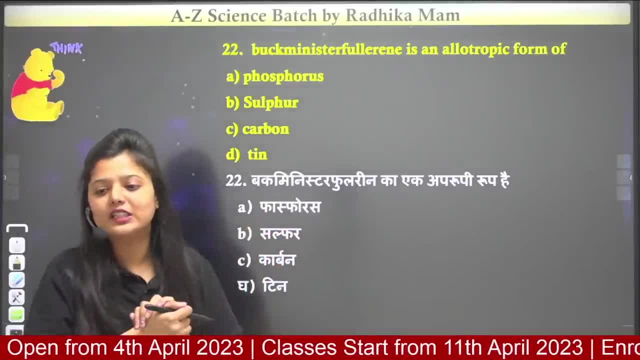 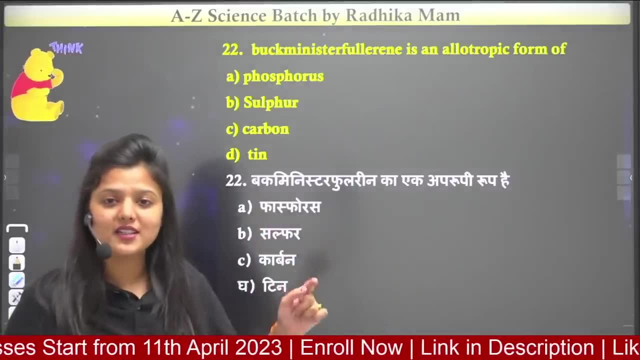 I don't know this big name, Buckminster fulrine- while reaching the exam. whether I remember or not, The same questions come in the exam. For now. you will remember that the good ma'am told 3. Diamond graphite: C60 means Buckminster fulrine. 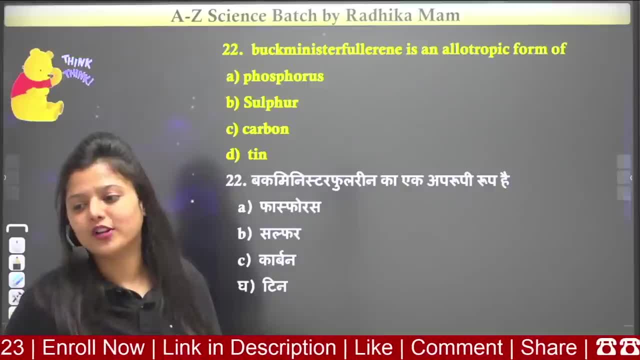 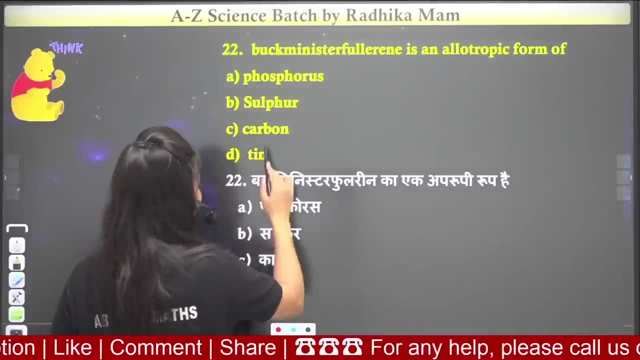 Now. do you remember now? How much do you remember later? This is important. This is important to you. That is why it is said to attend chemistry class at 6 pm daily. At least your revision will continue. Answer is carbon. 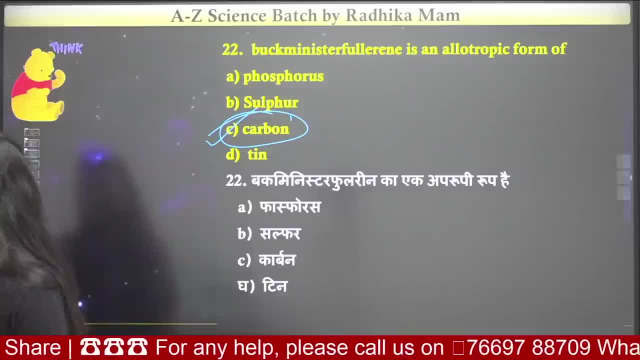 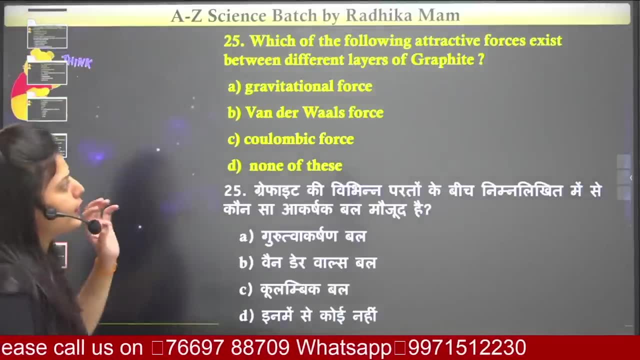 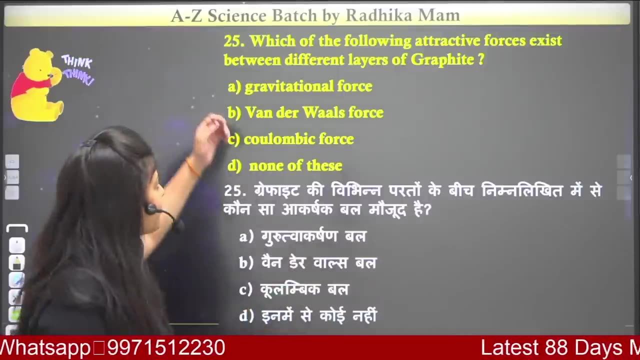 What will happen? The right answer for carbon will be here. The next question is saying that: tell me which of the following attractive forces exist between different layers of graphite. I said that many layers of graphite are visible. There are van der waals forces, coulombic forces, gravitational forces, and none of these forces are visible. 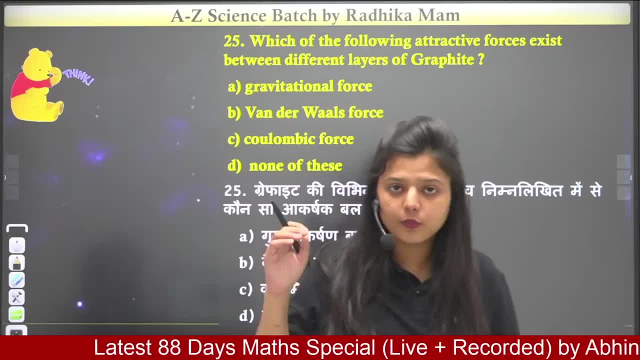 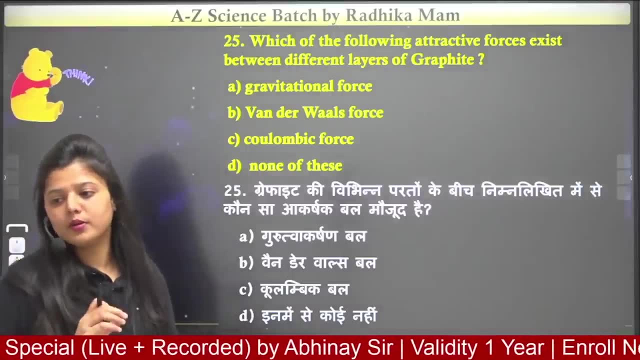 Everyone is having fun in questioning: Are all the points being clear or not? And if they are, then keep sharing and, like this session, Do this work quickly, Ma'am. this is also the case in mock. That's why I said you will forget while coming to mock. 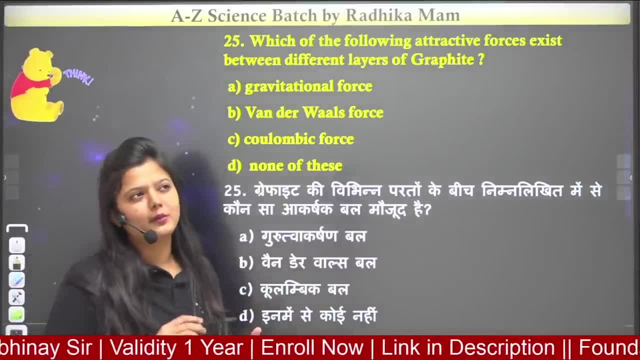 You will apply after 15 days. till then you will think that now I have studied metallurgy. I have read many names of aluminium. Now with whom should I compare this buckminster fullerene? I must have read hematite and magnetite. 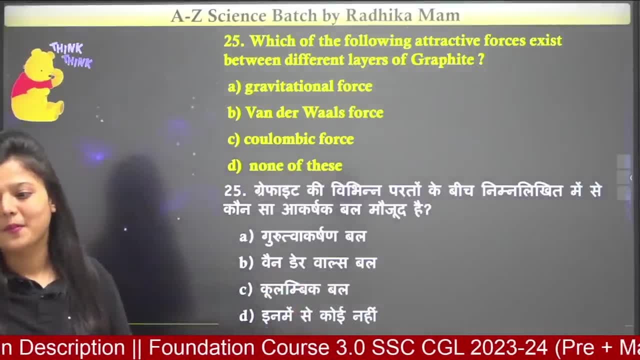 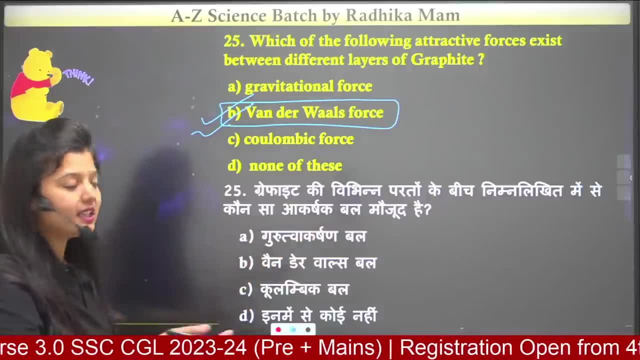 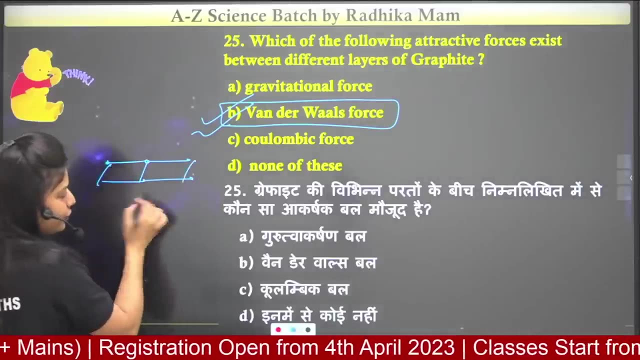 Many things come to mind. then These are the weak van der waals forces. Okay, actually they are weak forces. That is why the different layers that you see in graphite. you see these layers slipping on each other, Because what is the force between them? 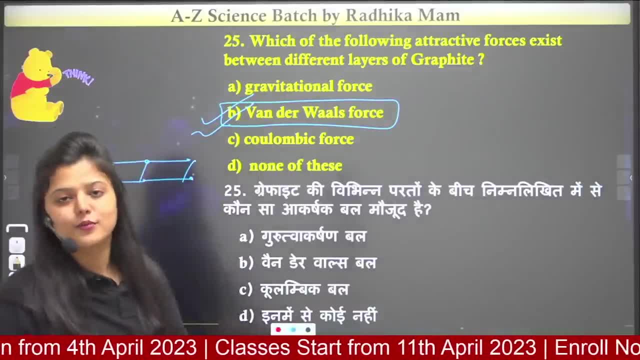 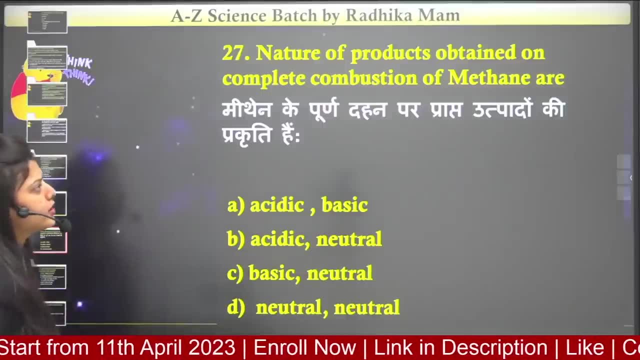 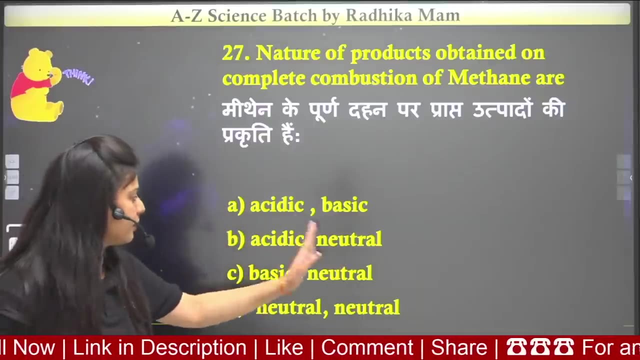 It looks very weak, Weak. We call it weak forces. The next question is Nature of products obtained on complete combustion of methane. If you are considering the content of methane, then how will the products be made? Acidic and basic, basic and neutral. 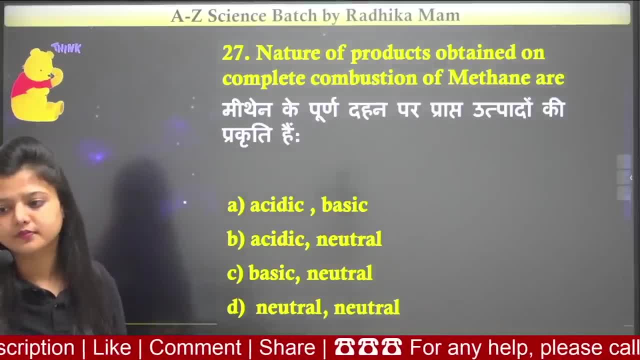 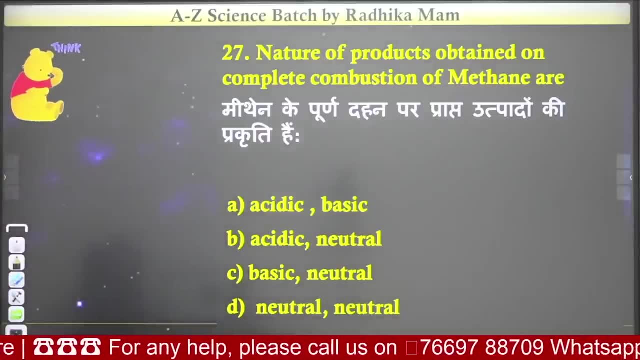 or what property will they have? Tell me quickly, Quickly, we will give the answer. This is what we had to think, ma'am. This is what we had to think, Acidic and neutral. Okay, tell me one thing. We were doing the reaction just now. 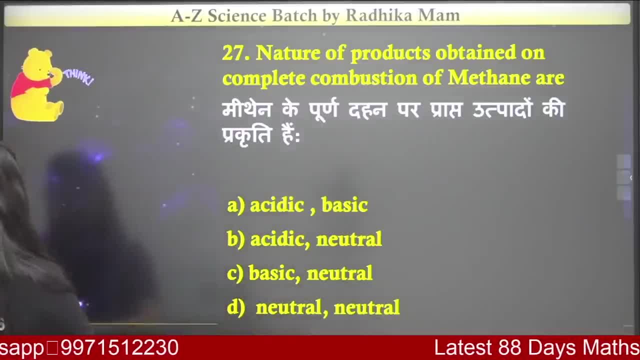 What was the reaction? Ma'am, we had done the combustion. Let's see where we did it. You did the combustion, Okay, You said, here is the methane. And I burnt the methane. What did you make? You made CO2, you made H2O, you made heat, you made light. 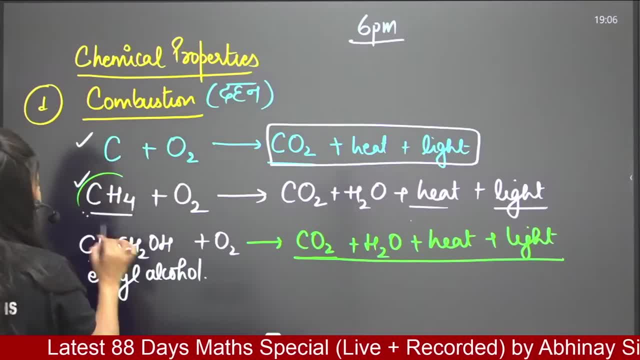 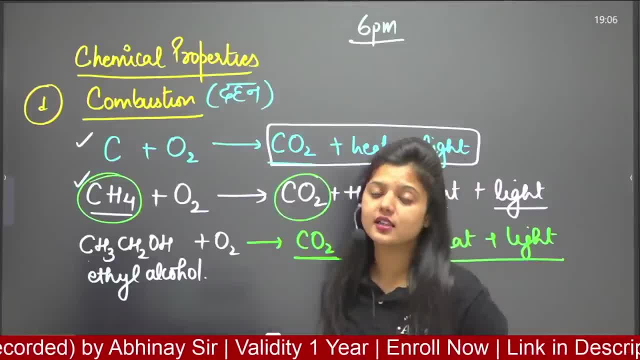 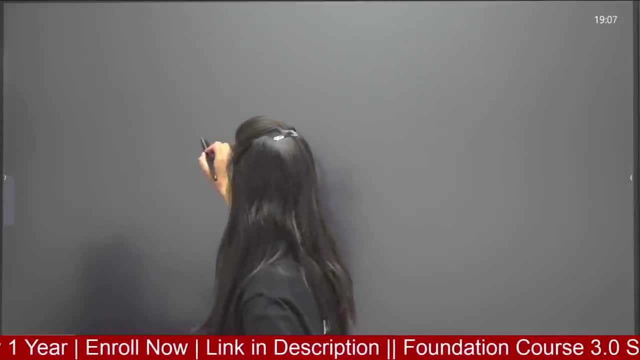 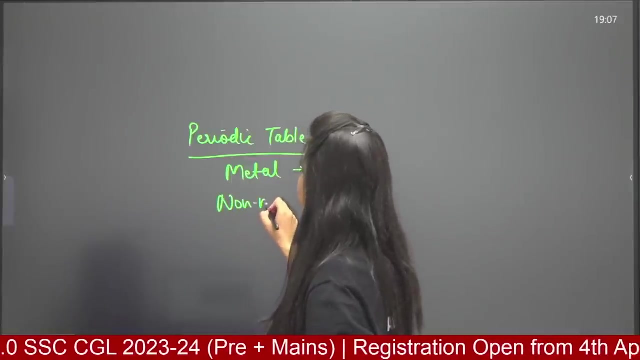 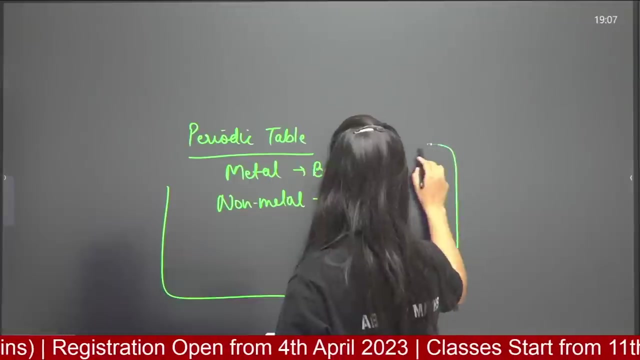 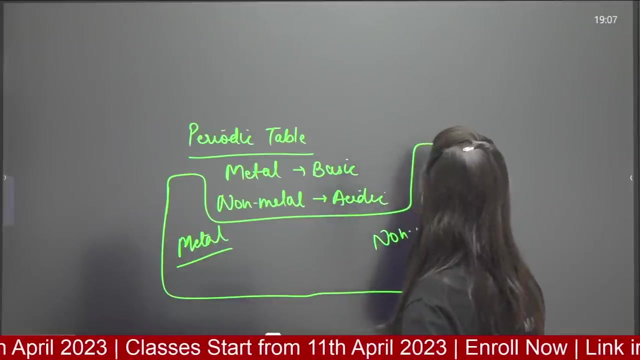 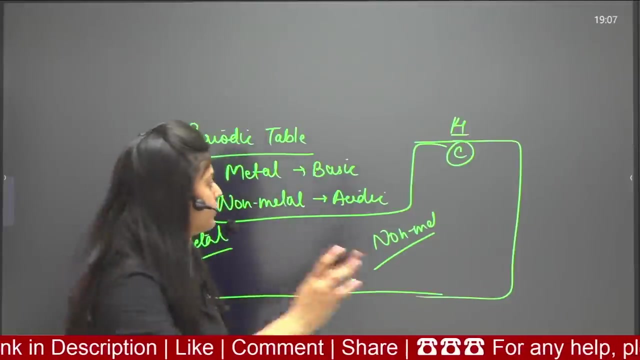 Is it carbon dioxide? Is it carbon dioxide? Is it carbon dioxide? Do you call it neutrality disequ comedy? Do you consider it aa? Why not? Okay, Okay, Okay. On the left side we had all the metals. they were making basic oxide. if you come this way, then, madam, was non-metal, they were making acidic oxide. and here somewhere in my group, number 14, carbon is visible. so even if I have not read anything, then can I tell or not tell that madam? tell me one thing: this was carbon and carbon was made non-metal. and if this oxide is making CO2, then will this be acidic or not? 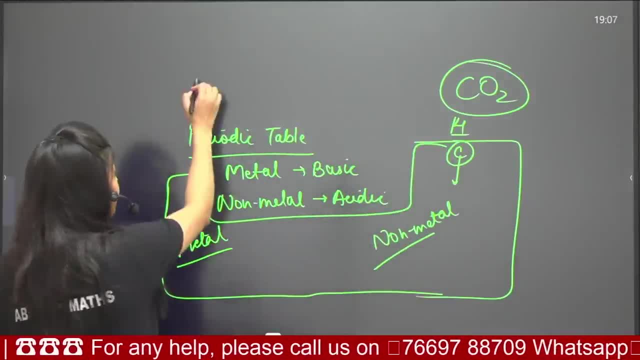 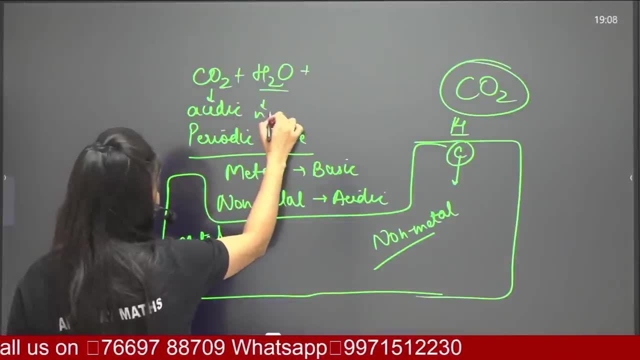 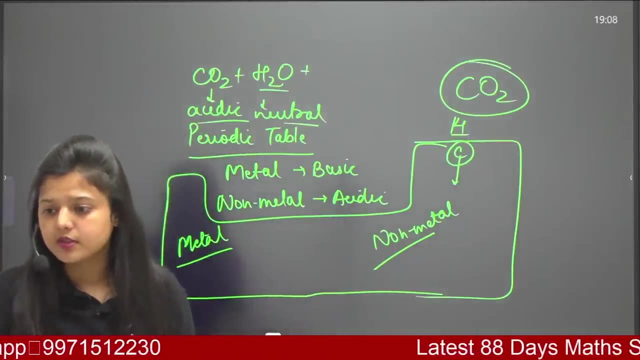 water is neutral, then what did you make? CO2, water took out the heat light separately. this is acidic and this is neutral. what answer will you give? all the basics we were putting. come quickly and tell me. this series is very important for us. thank you very much. you are good for everyone and quickly take your selection, okay. 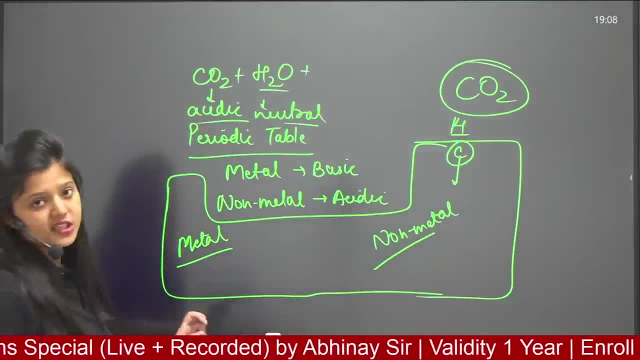 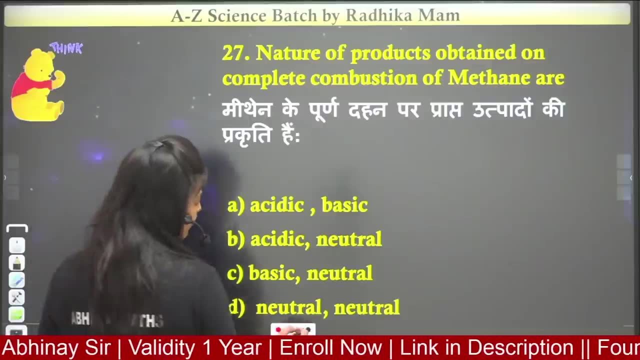 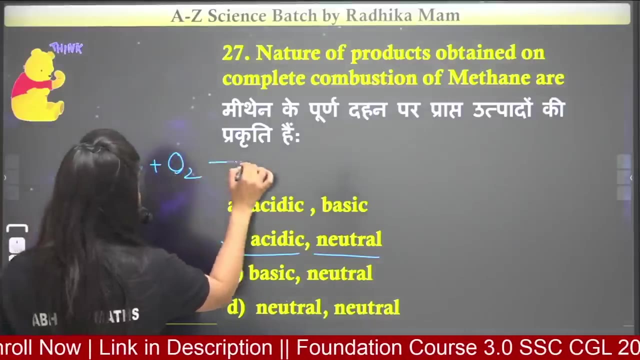 okay, okay, okay, okay. I will put it in detail. When we talk about physics, then we will talk about all the forces there. then what will be the answer? here? you will put: one is acidic and the other is neutral. now someone has a problem in it. you have made a complete combustion of methane. and what has been made? some have been prepared by making a product in this way. 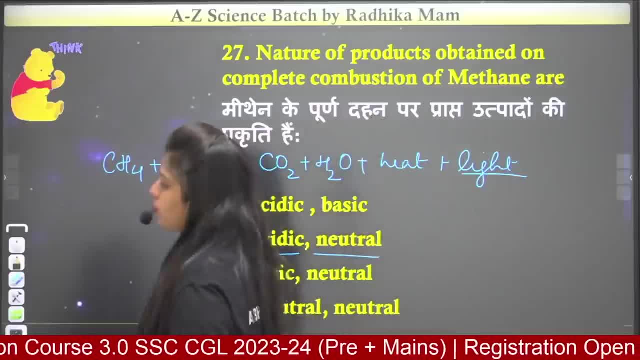 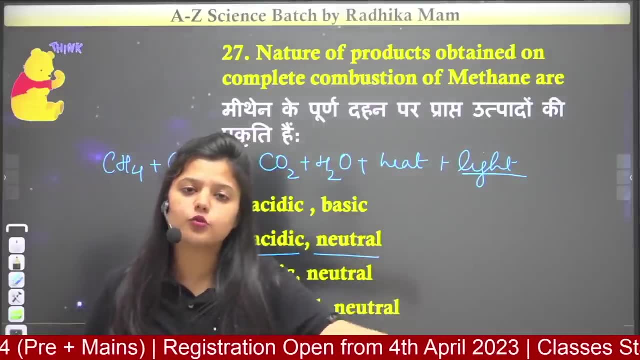 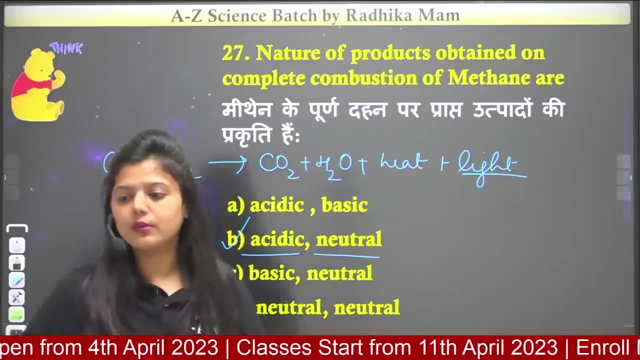 Tell me, the oxide of metals will always be made. it will be basic. so we are not taking metals here. but if we take lithium and say that we have to make the oxide of sodium and lithium, then you say that the basic oxide will be made. now you have carbon, so this will make basic, not acidic oxide, acidic oxide. 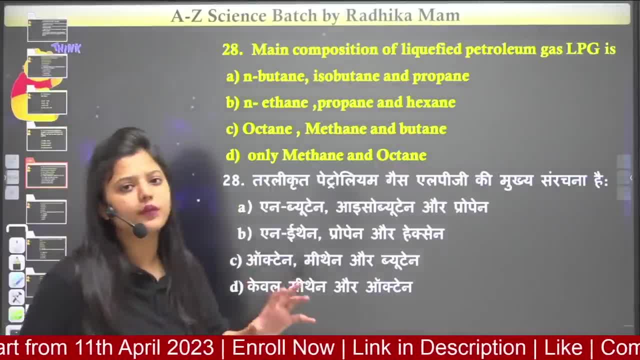 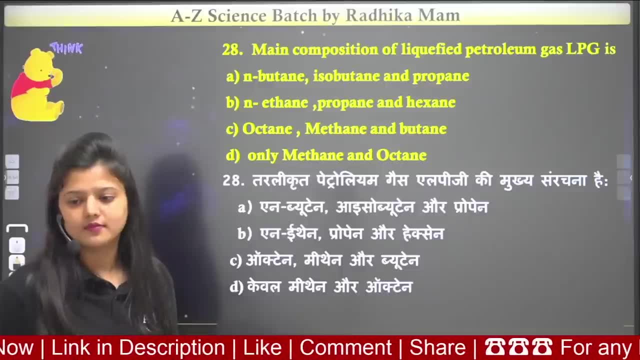 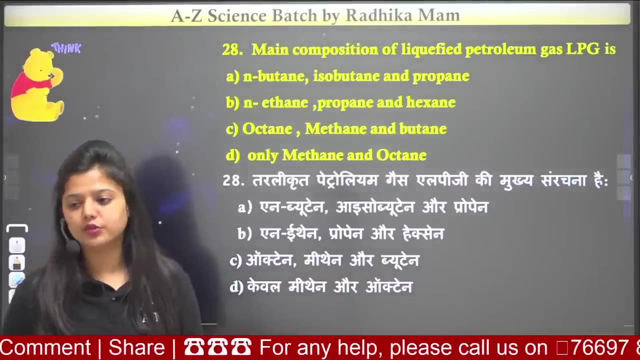 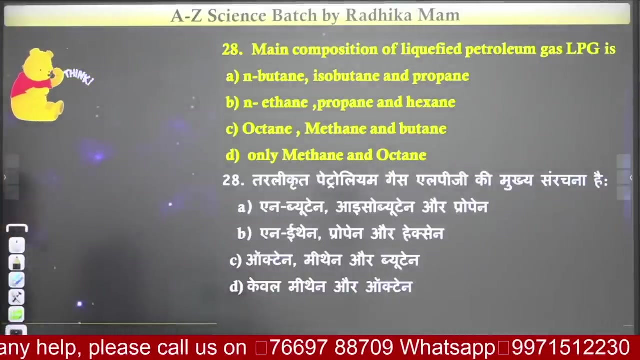 The next one is saying: tell me the main reduction of LPG, what is mainly seen in liquefied petroleum gas, What is mainly seen in liquefied petroleum gas? Tell me quickly. we will tell you quickly. LPG, liquefied petroleum gas, n-butane, isobutane and propane, ethane, propane, hexane, octane, methane and butane or only methane and octane will be here. what things are present in your case? 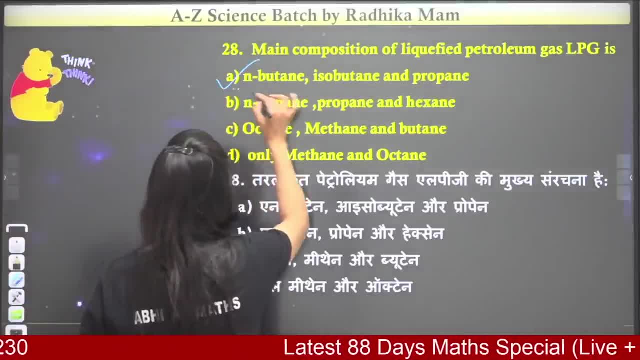 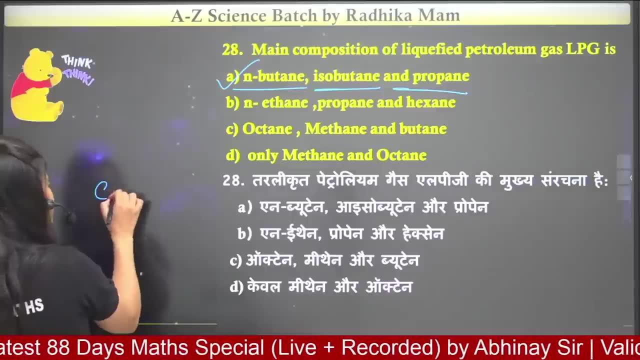 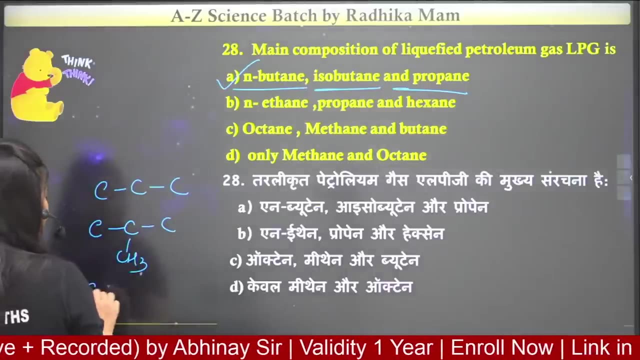 Very good, you are talking about LPG, right? LPG N-butane, isobutane and propane. one will be normal butane, one will be isobutane and one will be propane. If you say propane, then you can see three carbons and isobutane is done. and if we are talking about normal butane, then this is your normal butane. 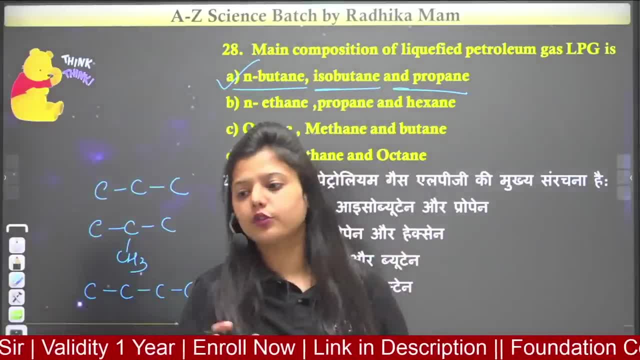 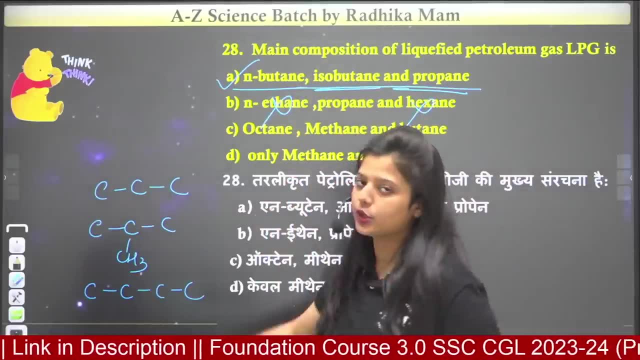 These three things are present in LPG. liquefied petroleum gas. A is the right answer. ethane is not there. neither hexane is there, neither ethane is there. If I talk about CNG here, Let me talk about CNG- compressed natural gas. 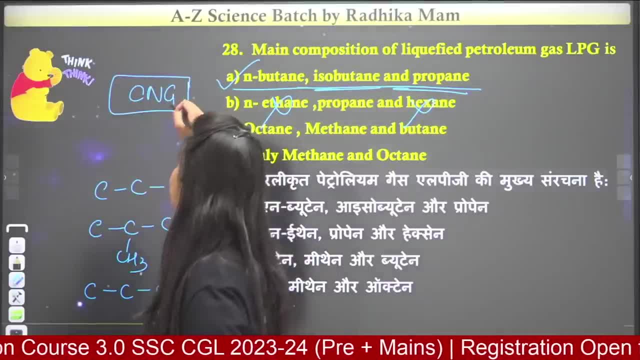 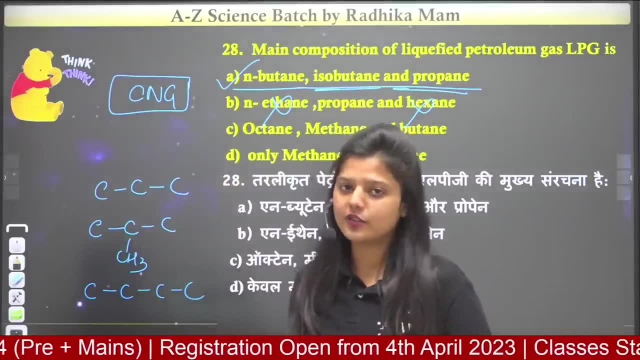 Tell me what is compressed natural gas. how much methane is there in it? Who is answering? N-butane means normal butane. One is the iso position. iso means I put a methyl group and put it back here, So that is iso. iso becomes a different chain. 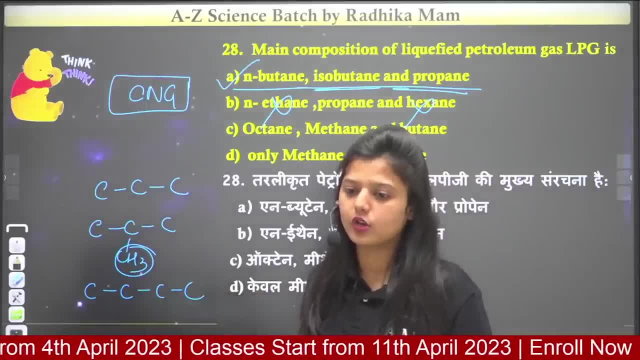 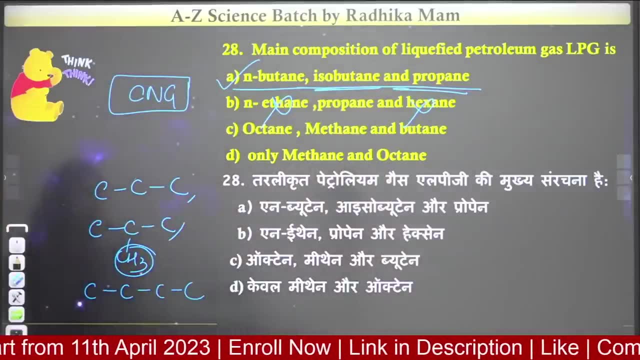 We have to remember the name. isobutane will be here and the rest is butane. this is isobutane and this is propane. Okay, N-butane was given right. Yes, I will talk about CNG, brother. what is there in CNG? 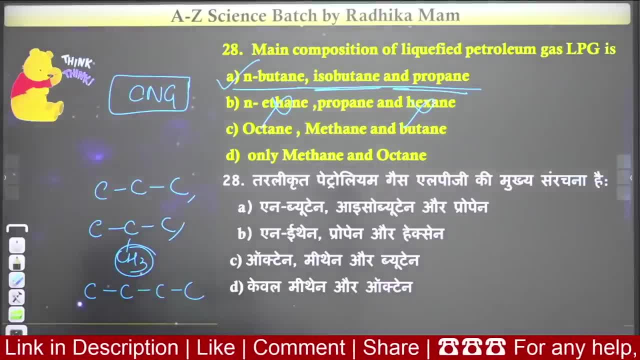 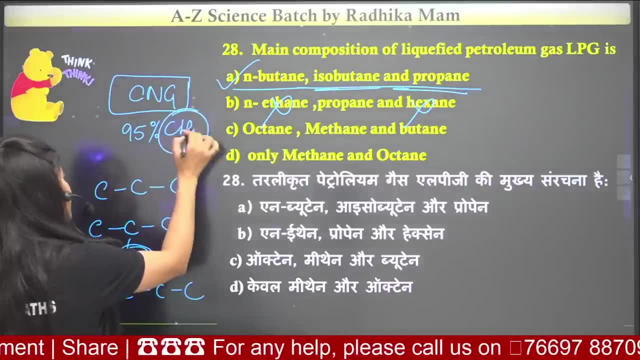 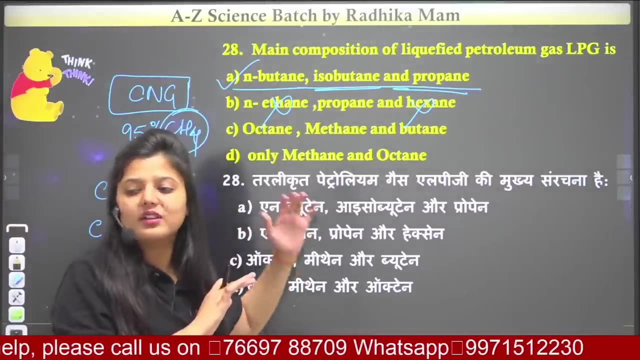 Very good, 95%, around right CH4.. Ultimately, methane is present here. Natural gas means methane. What did you do to methane? Compressed it and compressed it. it became compressed natural gas. What do you see? around 80%, 90%. 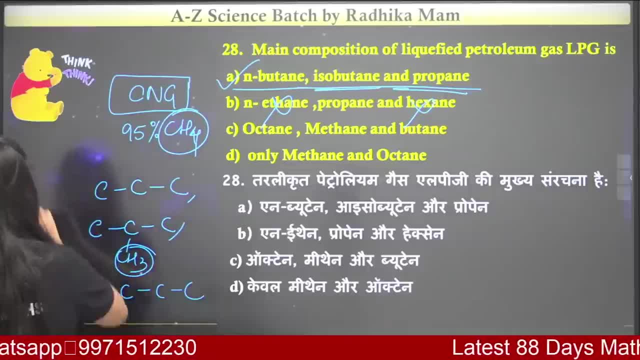 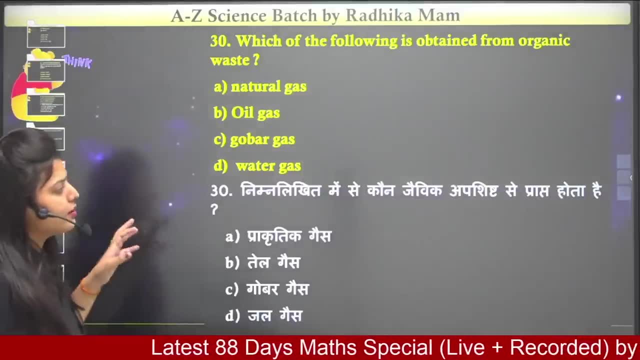 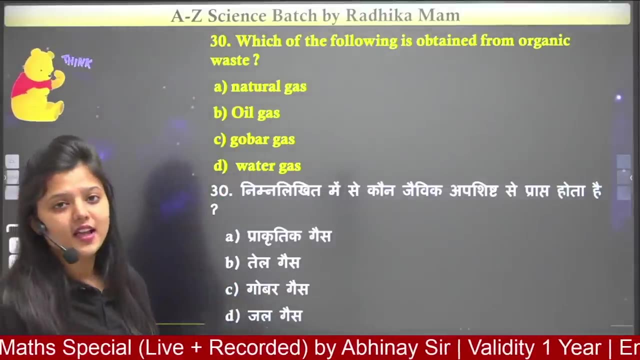 CH4 is shown here. I hope this is clear. I hope this is clear. The next one is saying which is obtained from organic waste. What can you take from the organic waste- Natural gas, oil gas, cow dung gas or water gas? 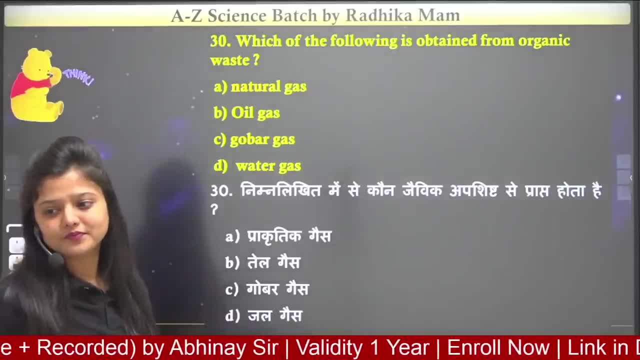 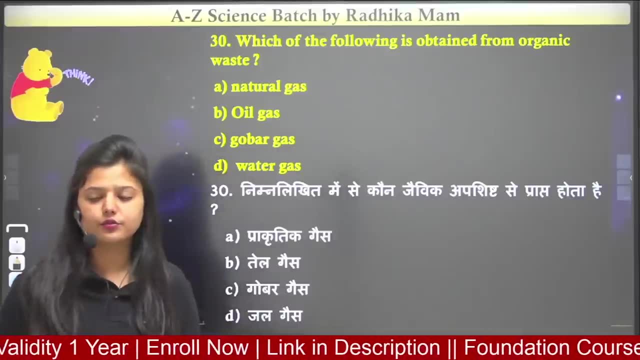 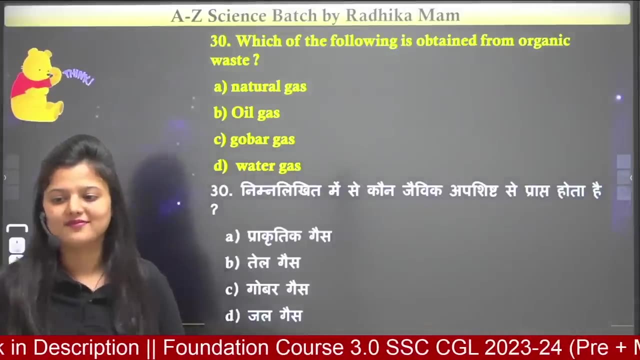 What can you make from organic waste? Quickly, When is the last day of chemistry? Read this week again. we will start physics from Monday till Saturday. Okay, we will start physics from Monday. Read this week again: Natural oil, cow dung gas or water gas? 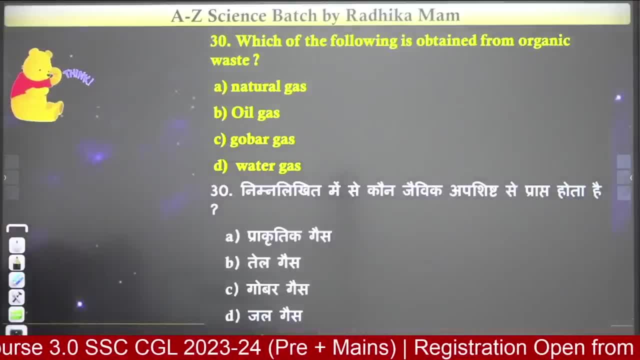 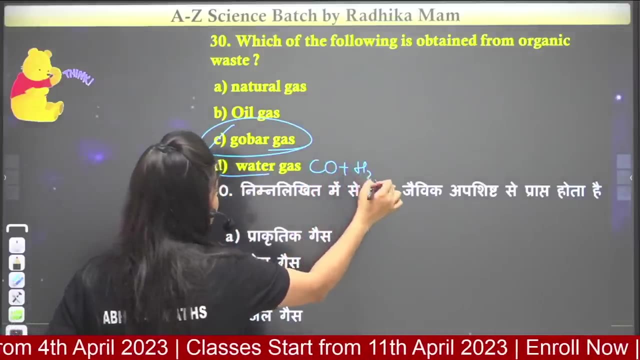 Very good. There is a chemical compound. let's make cow dung gas. Water gas will not be made Here. carbon monoxide plus H2 is there, so this will not be made. Cow dung gas. you will see it being made. 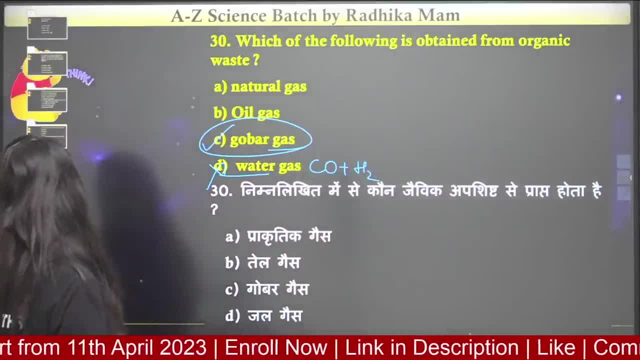 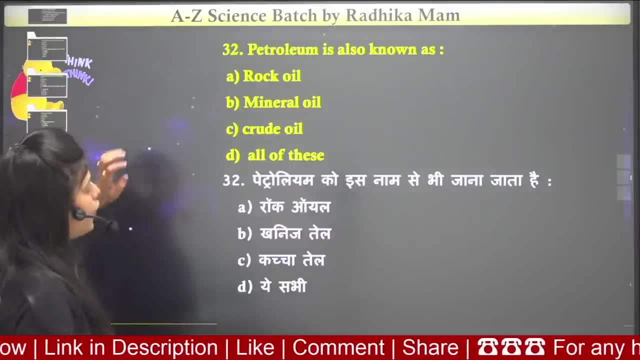 Very beautiful answer. With this, let's move ahead and come to our next question, which is saying to us what is the name of petroleum, Rock oil, mineral oil, crude oil or all of this Or all of this? Tell me quickly once. 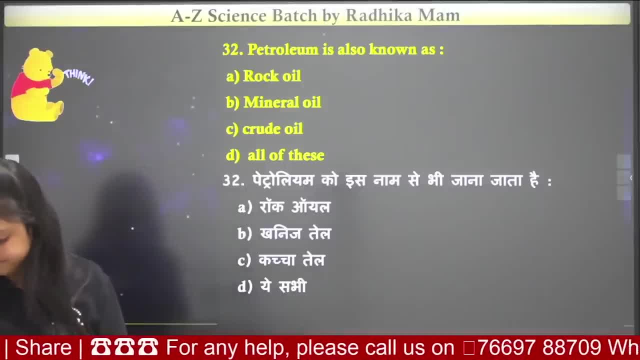 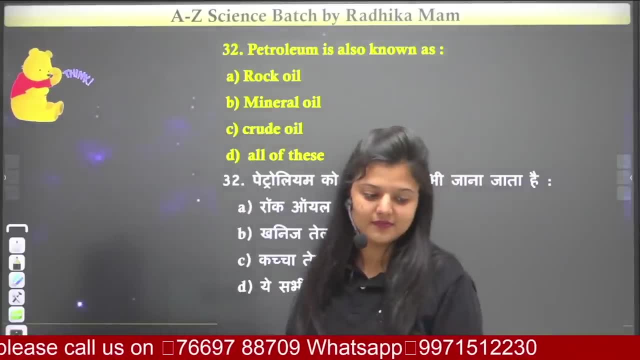 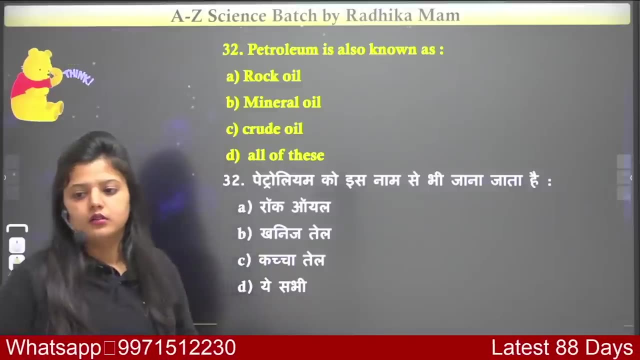 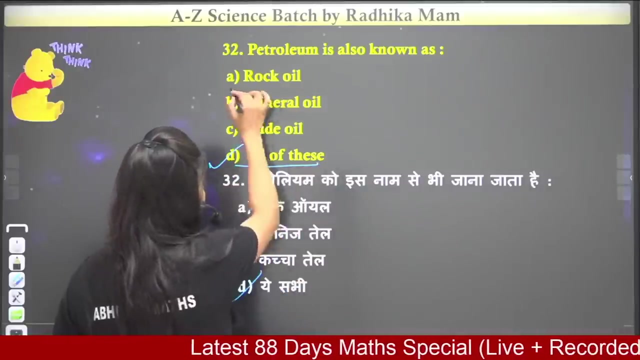 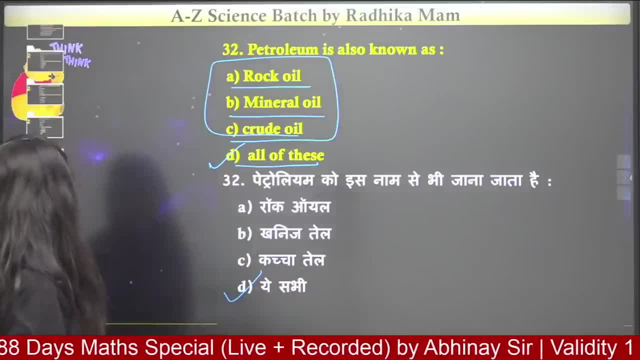 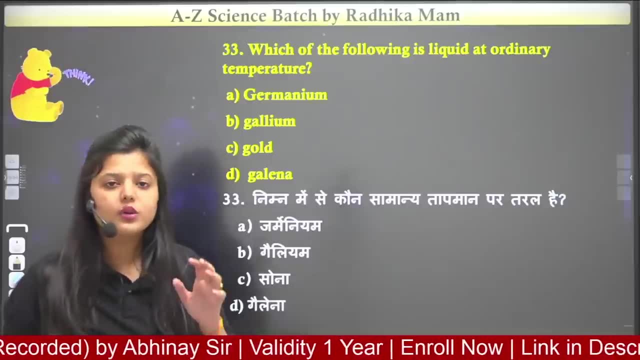 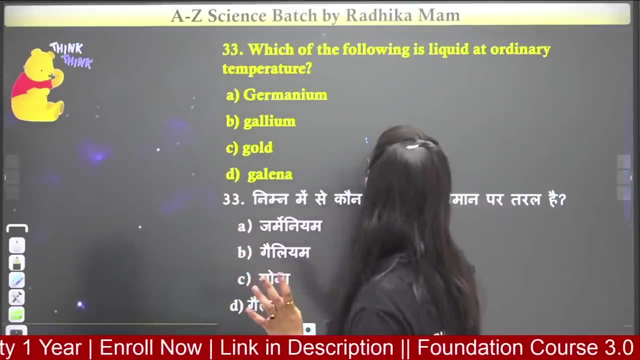 Petroleum is also known by these names. And next question, which you will tell me here: which of these things is liquid in the heat? Which metal is liquid at room temperature or ordinary temperature? This was your today's question. there was a homework question that you guys are telling me by commenting offline. 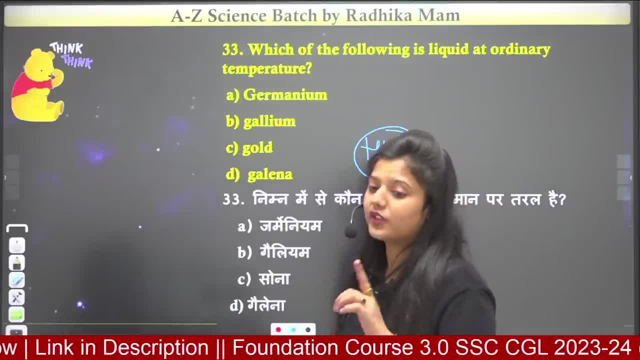 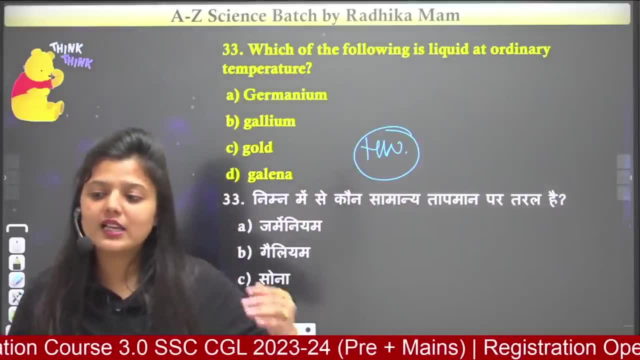 that what will be the correct answer for this? and don't think that ma'am doesn't look at offline comments. I look at all the answers of all your homework questions properly that who is telling the truth and who is not telling the truth. there are some who give us answers regularly and there are some who 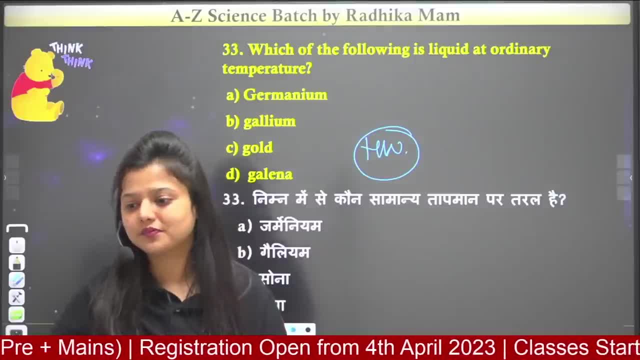 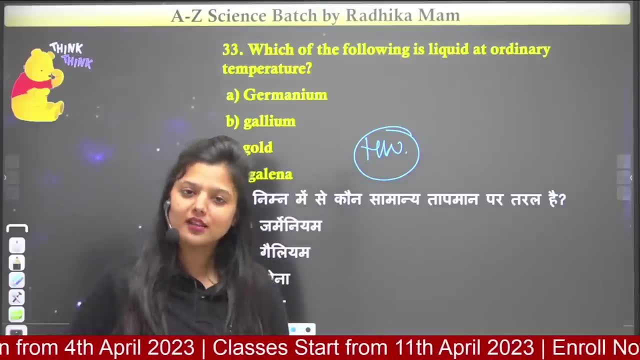 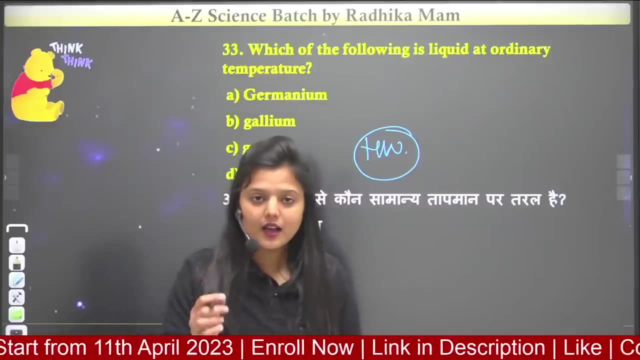 don't pay attention at all if I told you in the class. then I told you: okay, it's okay, read this science like this so that whatever exam you give ahead, you will be fruitful in all of them, Even if it takes time. but they say that, brother, if we just have to build a house, 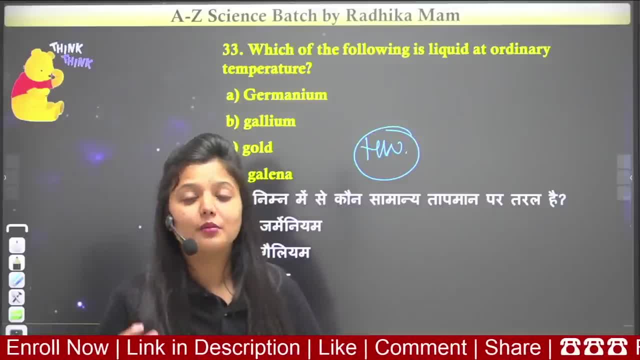 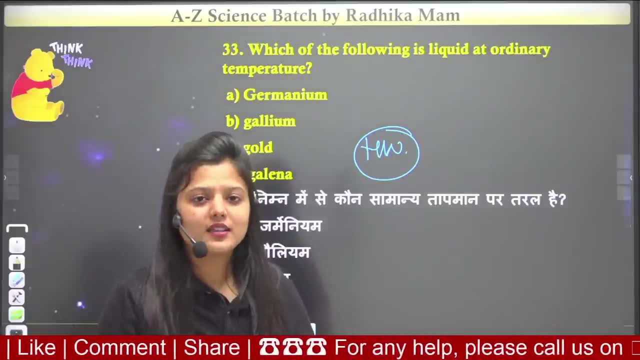 it becomes an easy house. but we don't have to build a house, we have to build a palace. and it takes time to build a house. so don't build a house. build a palace If it takes time. it's a good thing when something is made by taking time. 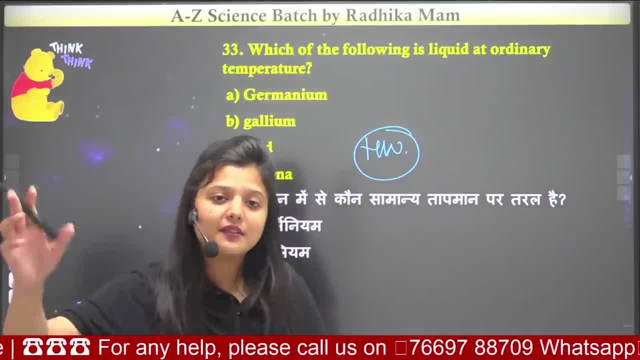 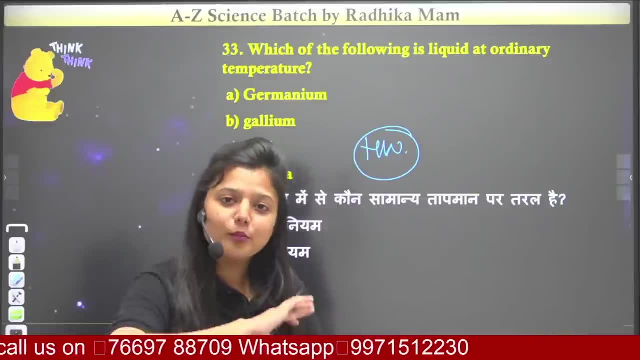 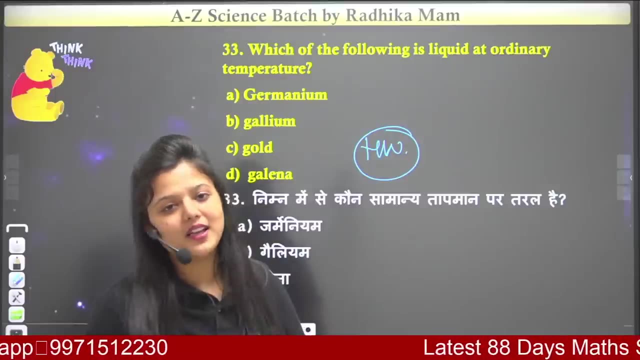 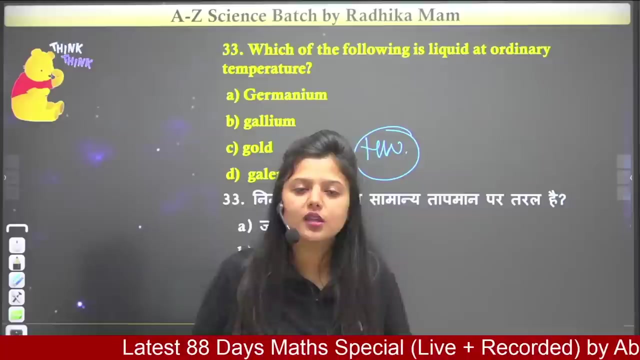 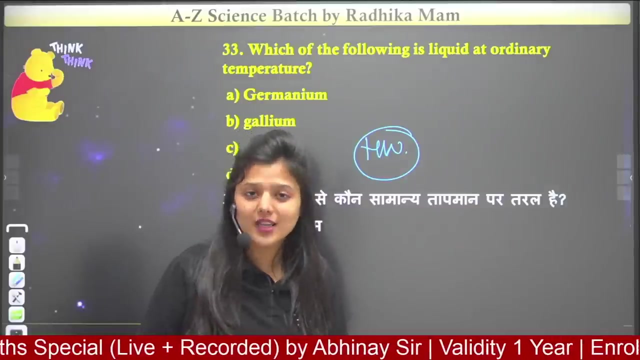 When something is made by hard work, then that thing benefits you. That palace will not become a house. So now it is upon you to build a house. If you want to do a short crash course or a complete science course, you do not have to make your house your palace, so it all depends upon you. the rest of the brother will be your regular classes. tomorrow we will discuss the difference between polymers and soap and detergents. we will discuss on all of them. what is the difference in the life of chemistry, which is dying every day? what are the tests, what medicines are used and how do you show your different problems? we will discuss on all of them tomorrow evening at 6 o'clock. and with this there is some important news that you have to give me here: that if you are also doing preparation, then 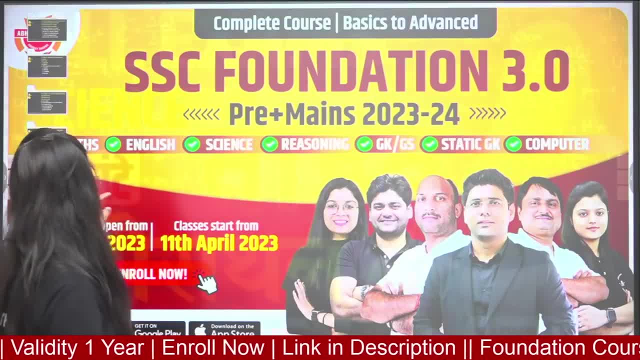 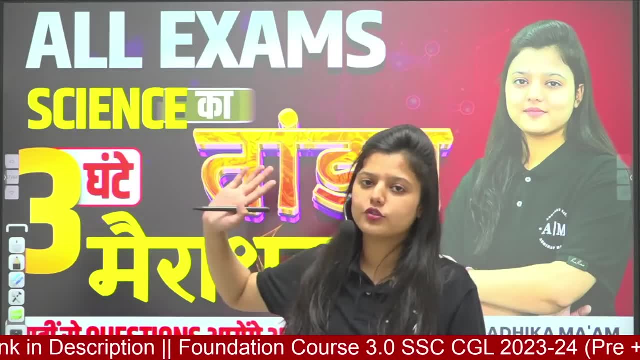 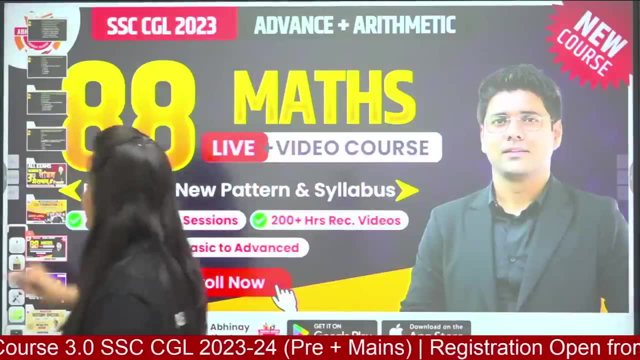 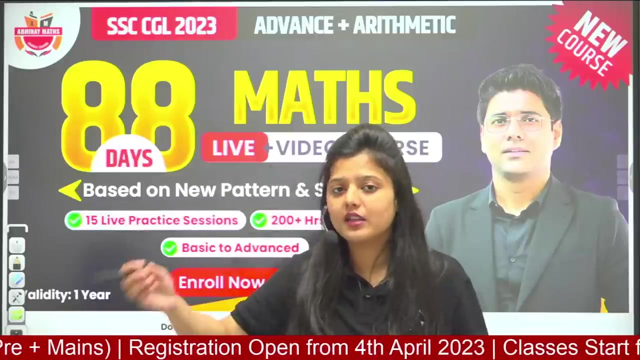 important thing. first of all, your 3-hour marathon is on Saturday evening at 6 o'clock. you will meet with all the best to best questions of science, physics, chemistry, biology- not alone with physics, chemistry and bio. plus, see, whatever pain you have in math. get rid of that pain, because your 88 days course has come and Abhinay sir has already recommended so many toppers, students who have already recommended themselves, those who have benefited. now you can also become one of them, and